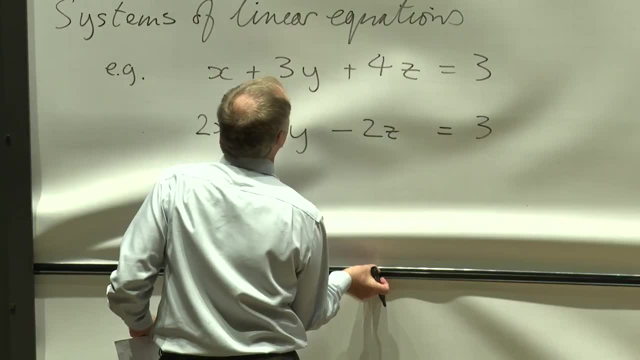 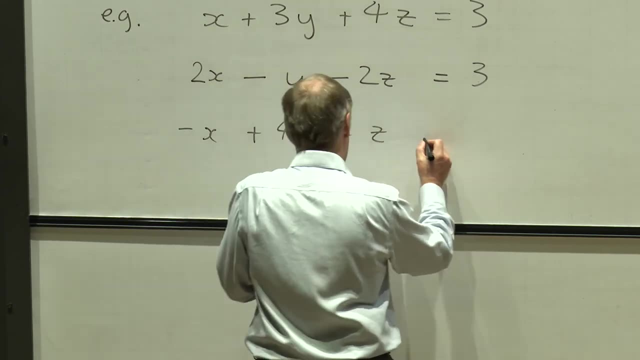 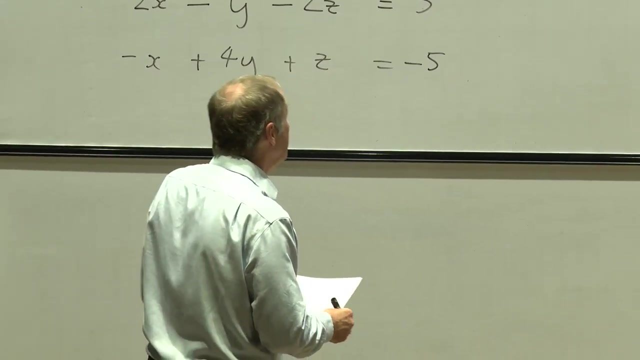 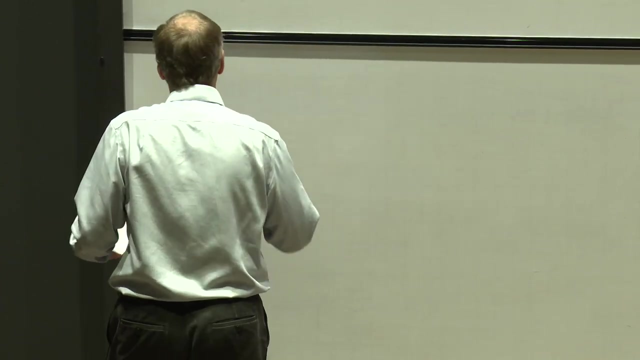 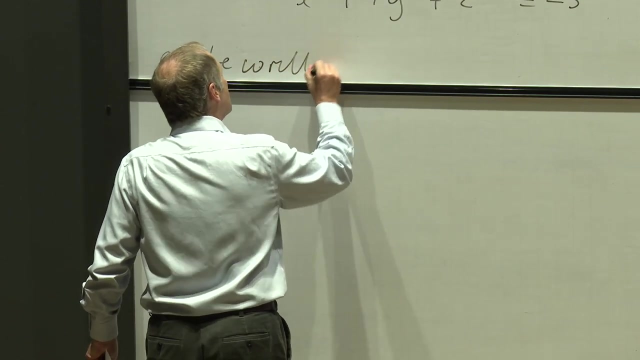 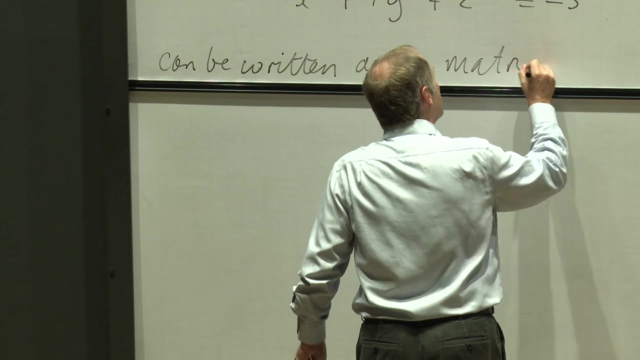 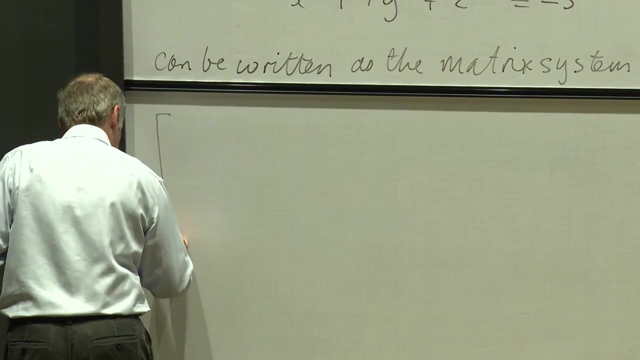 And minus x plus 4y plus z is equal to minus 5.. So here's a system of linear equations that you perhaps recognize. Okay, and this can be written as the matrix system. And the matrix system would be well, we put the coefficients in this matrix. 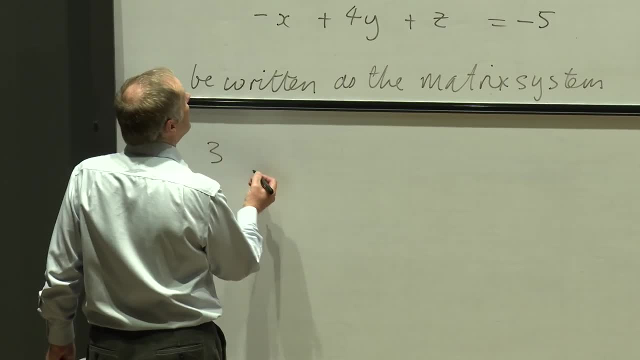 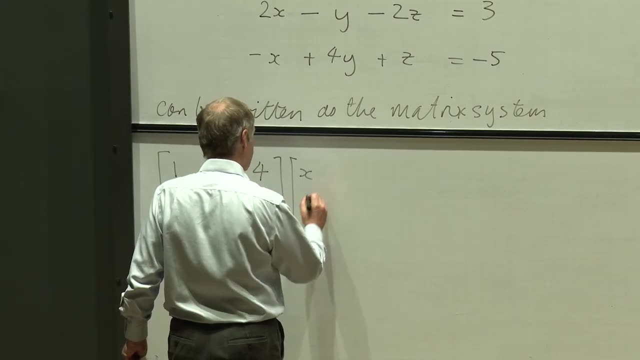 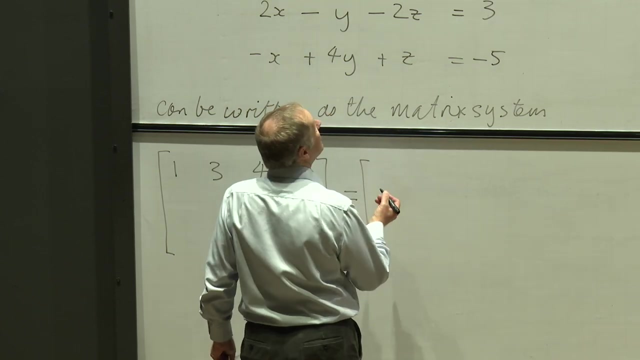 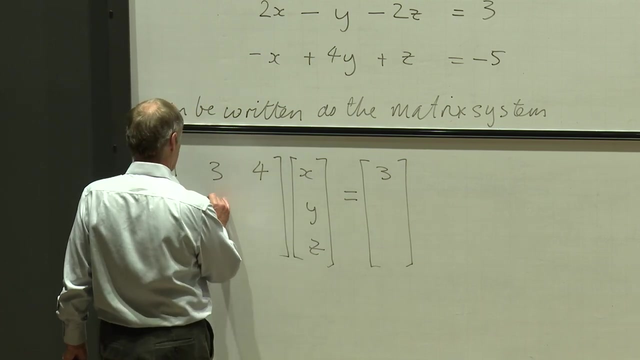 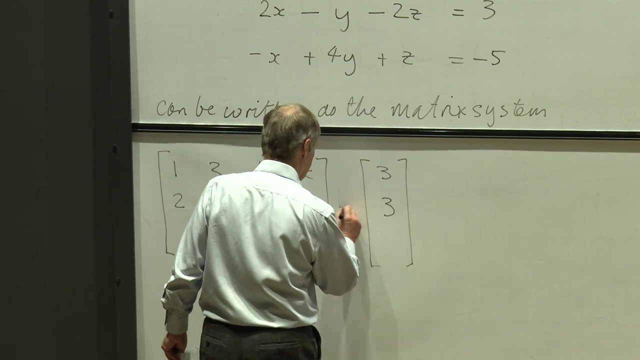 So we have 1,, 3,, 4.. Okay, it's our initial variable. So here's the function, right? The function of the matrix, right? So it's the exact same equation as you would use a random variable. Okay, Okay. So so we've got x, y, z, and that's equal to the first. one is 3.. Okay, And then the next equation is 2, minus 1, minus 2, is equal to 3.. 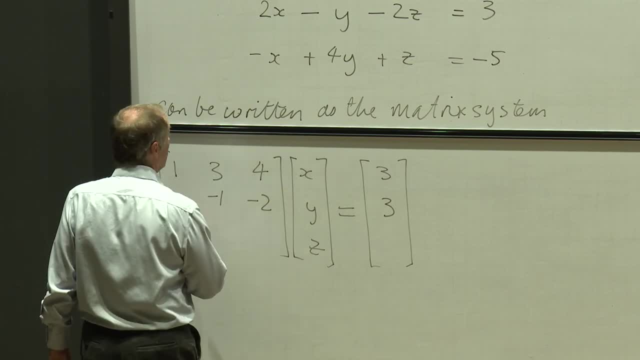 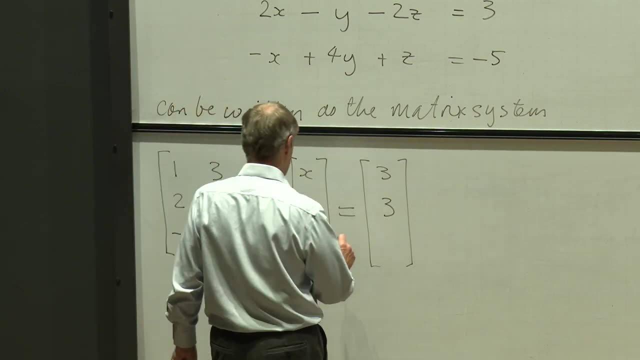 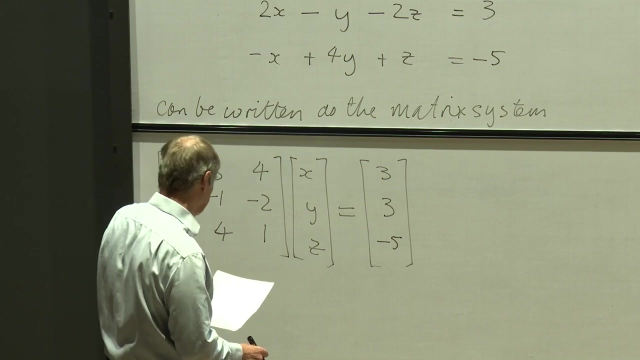 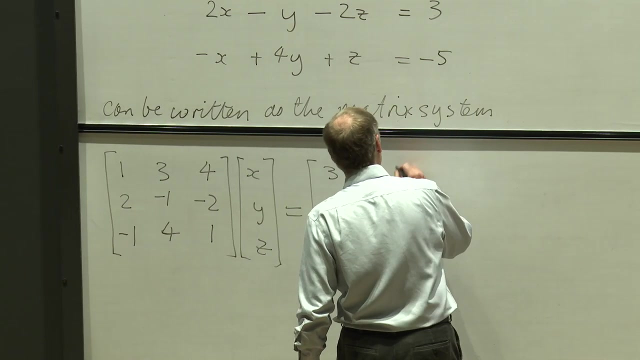 Okay, Okay, Okay, Okay, Okay, Okay, Okay. And then the last equation is minus 1,, 4, and 1,, and this is equal to minus 5.. Okay, Or we can write it as a so-called augmented system. 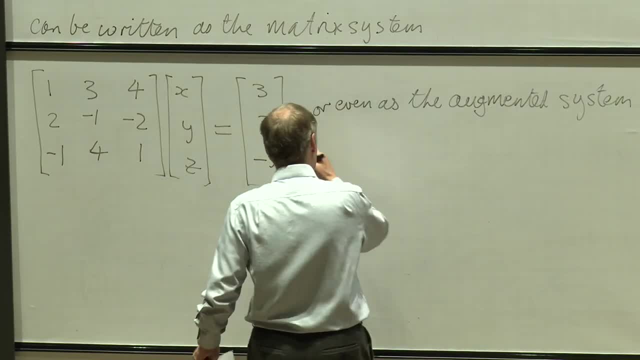 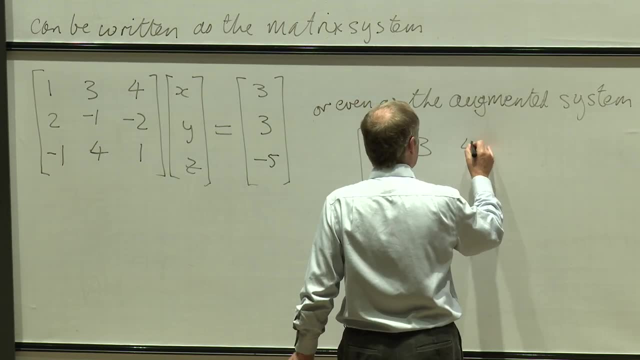 And the augmented system would be: I'm sorry I haven't lined this up, But essentially this is the same. So I'm going to take the numbers from the matrix and I'm going to augment And I'll just put a little dashed line in here. 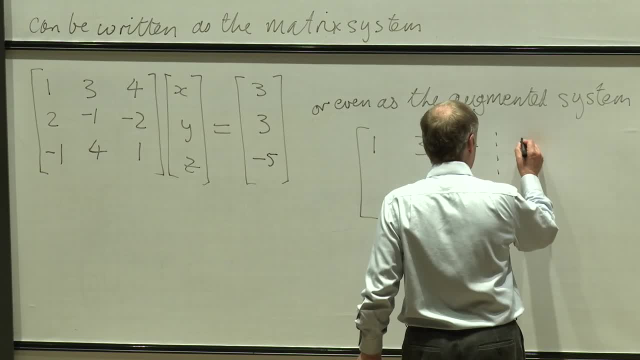 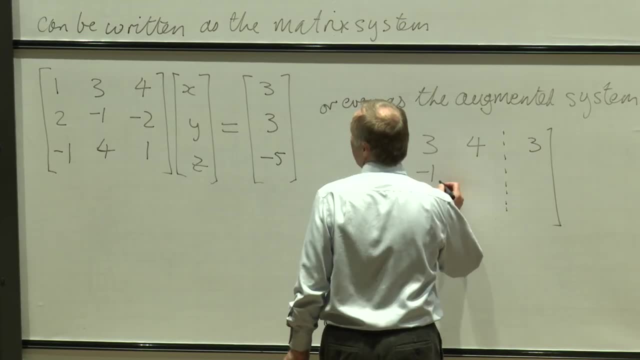 That's of no consequence, It's just to help you read this. And we put the 3 at the side here, So in some sense we've lost the x and the y and the z. Please tell me if I make a mistake, right. 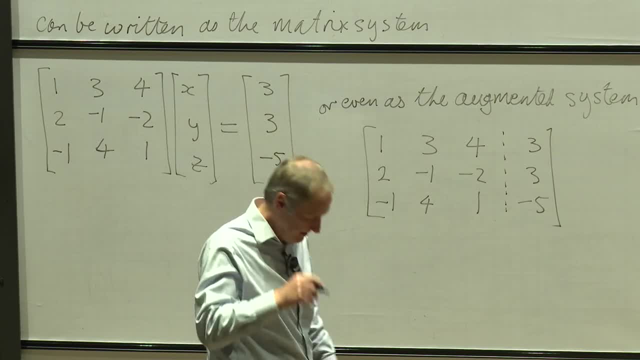 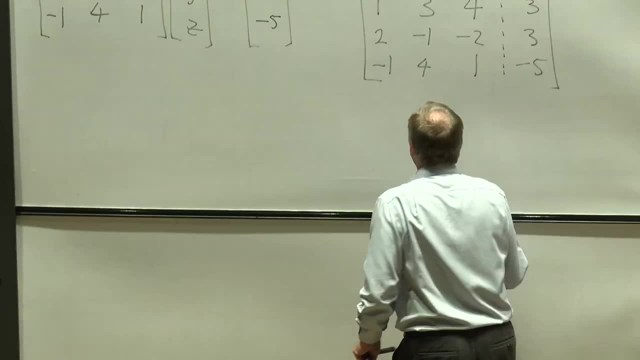 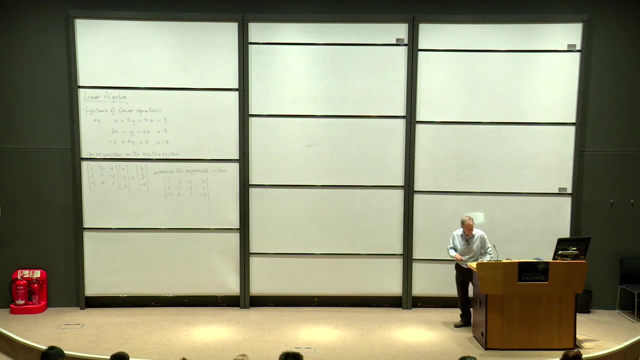 So, as I can see, that's the same augmented system. Okay, so if we have such a system of equations, then we can manipulate them in certain ways. So tell me if this pen is too thin, because I can't find a thicker one. 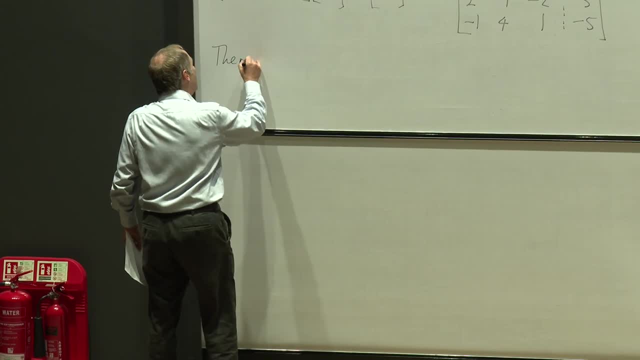 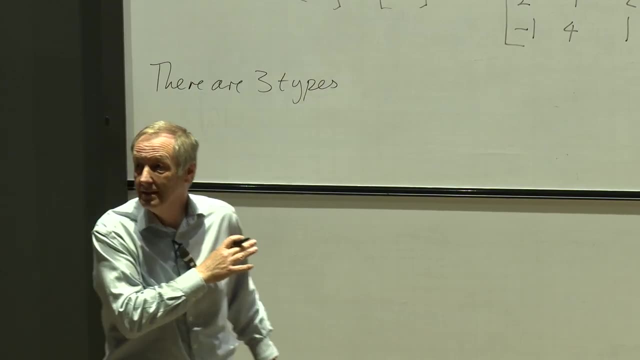 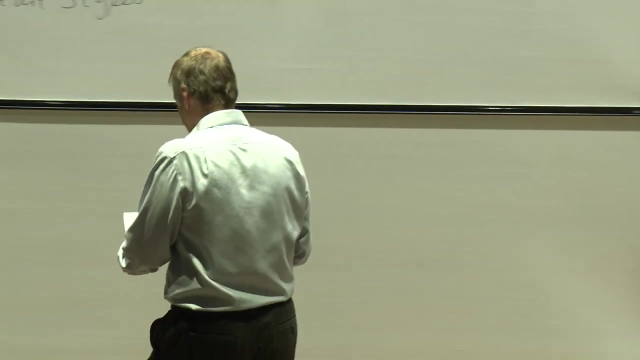 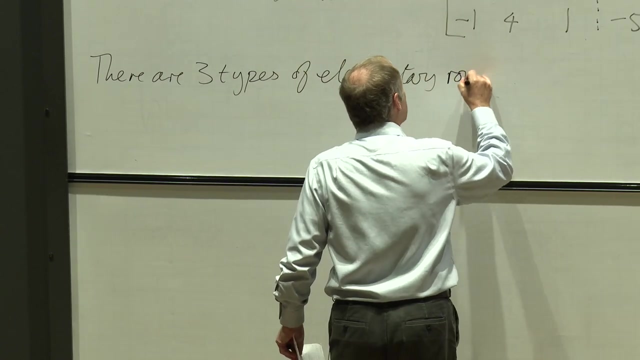 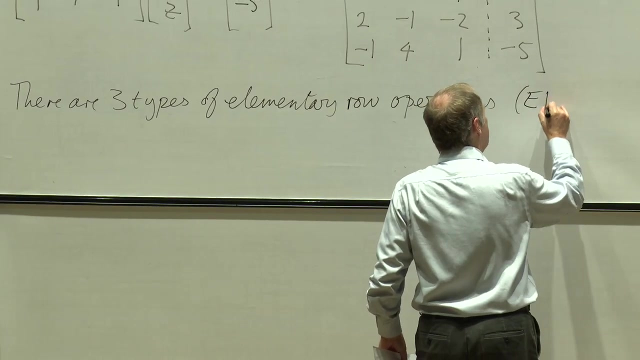 So there are three types. Can you read that? Can we read that? I'm asking the people in the back row really, Okay, Okay, there are three types of elementary row operations. So, people, I'm not going to write this all the time, so I'm going to call this an ERO. 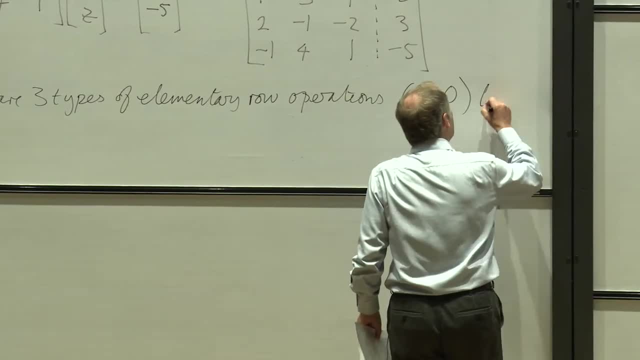 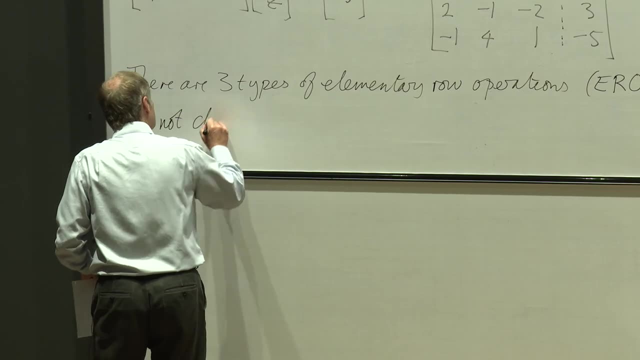 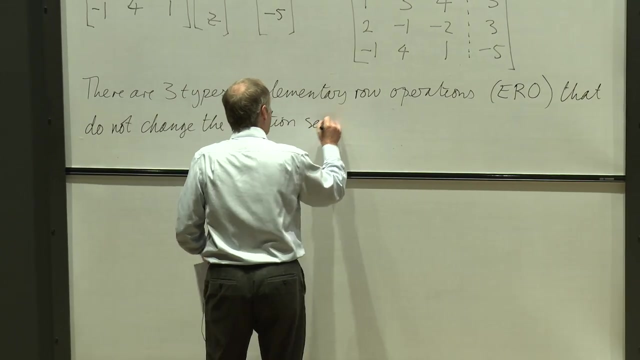 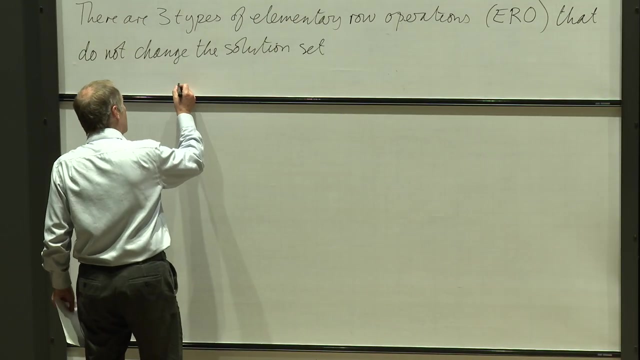 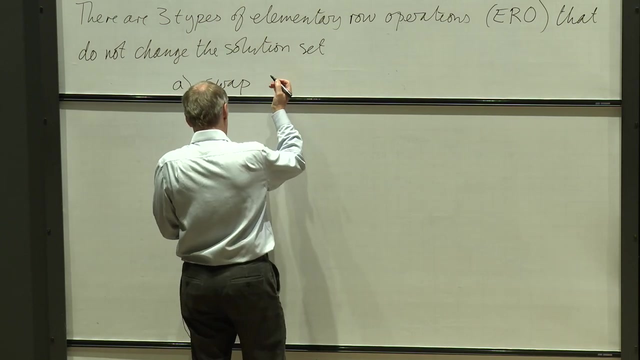 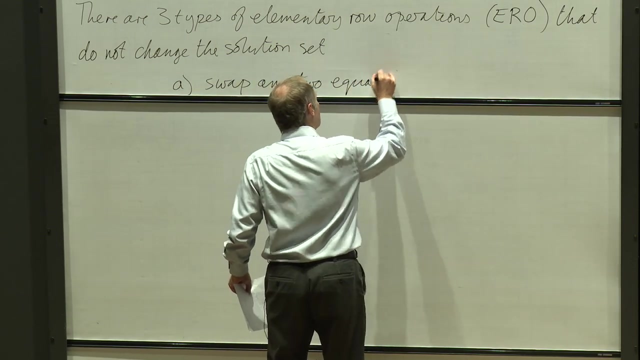 An elementary row operation: Okay, And they that do not change the solution set, Okay. So the first elementary row operation I'll call A is to swap any two equations. So the first elementary row operation I'll call A is to swap any two equations. 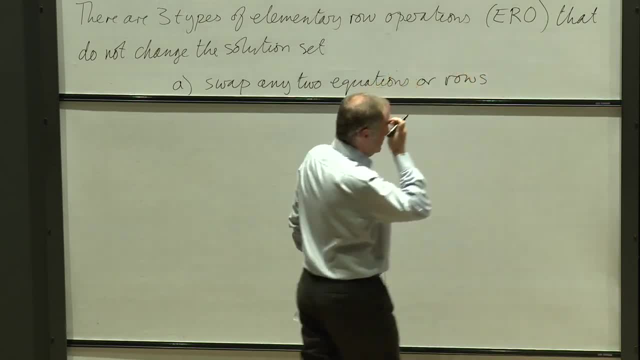 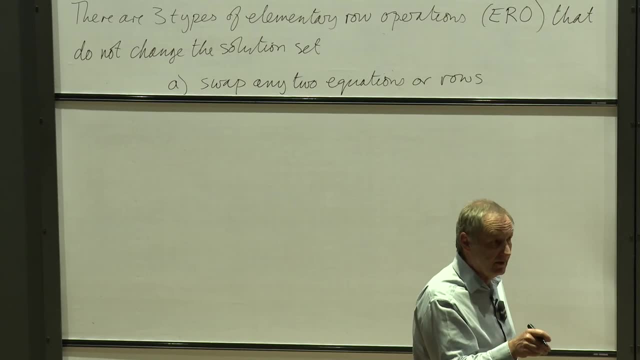 And the equations correspond, of course, to rows, as you see in this matrix, So I can swap them. In other words, those equations I was given at the top, I could have been given the second one first, The first one first. 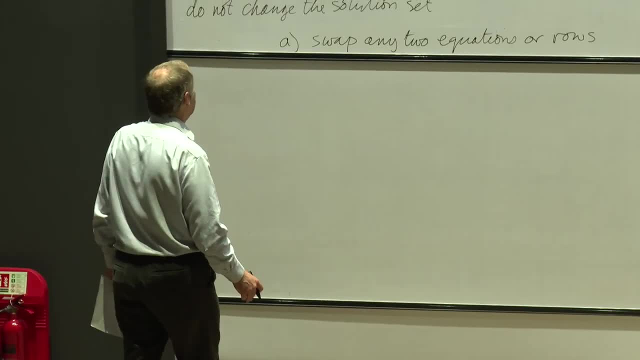 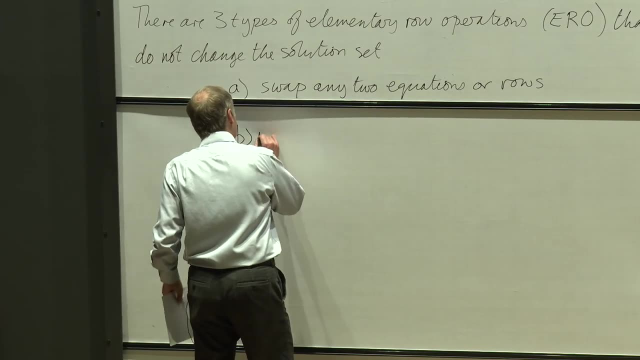 So no change in the solution set, if I simply take them in a different order. Yeah, I liked that. Okay, it's served. You're right, It's that simple and it fits in. So let's do it for one more time, but I think it's all a little bit tricky. 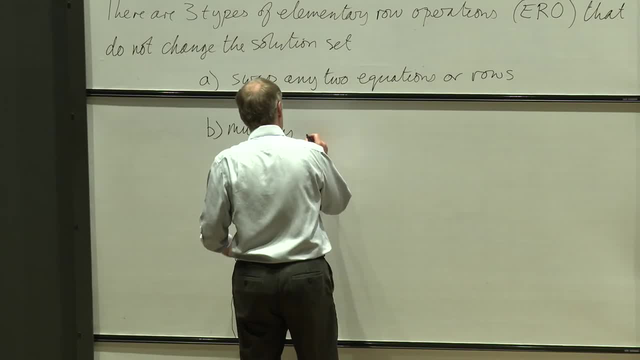 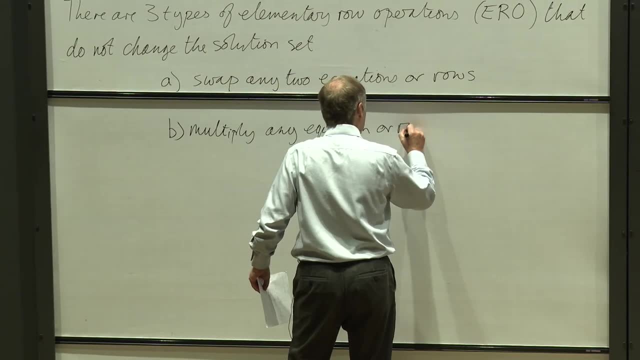 But one of them looks a little bit complex And actually it's very nicely made and little bit fast. It looks more like a Clouder application, but it's got desery thinning stuff. Yeah, This one is on an 11th channel. 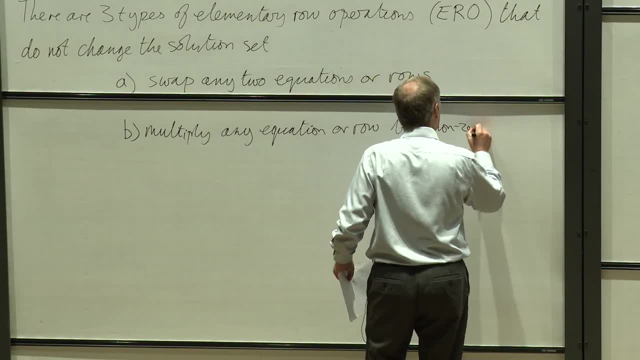 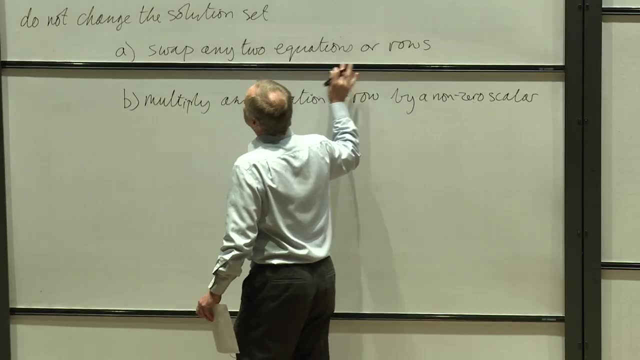 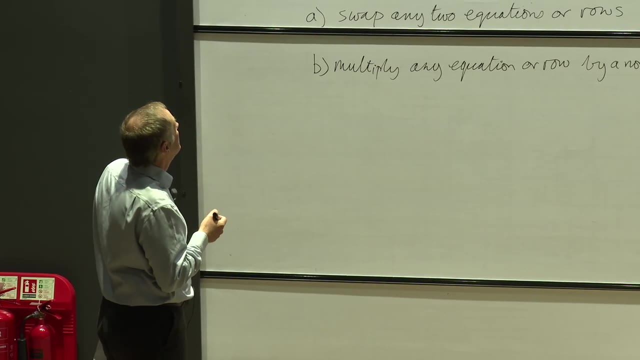 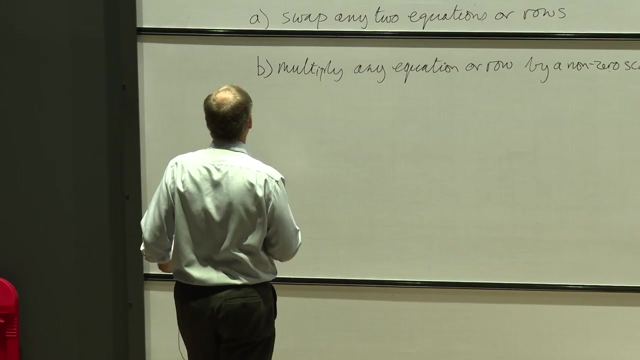 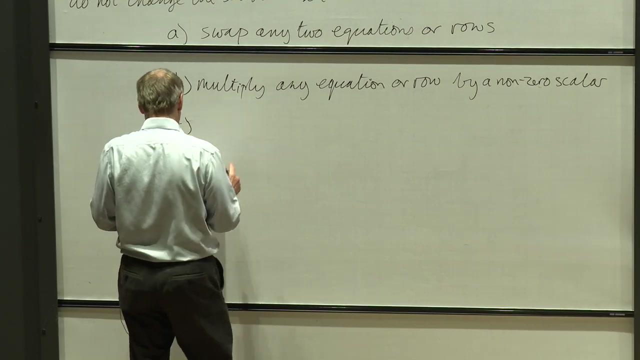 Yeah Well, we'veamo Representative Web, Isn't It the Only E霨 See scalar. so if my second equation there was 4x minus 2y minus 4z equals 6, it would carry essentially the same information: C okay, and C is add a. 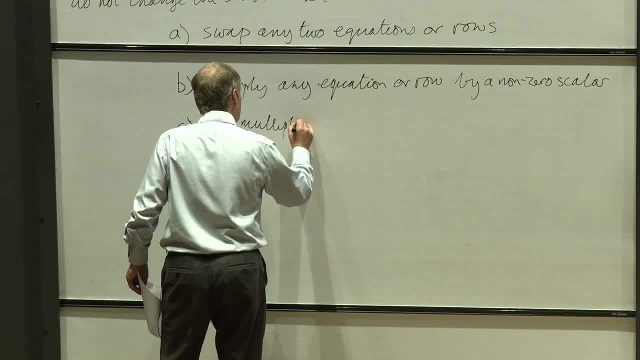 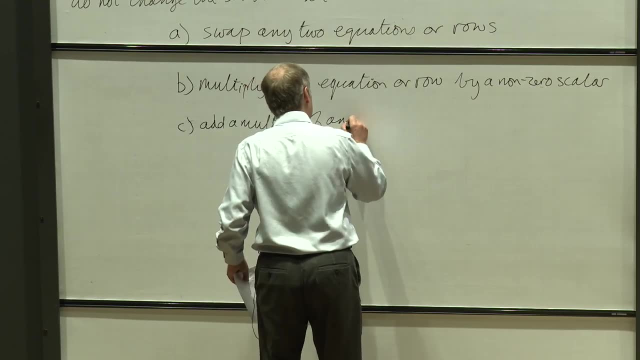 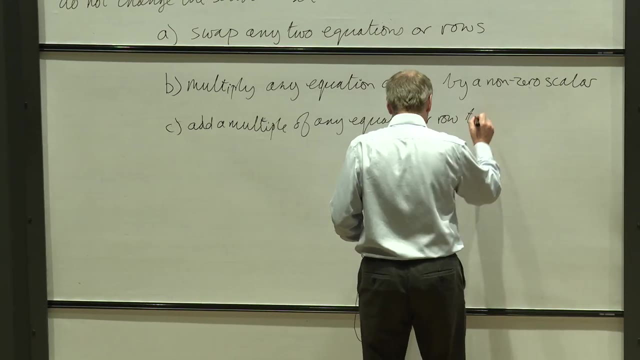 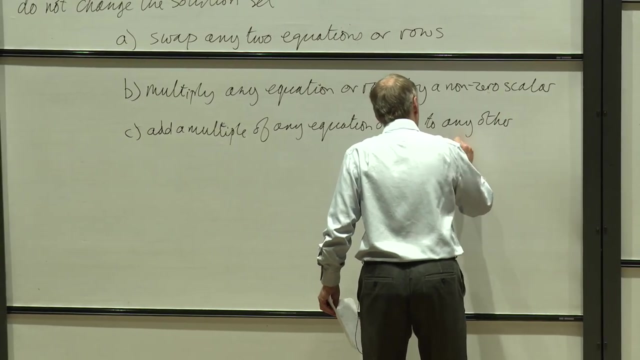 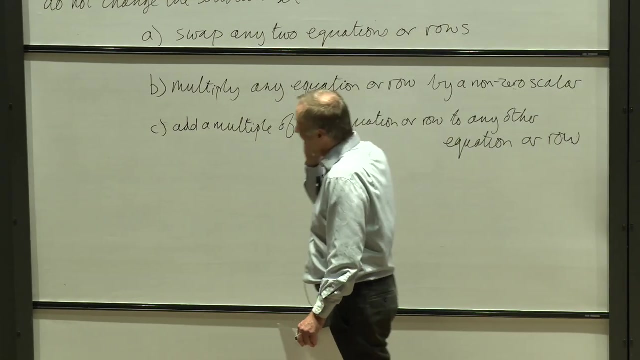 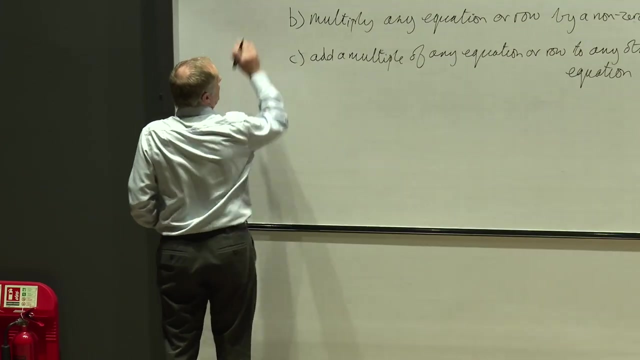 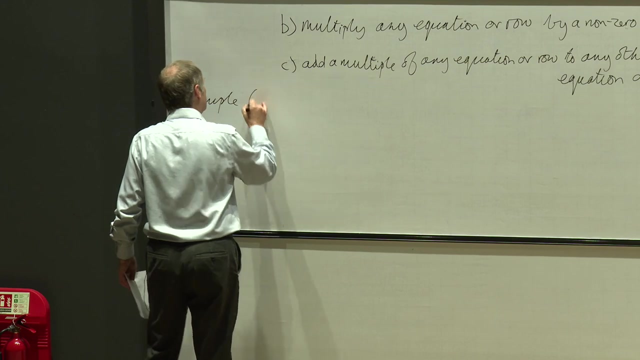 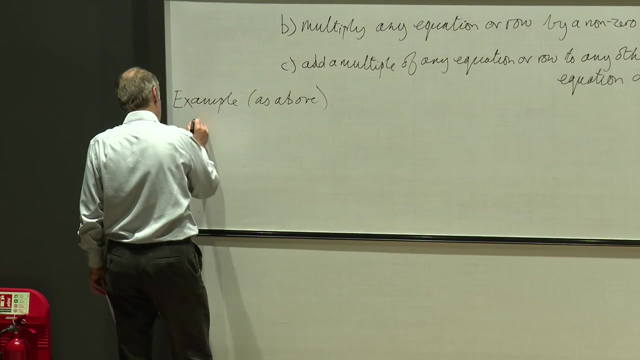 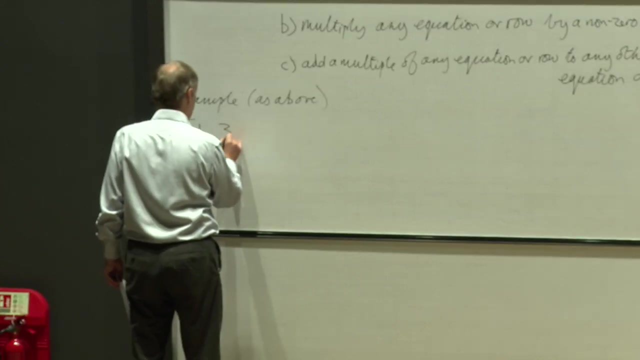 multiple, multiple, yeah, okay, of any equation or row to another equation or row any other. so these are our three elementary row operations. so let me do an example as above. so this is exactly those equations there. okay, so I start off with the augmented matrix: 1, 3, 4, and then there's this little partition, and I'd meant it. 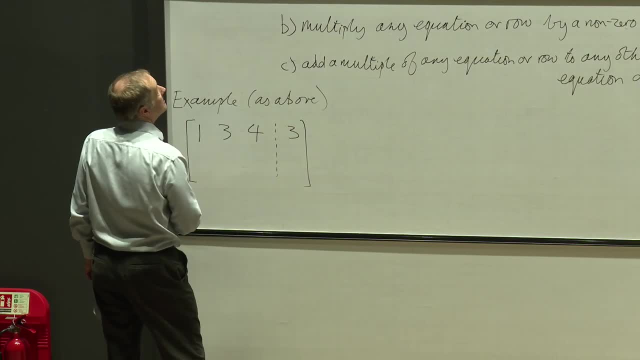 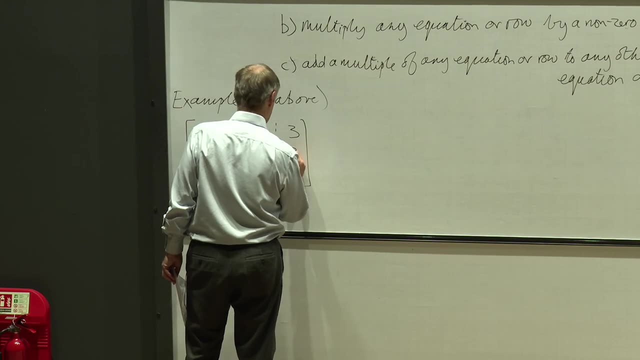 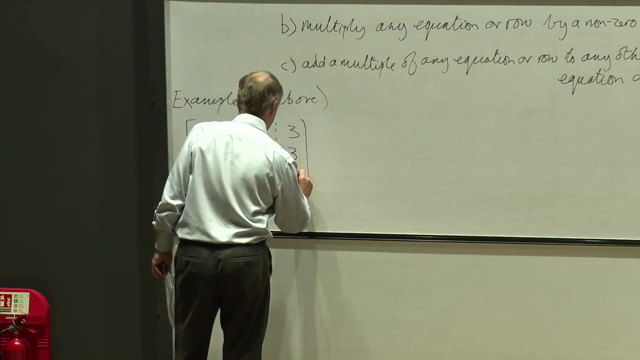 by 3, and then the second equation is 2 and minus 1 and minus 2, and that's gives us 3, 3, and the final equation is minus 1, and 4, and 1,, and that gives us minus 5.. 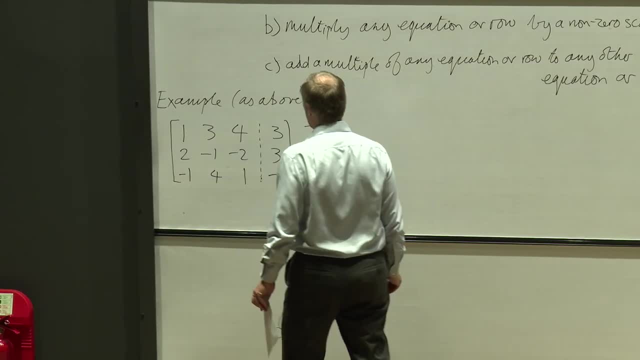 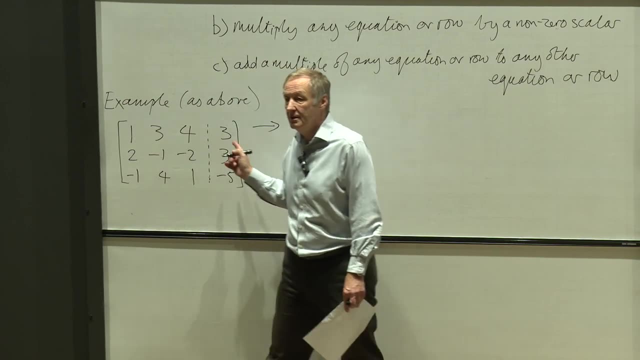 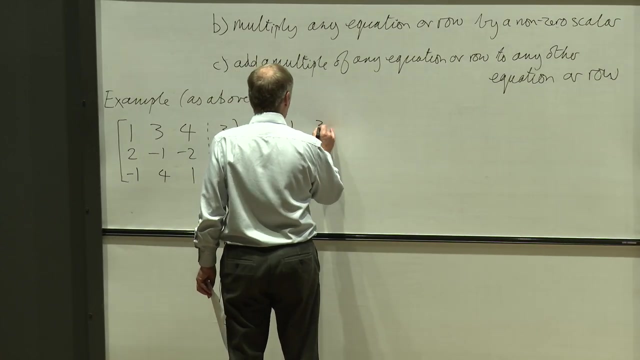 So now I'm going to apply elementary row operations. So the first thing I'm going to do is I'm going to subtract twice the first equation from the second equation. So I'm going to leave the first equation alone, so this will be the same. 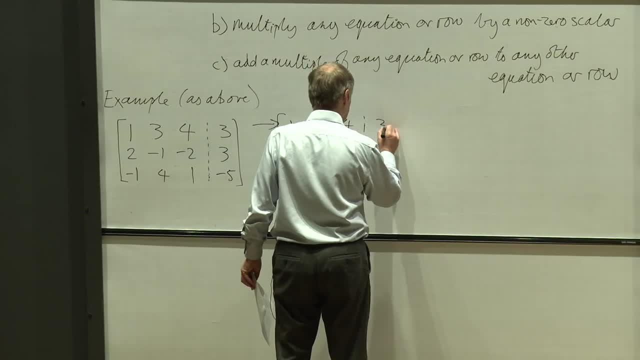 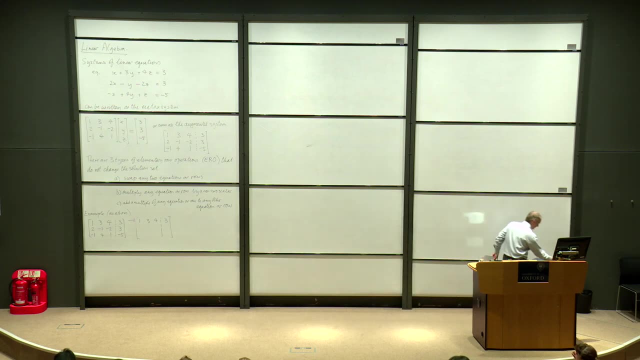 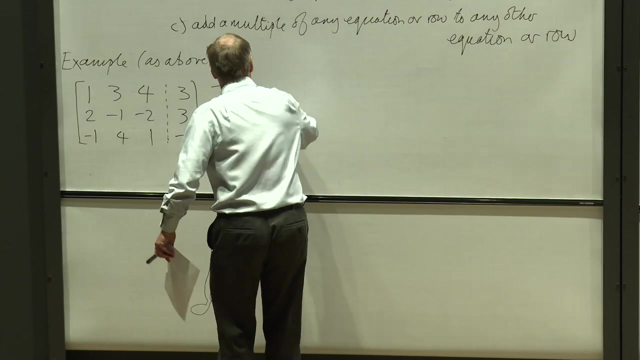 1,, 3,, 4,, partition 3.. But I'm going to- oh, I need to leave myself space to tell you what I'm doing, so I'll leave some space. I'm going to leave some space for what I'm doing. 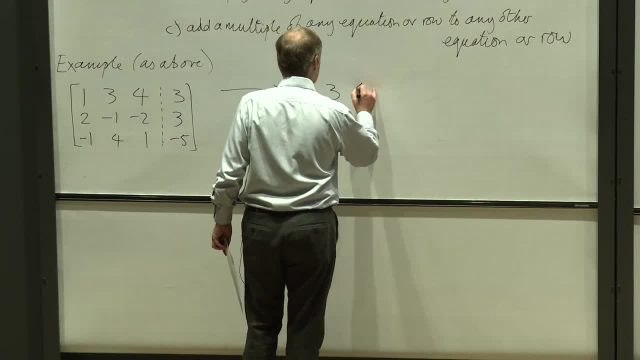 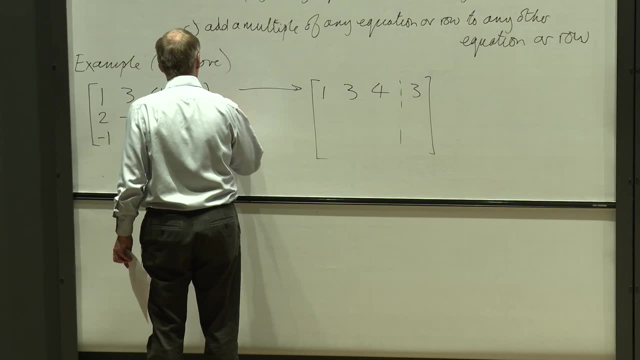 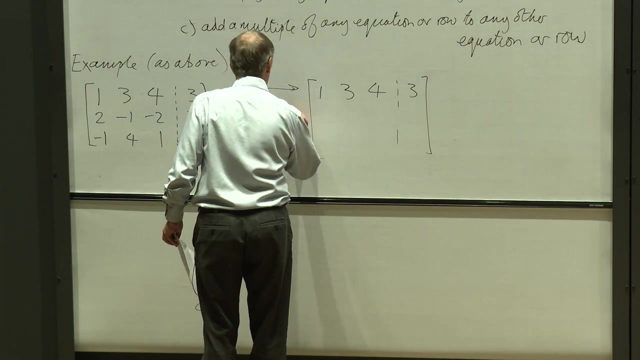 So here we go, So 1,, 3,, 4, the partition and the 3.. And then I'm going to do: row 2 becomes row 2, OK, plus minus 2.. I'm going to move this again because there's still not. 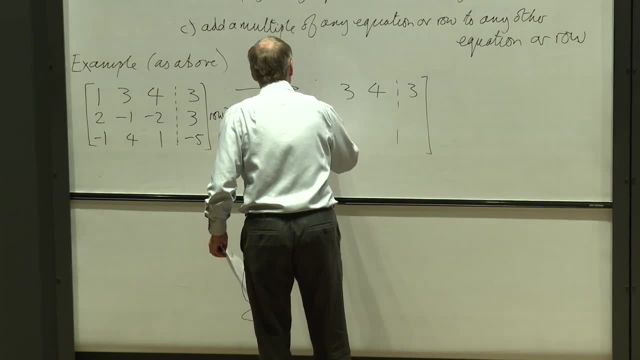 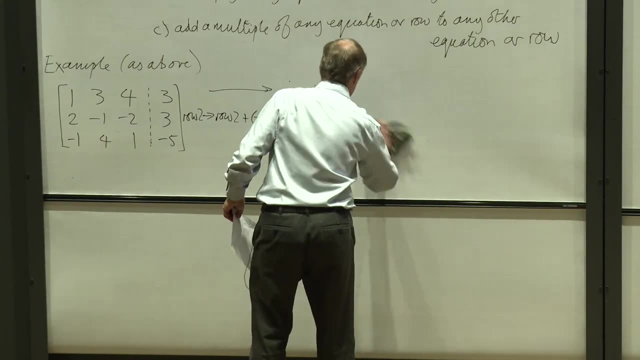 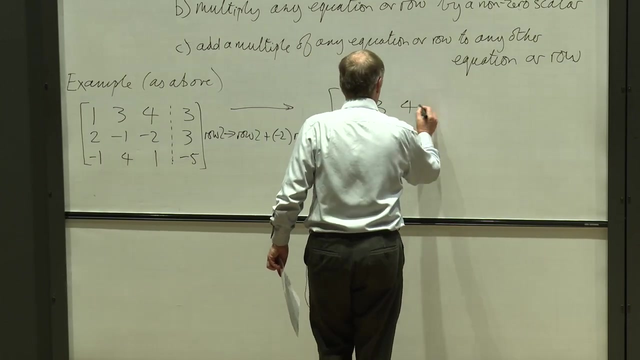 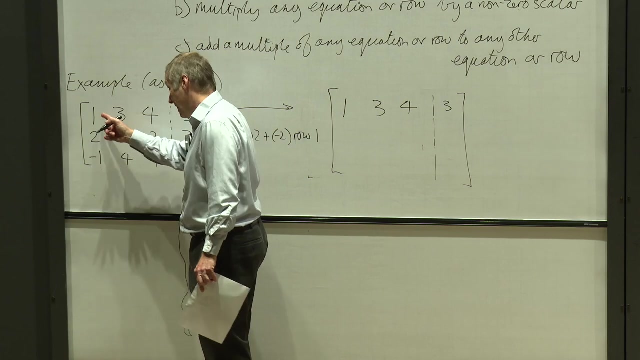 enough room times: row 1.. So the first row stays the same. So I'm going to add to the first row minus 2 times the first row. And now, if I add subtract, I add minus 2 times the first row. 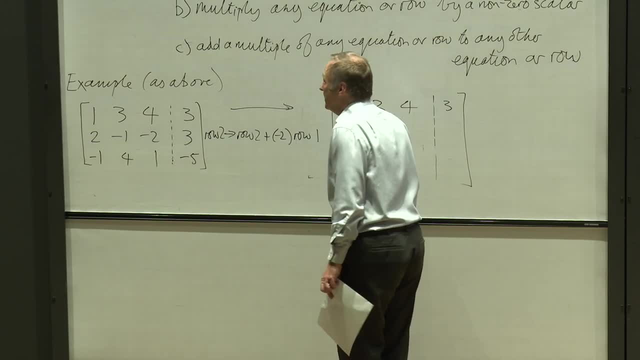 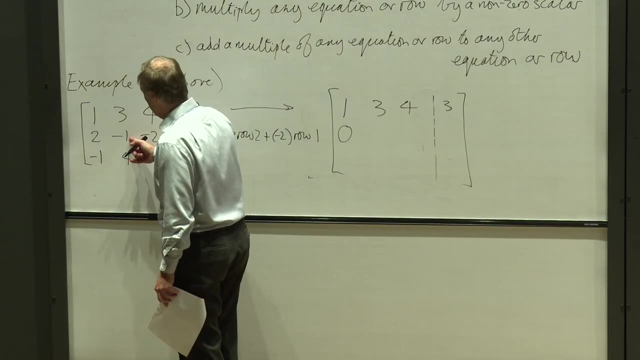 to the second row. I'm going to create a 0. there aren't I? 2 plus minus 2 times 1 is 0.. And then I've got to take minus 1 and add minus 2 times 3 to it. that's minus 6.. 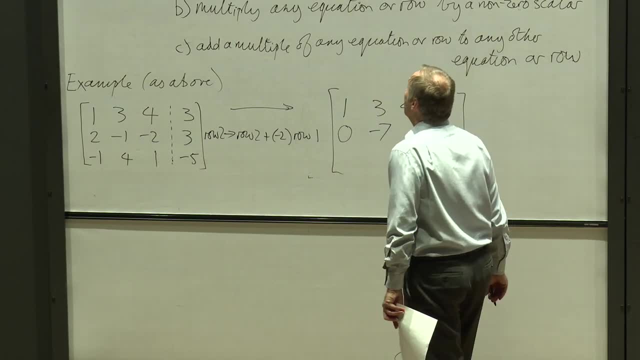 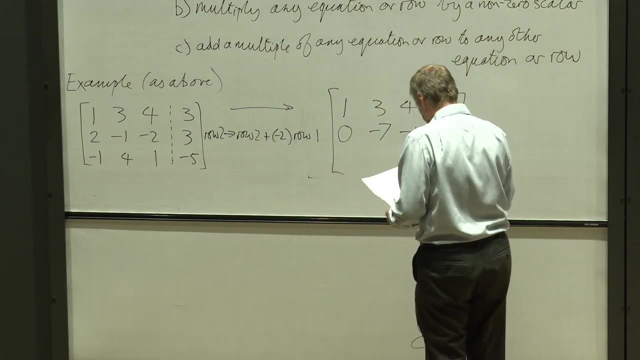 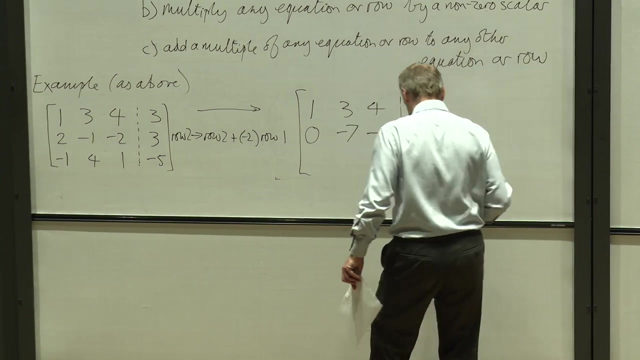 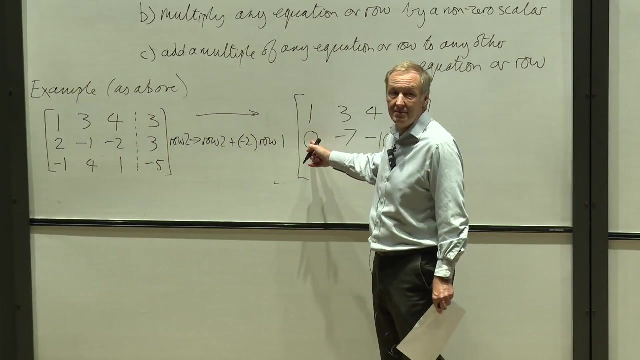 That gives me minus 7, as far as I can see. Minus 2 minus 2. lots of this gives me minus 10, I think. And then 3 minus 2- lots of 3 is minus 3.. OK, So all that I've done is somehow make this simple. 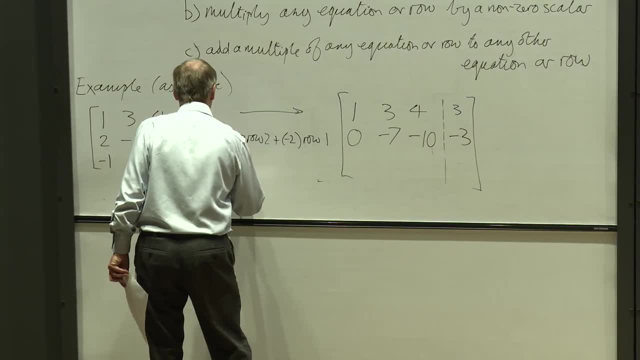 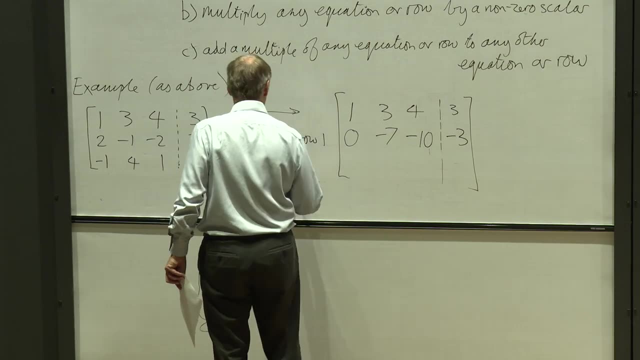 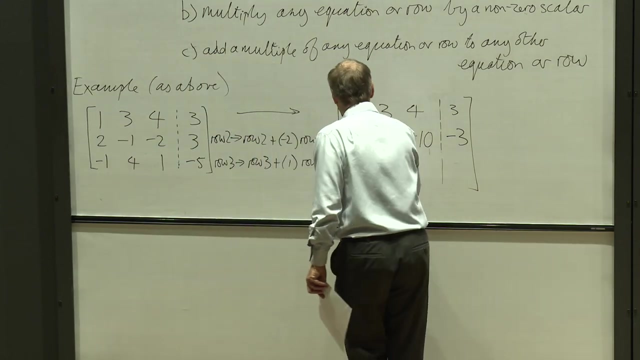 And then I'm going to do the same sort of thing in the final row. So row 3 is going to be row 3, plus what? Plus 1 times row 1.. OK, Because then if I add minus 1 to 1, I get 0.. 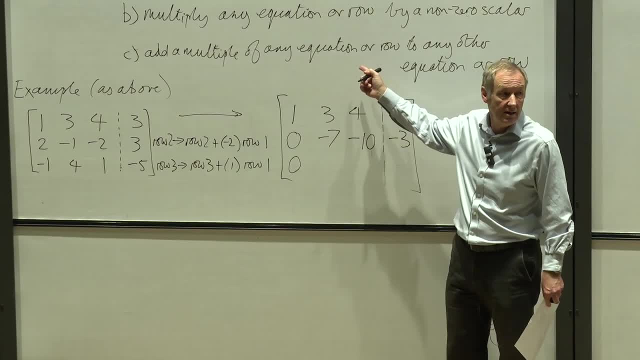 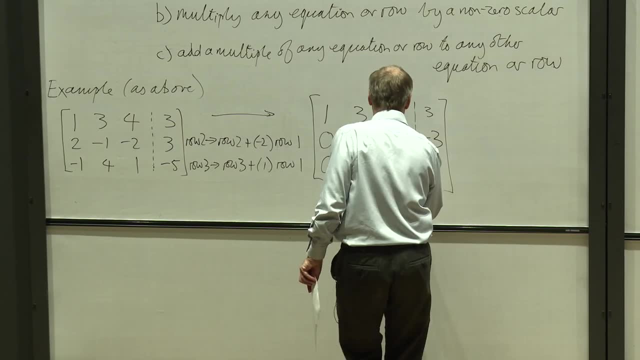 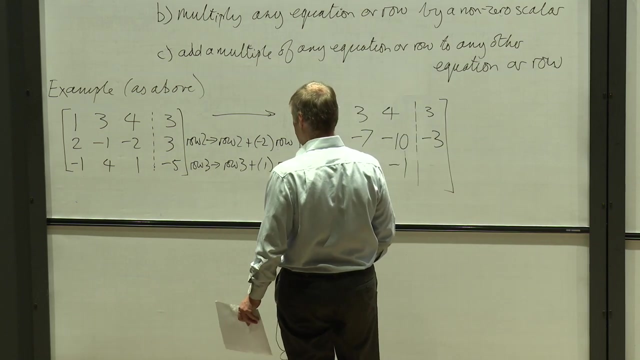 So this is just this elementary row, operation C. That's all this is. And so 4 plus minus 1 is 3. And 1 plus minus 2 is minus 1, as far as I can see What, Oh, I'm adding the wrong row. 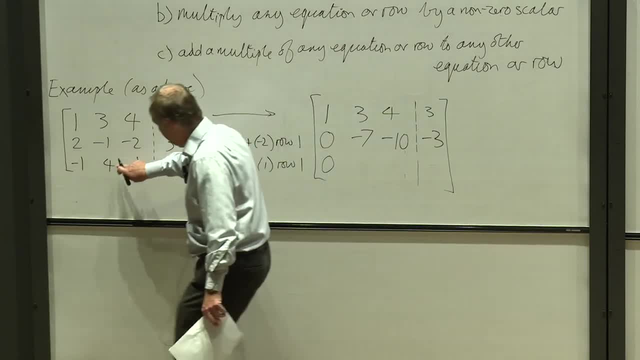 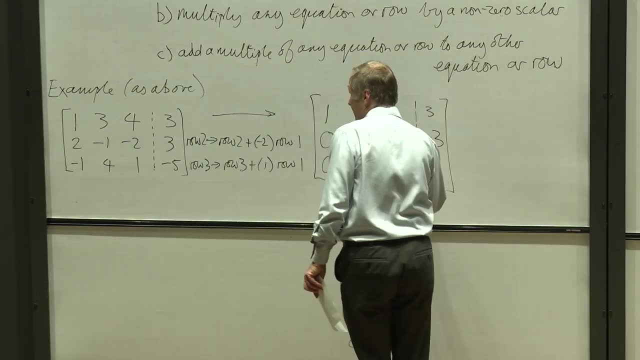 I'm adding the wrong row. Look at that. OK, I've got to add 4 to 3 to give me 7, because I'm adding row 1 here And 1 to 4 to give me 5.. Is that right? 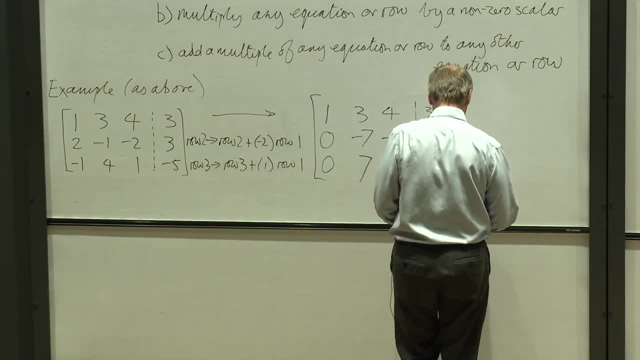 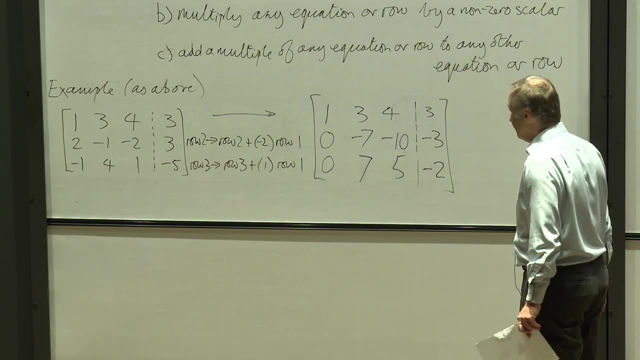 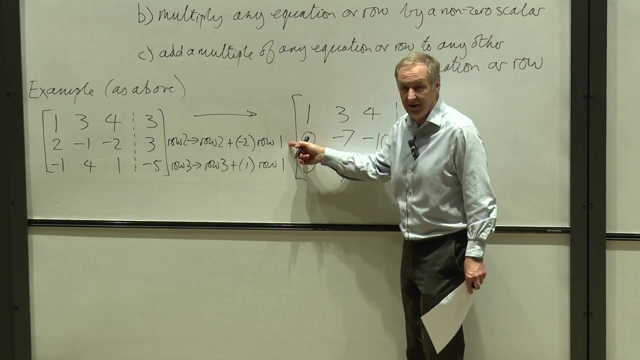 That seems reasonable. OK, And then minus 5. add 3 is minus 2.. OK, So that's just using this elementary. I've done two of them at the same time, because this one doesn't affect row 3, and this one doesn't affect row 2,. 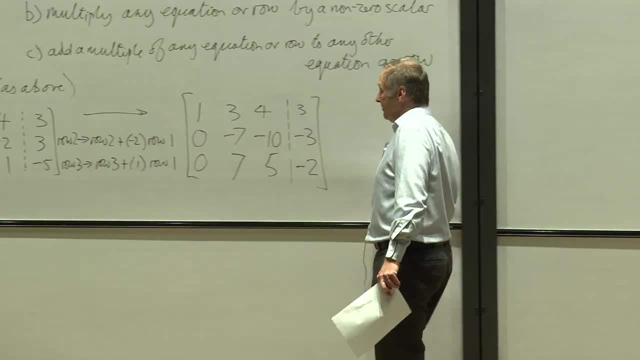 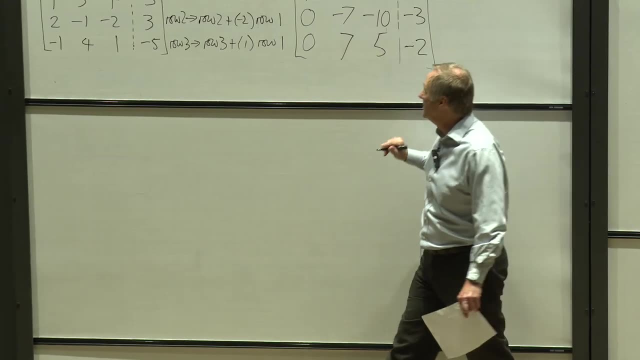 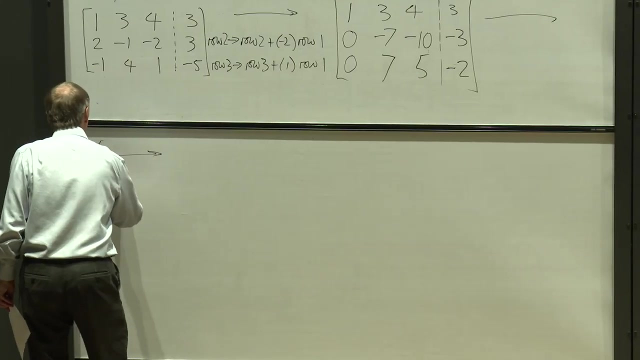 so I can do them at the same time. And then what I'm going to do is I'm going to add row 3 to row 2.. All right, And so this carries on to: if you like, OK, I'm going to do. row 3 becomes. 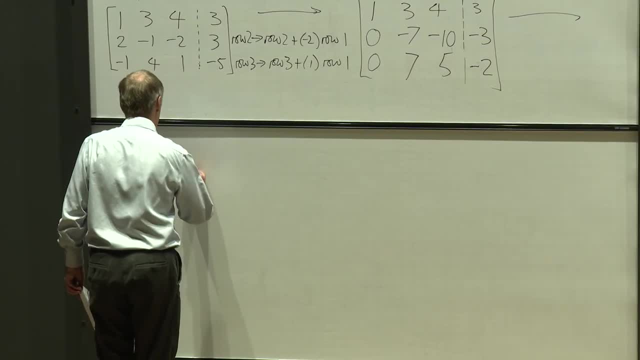 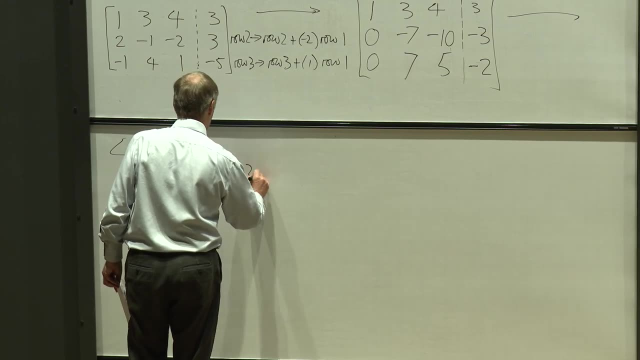 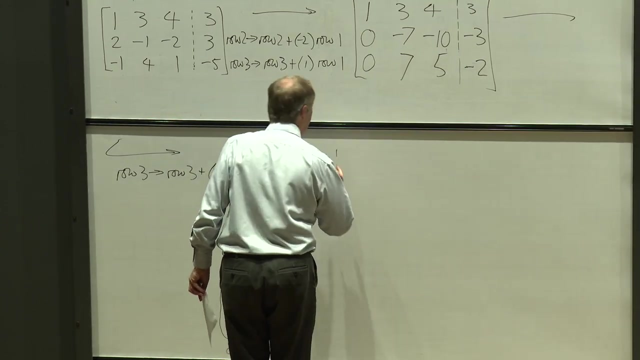 that's what this means: right Row 3.. Plus 1 times row 2.. And what's that going to give me? Well, the first equations are going to be the same, And now the second equation is not going to change. 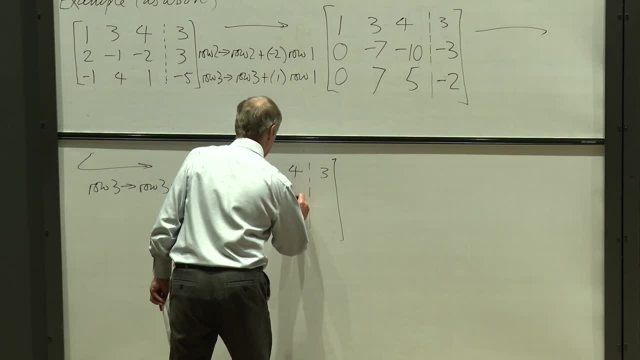 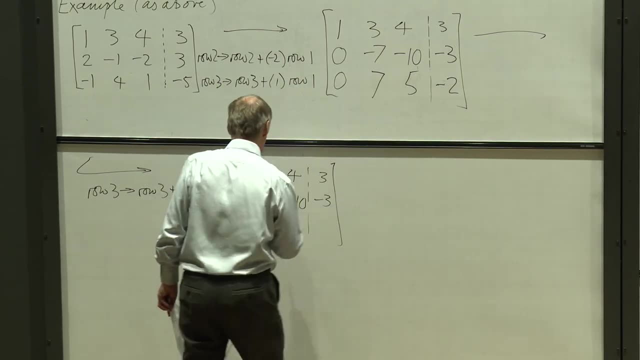 So this is 0, minus 7, minus 10. And I get minus 3.. But now I add this to this to get. well, fortunately, a 0 plus any multiple of 0 is 0. All right. 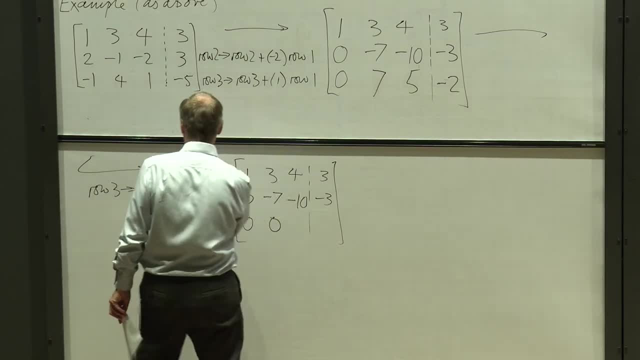 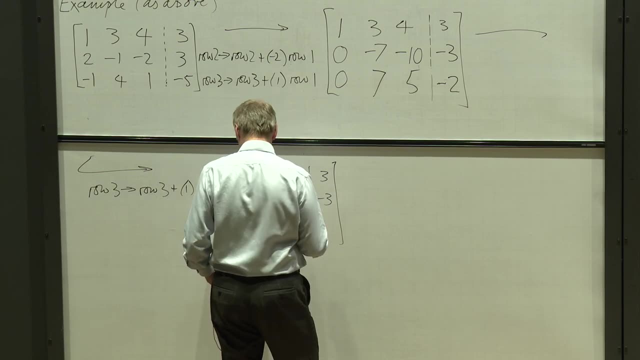 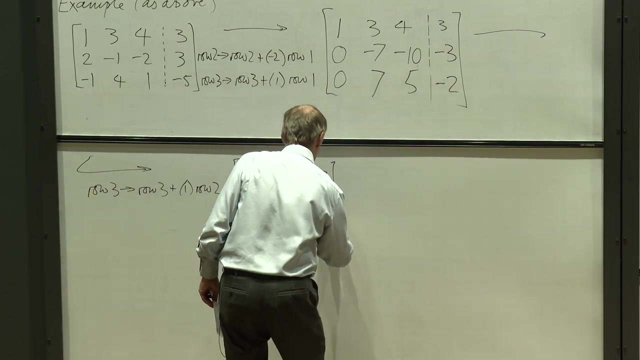 And this gives me a 0 here, by adding row 2 and row 1.. And if I add these two together, I should get this: I should get minus 5.. Add these two together, I should get minus 5.. OK, 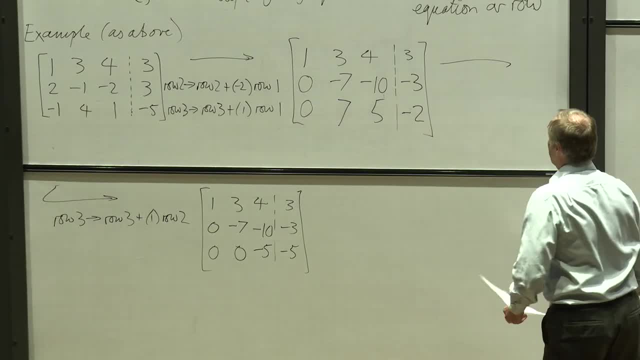 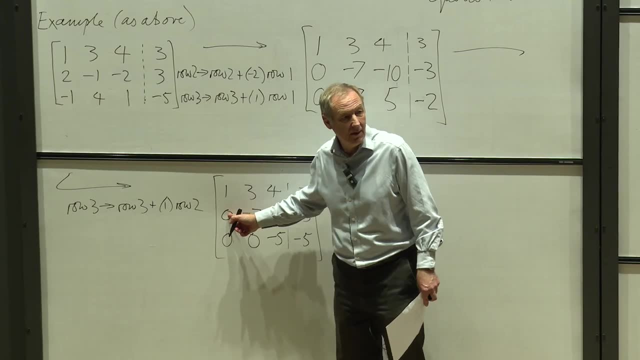 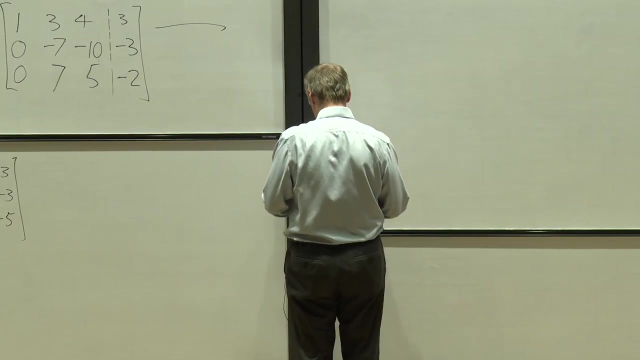 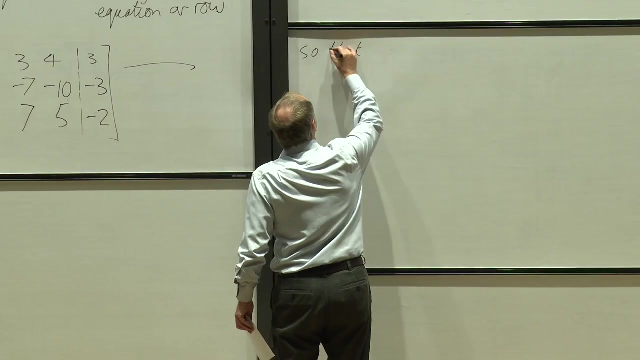 OK, All right. So what have we achieved? We've achieved that x doesn't appear in this equation and x nor y appear in this equation. All right, So what we achieved is that, so that now the matrix, the matrix, the matrix. 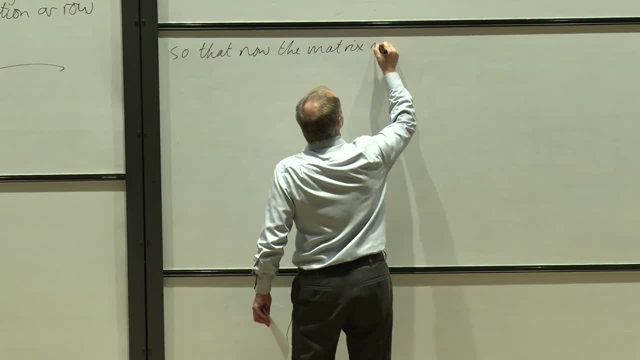 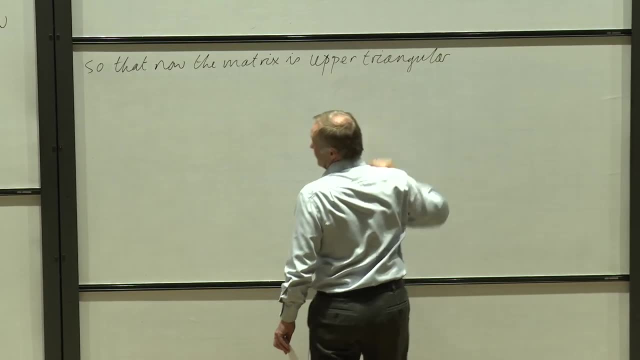 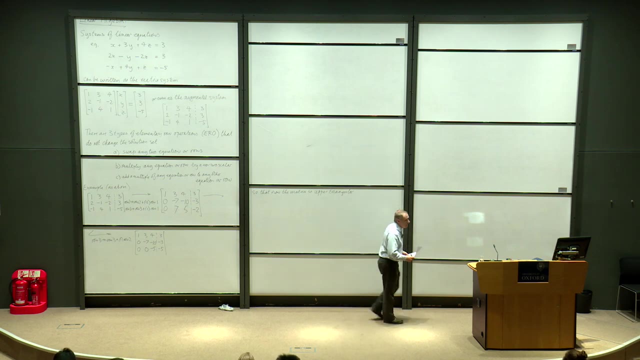 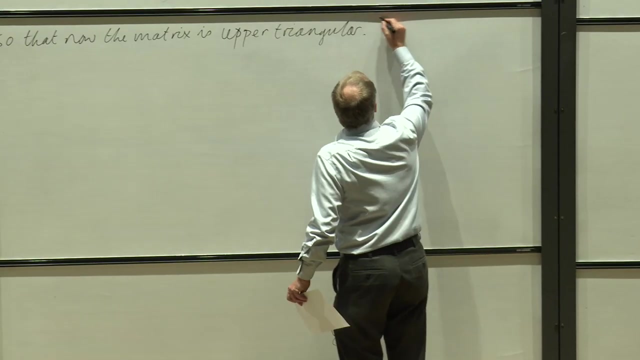 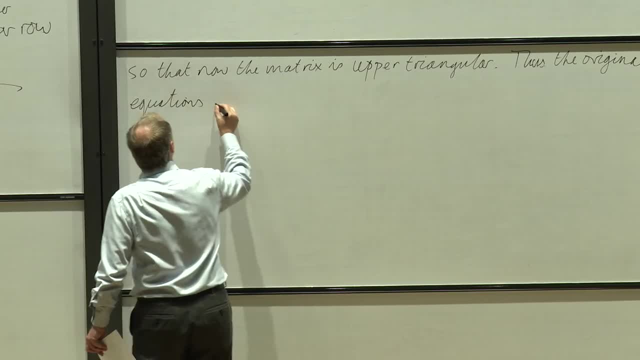 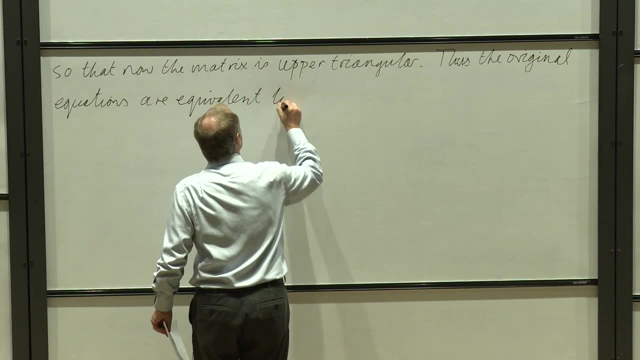 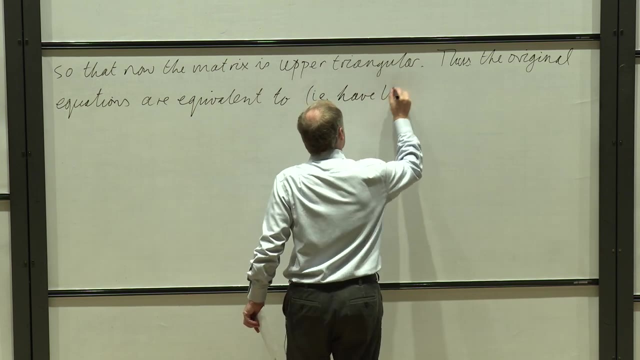 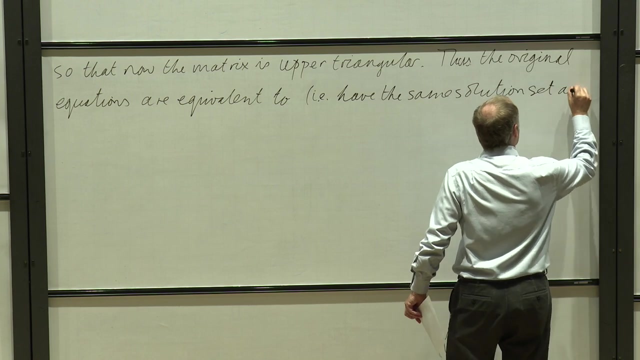 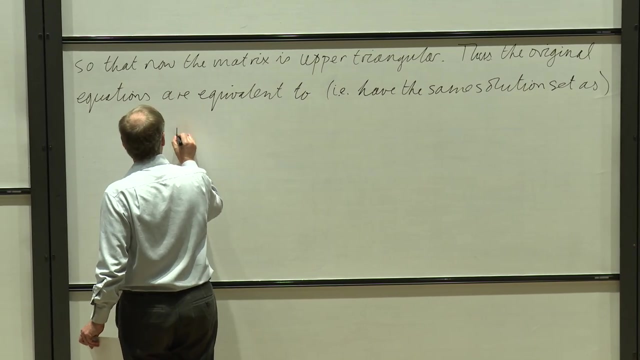 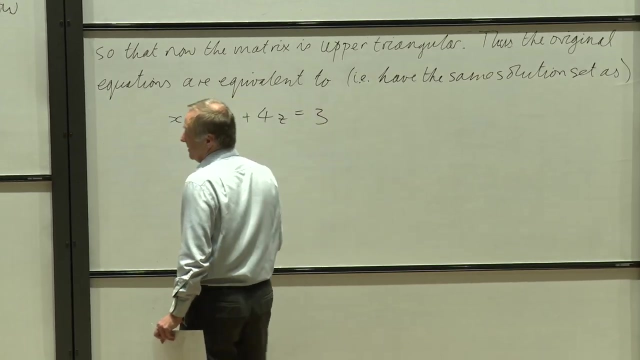 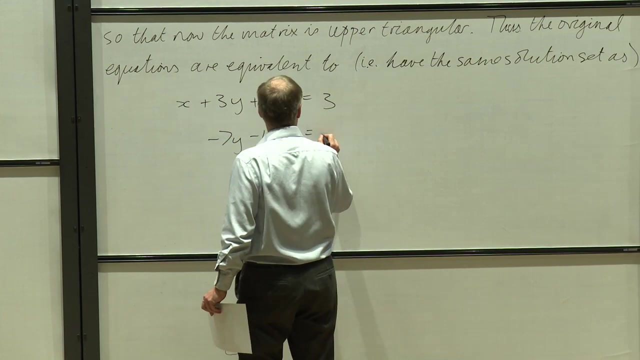 0s. 0s are equivalent to to. in other words, equivalent means. I have the same solution set as. that's what equivalent means here. OK, And these equations are now: x plus 3y plus 4z is equal to 3 minus 7y minus 10z is equal to minus 3 and minus 5z is equal. 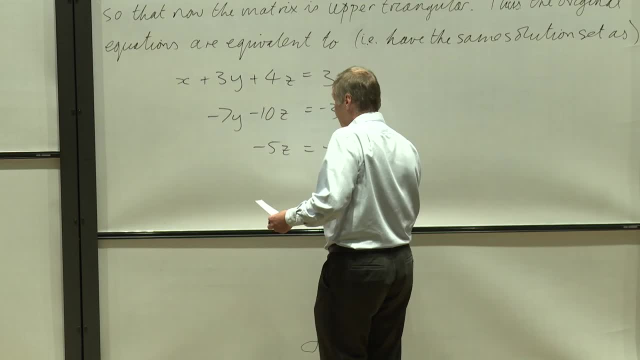 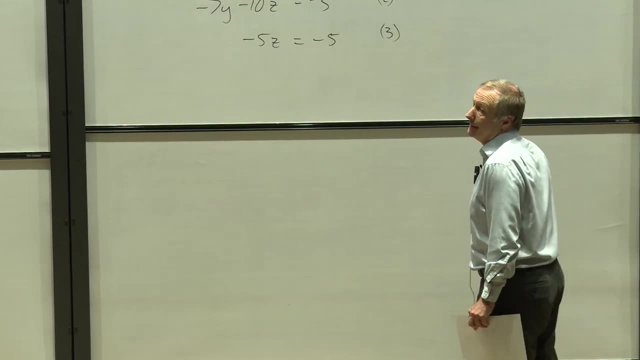 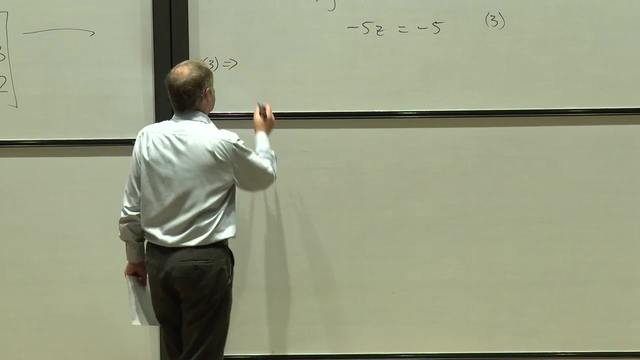 to minus 5.. So I'm going to call these 1,, 2, and 3, which I've not labeled so far, And immediately you can see from equation 3, what does this tell us? This tells us that z is. 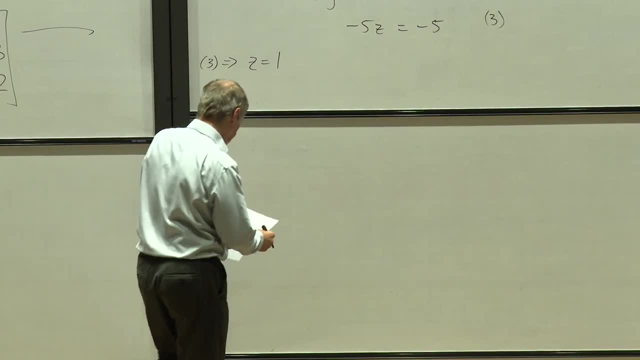 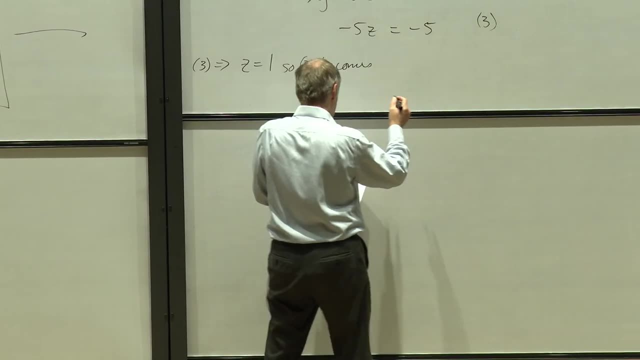 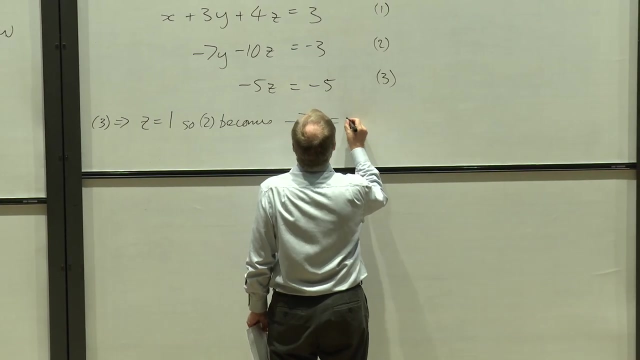 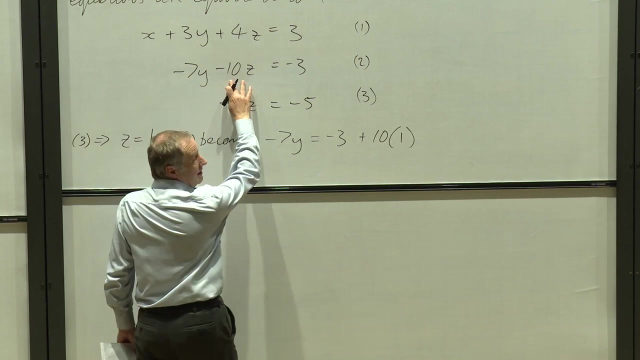 equal to 1.. All right, And so 2 becomes z Minus 7y. Oh, minus 7 times y is equal to minus 3 plus 10, lots of 1.. That is, I've simply moved that term, now that I know what z is, onto the other side, And minus 3 plus. 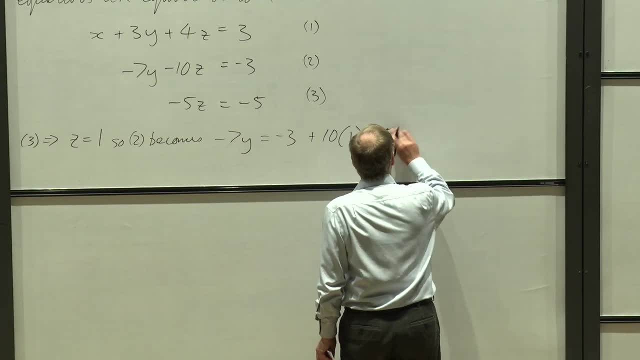 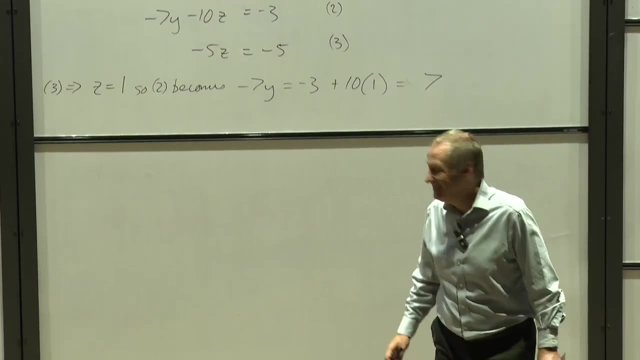 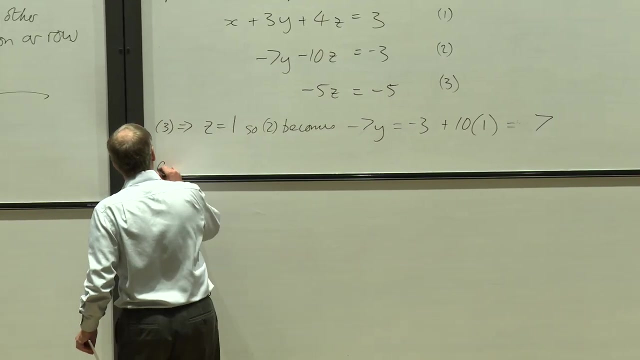 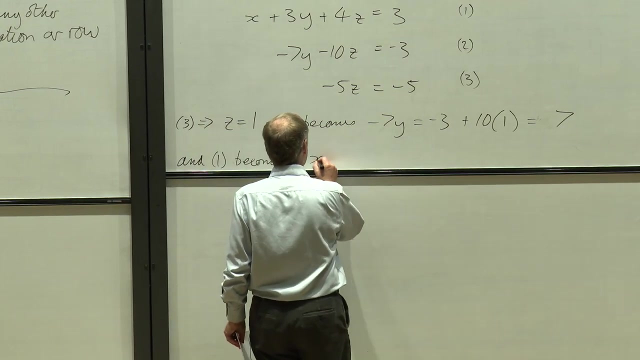 10 is minus 7, isn't it? Oh, minus 7.. Plus 7, right, am I right? Minus 3 plus 10 is plus 7.. And then, once the equation becomes x, so this one can't change, but it's essentially x, And then also equation 1 becomes x is equal. 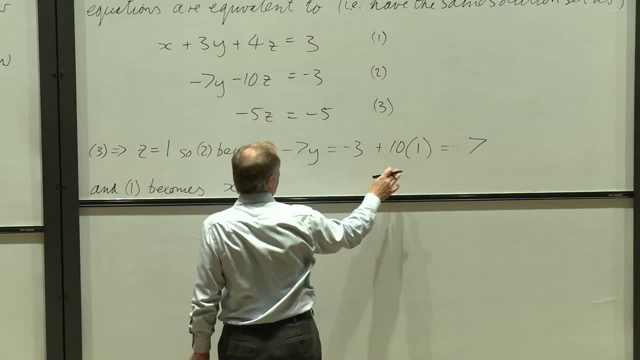 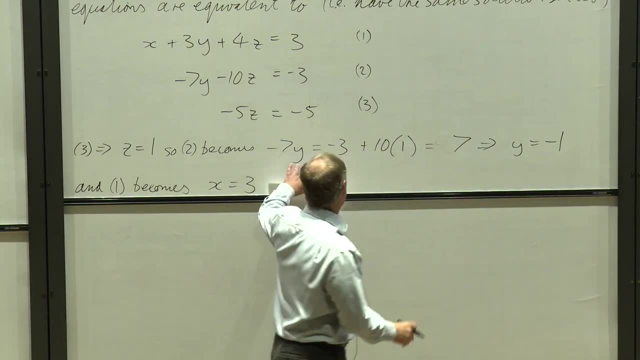 to 3.. That's this guy. Essence 2 is minus 2 and minus 3. lots of y. Well, not, y is So y is now minus 1,, by the look of things, right, All right. Minus 7y equals 7.. 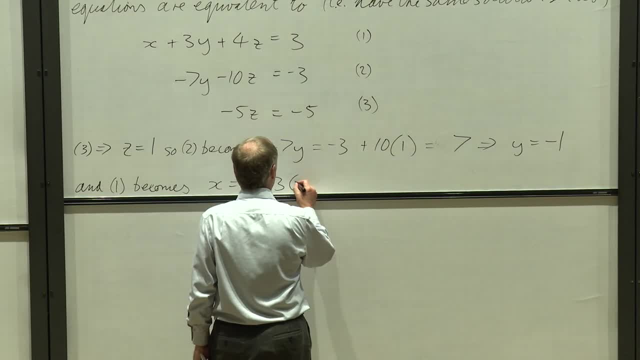 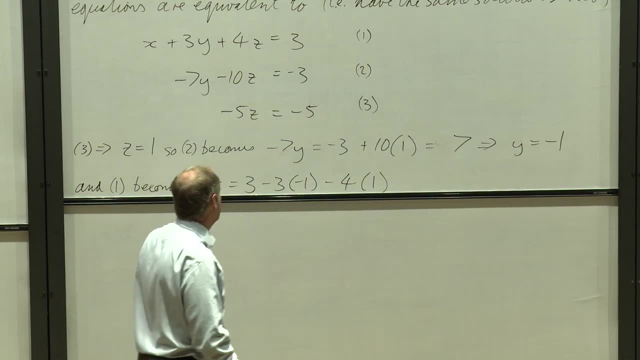 Yes, sam halt narratif and sk 남 끼투 and sam halt narratif and sk에도ff. So 3 minus 3, lots of minus 1, minus 4, lots of what z was and z was 1.. 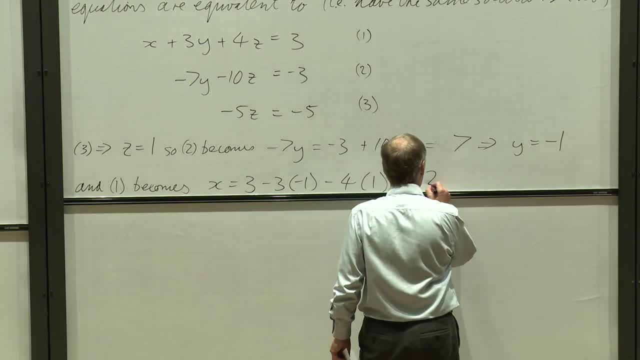 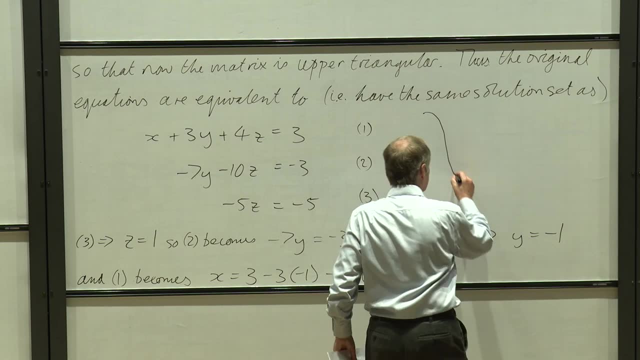 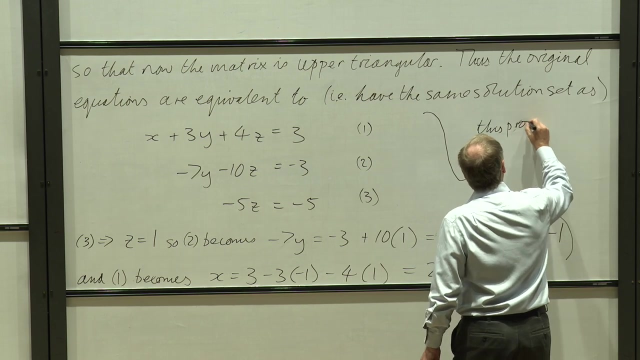 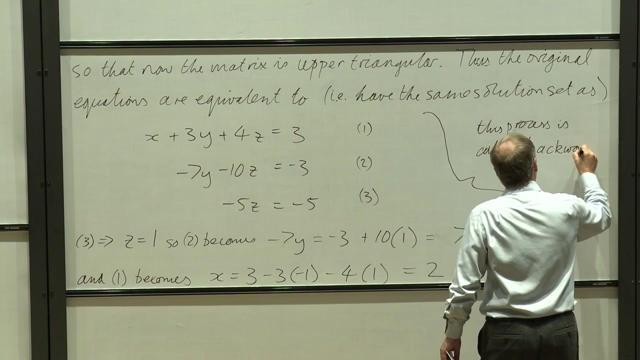 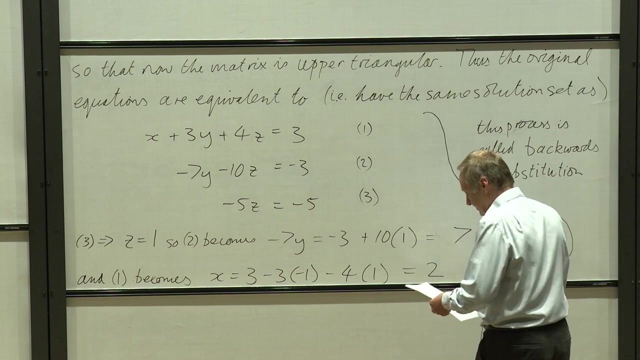 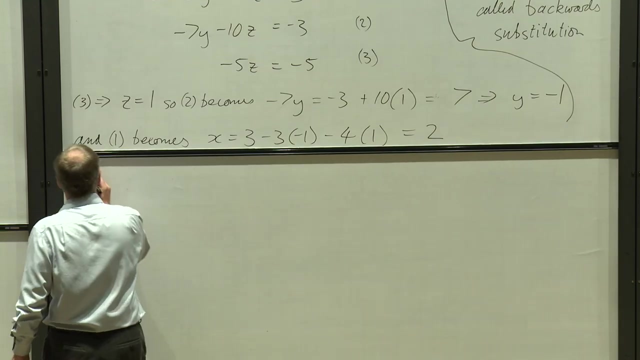 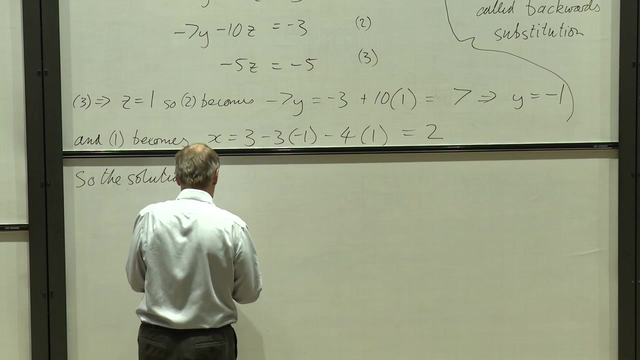 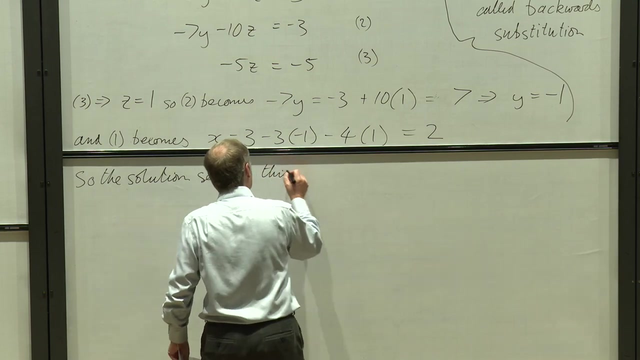 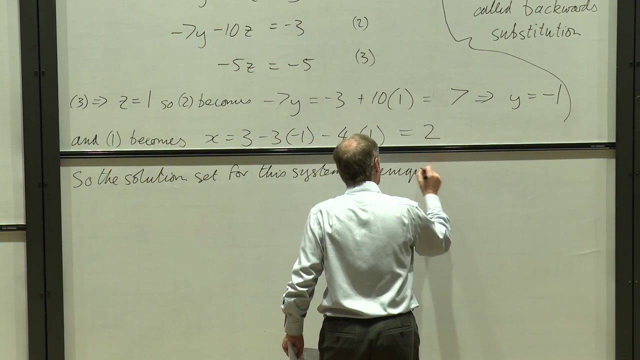 And so this is equal to 2,. OK, This process is called backwards substitution, OK, And now we finally have got the solution set. So the solution set, well, the solution here. OK, the solution set for this system is unique, OK. 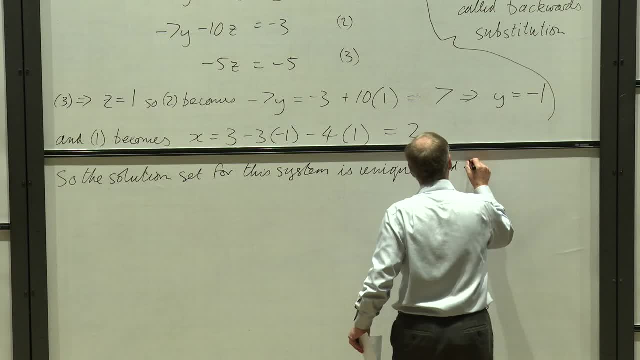 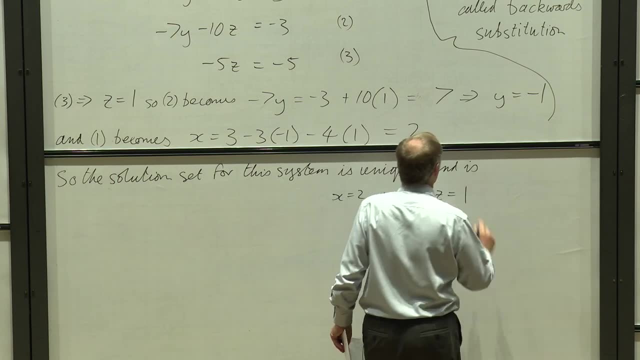 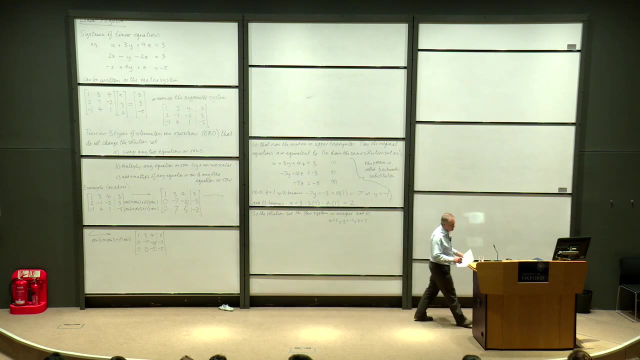 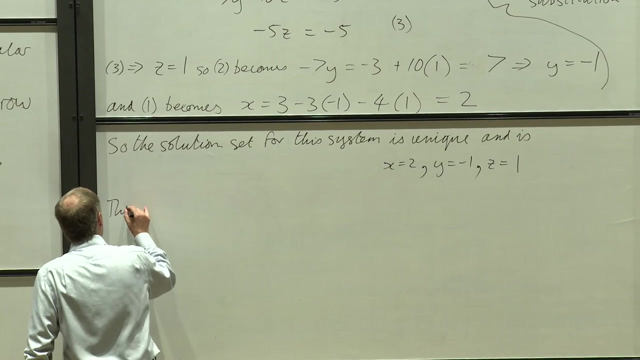 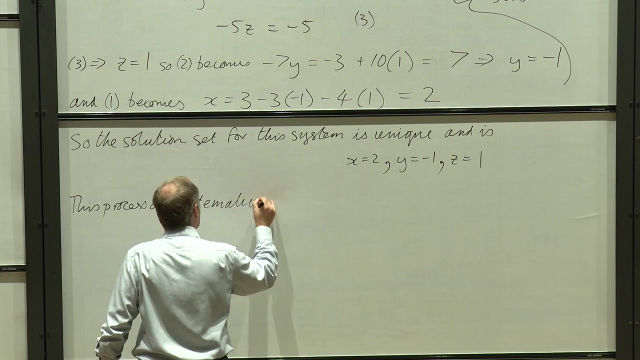 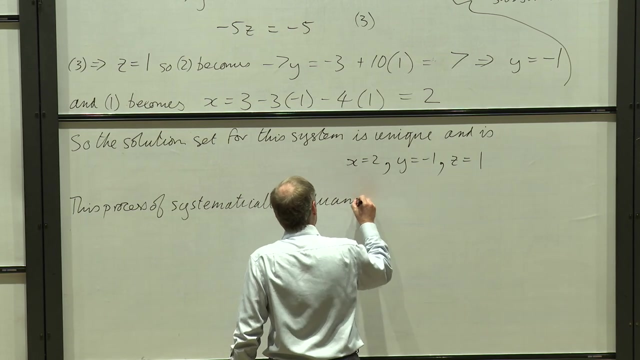 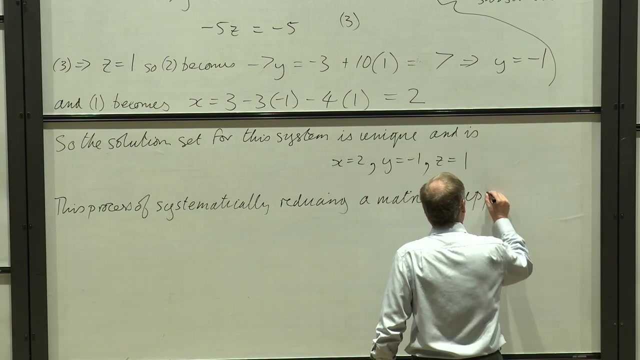 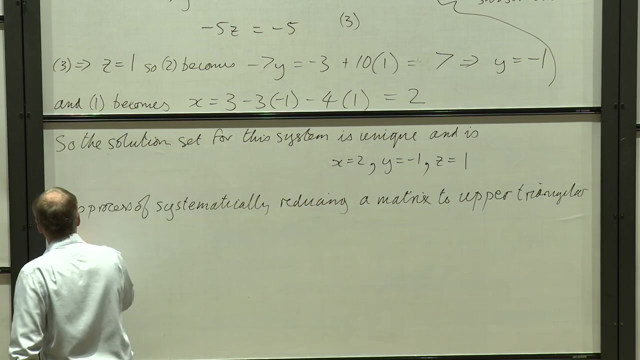 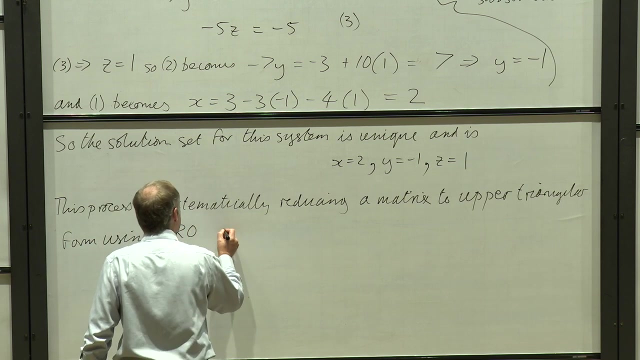 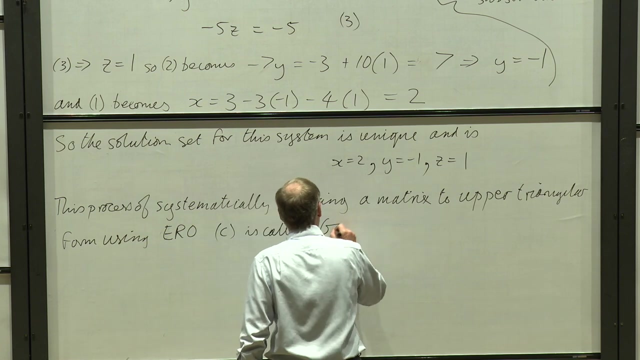 OK. And is, x is 2. And y is minus 1. And z is 1.. OK, So this process, This process of systematically reducing, I could say reducing a matrix to upper triangular form, using EROC, OK, what we call C over there is called Gauss or Gaussian. 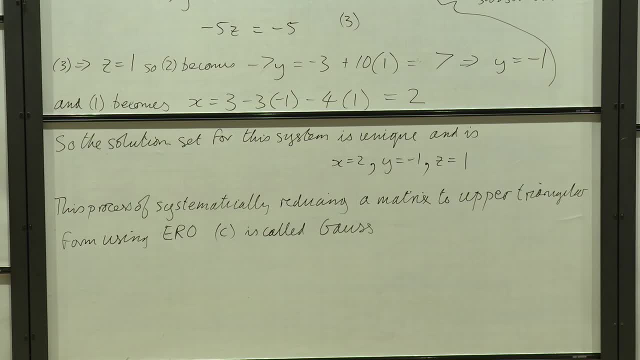 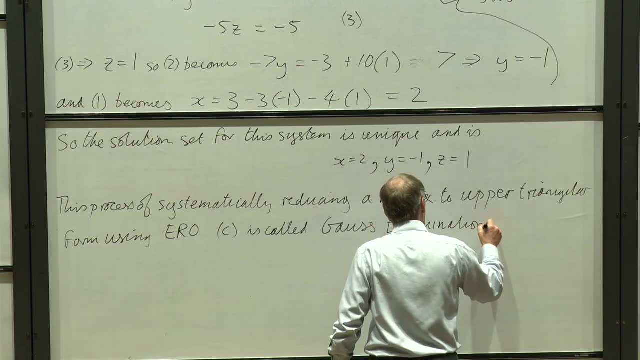 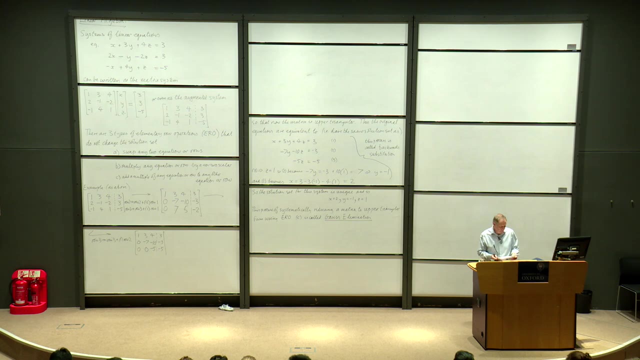 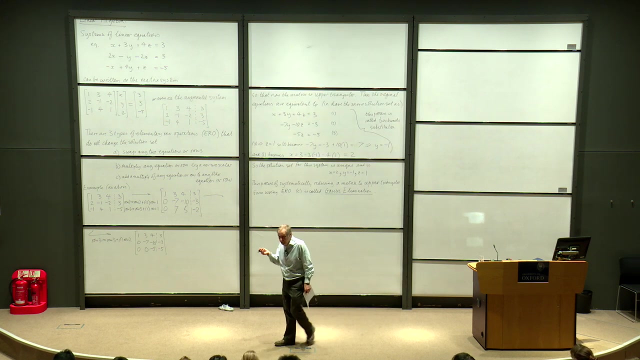 You've all heard of Gauss, right? Gauss or Gaussian. I call it Gauss or Gaussian elimination, OK, OK. So all you've done is you've systematically introduced zeroes into the lower triangle and that's your Gaussian elimination, And it's clearly one way of finding a solution set here. 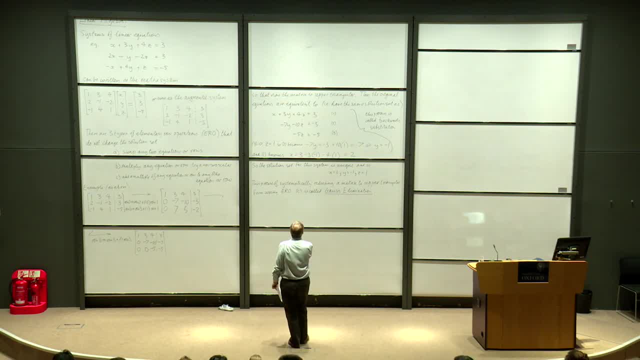 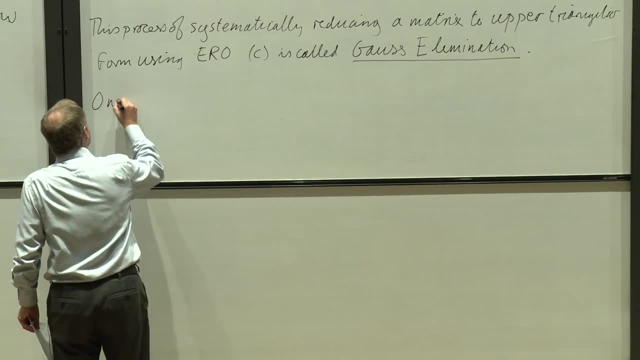 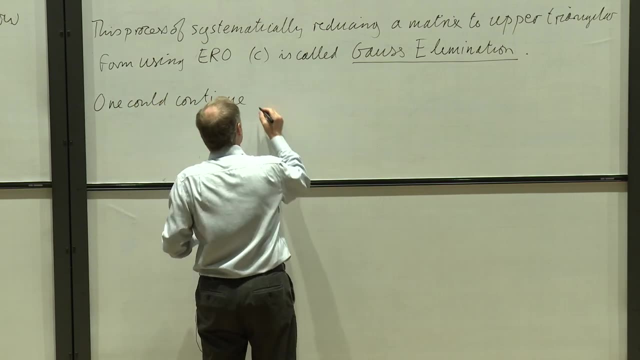 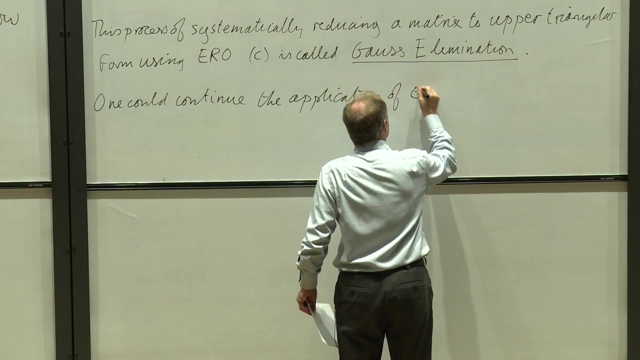 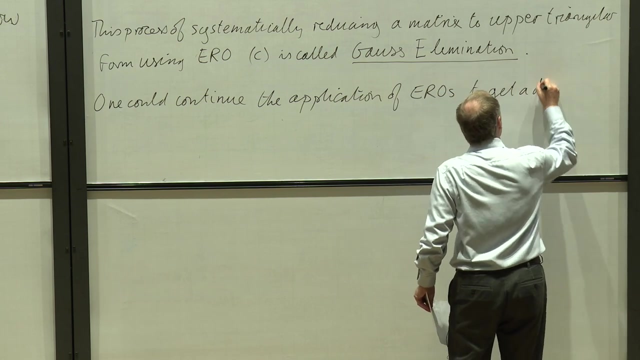 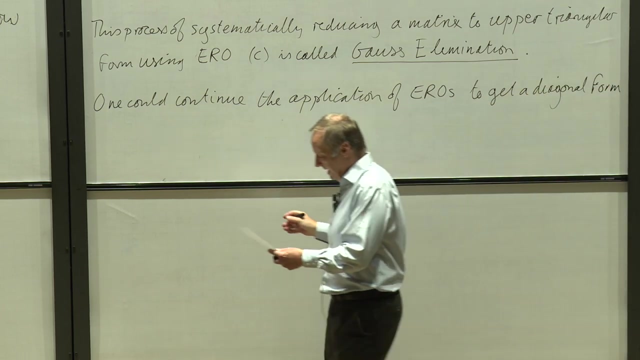 No question about that, and that's what we've done. OK, So one could continue. OK, The application of EROs, elementary row operations. OK, to get a diagonal form. OK. So what happens there? we start off with what we have. 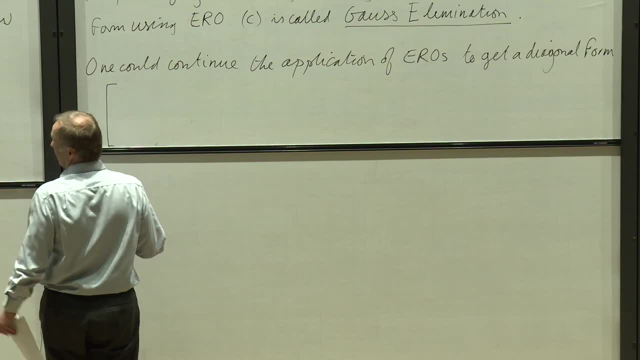 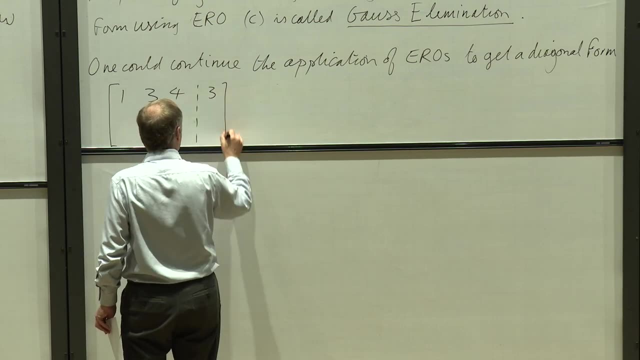 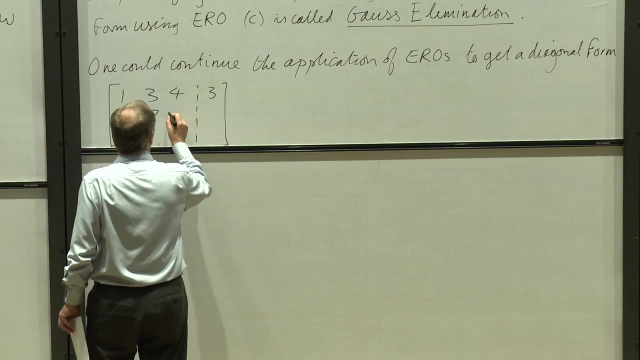 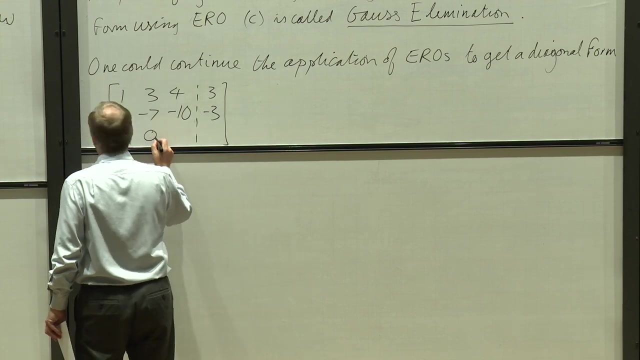 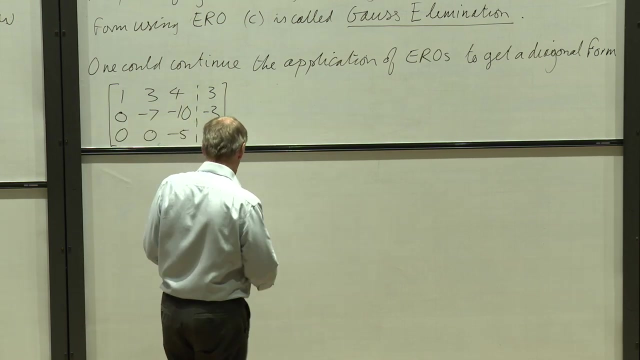 The application of EROs. OK, upper triangular form. So I take it from here: 1, 3, 4 and 3, 0 minus 7. this is 0, not 6 minus 10 and minus 3 and 0 and 0 and minus 5 and minus 5.. Okay, and what can I? 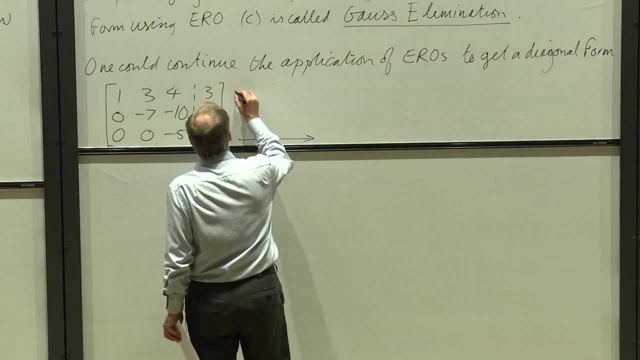 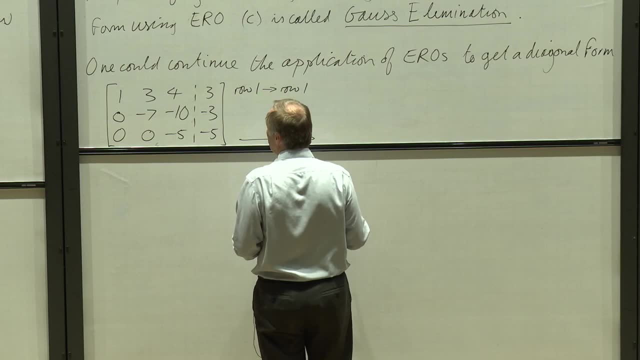 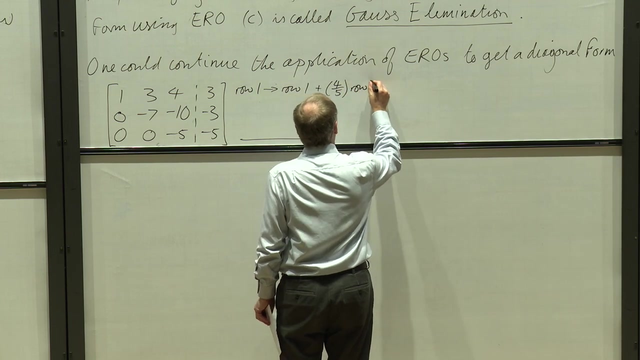 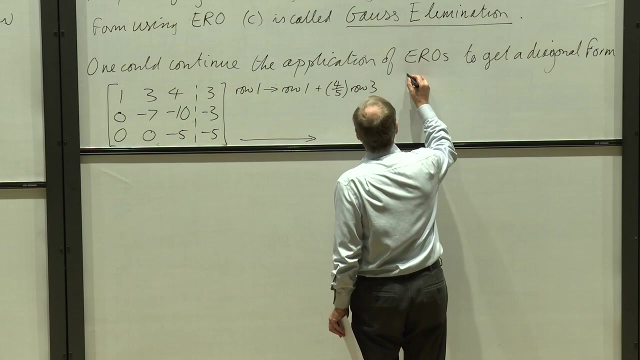 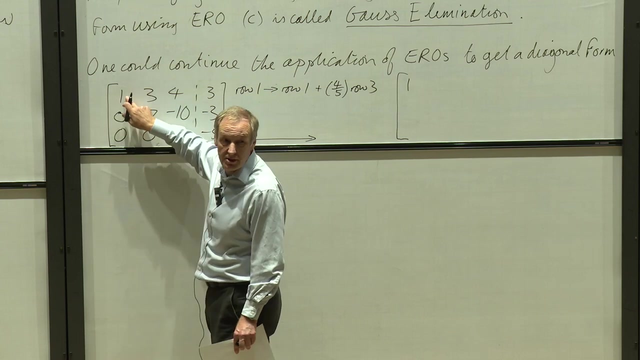 do now? I can do the following. I can say: row 1 becomes row 1, okay, plus 4 fifths of row 3.. Okay, so if I do that, then I get well, the first row becomes 1, because 4 fifths of 0 add to 1 is going to change it clearly. I get 3. similarly. 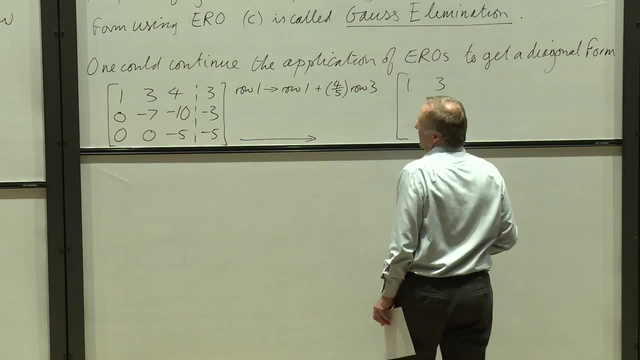 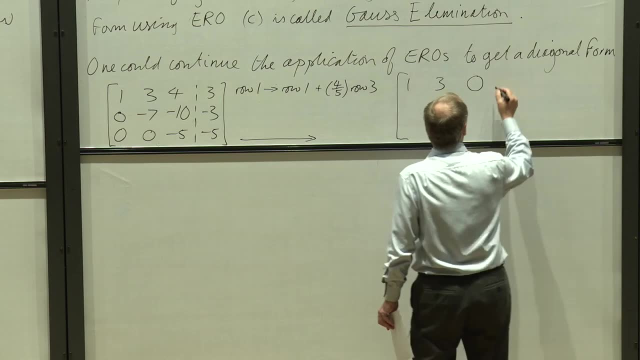 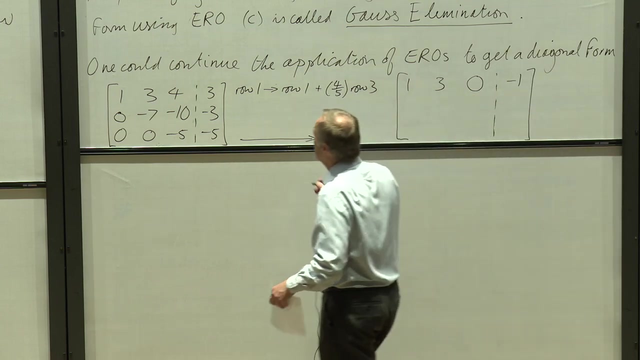 because 4 fifths of 0 add to 3 doesn't change it, but 4 fifths of minus 5 add to 4 gives me a 0. Okay, and the right hand side becomes, in fact, minus 1, and I'm also at the same. 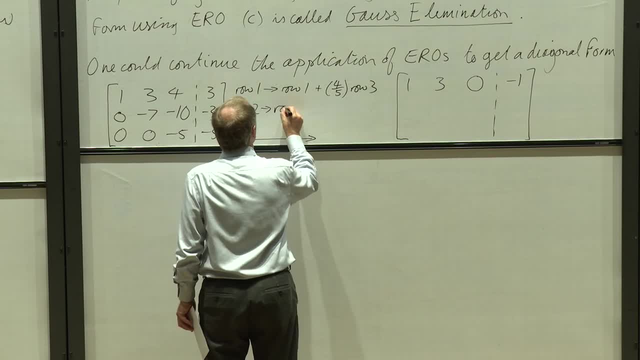 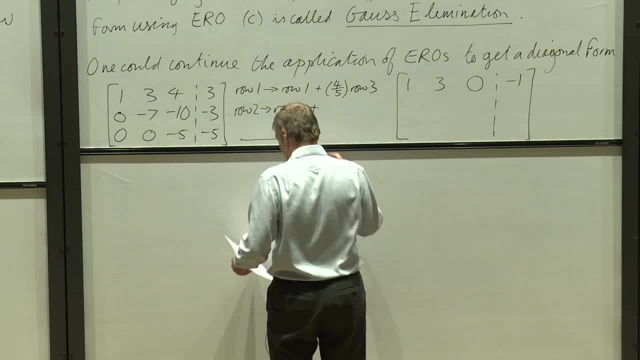 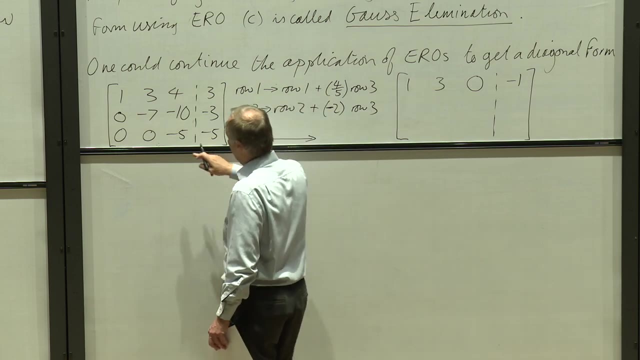 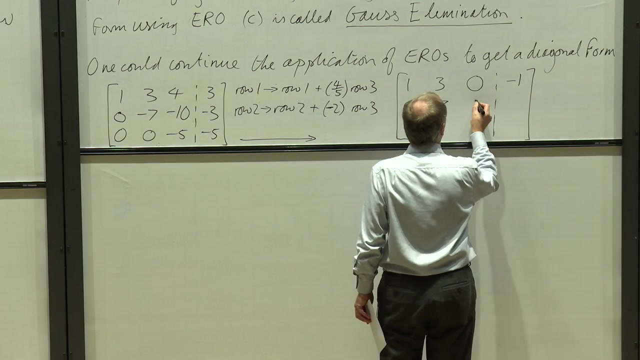 time going to do. row 2 becomes row 2. okay, plus what am I going to do? here looks like minus 2, lots of row 3.. So if I add this minus 2, lots of this to this row, I should get 0.. So again, I get 0 and 7 and 0 and the right hand side becomes 7. 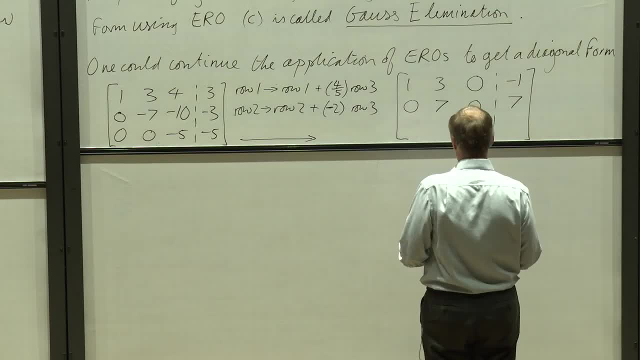 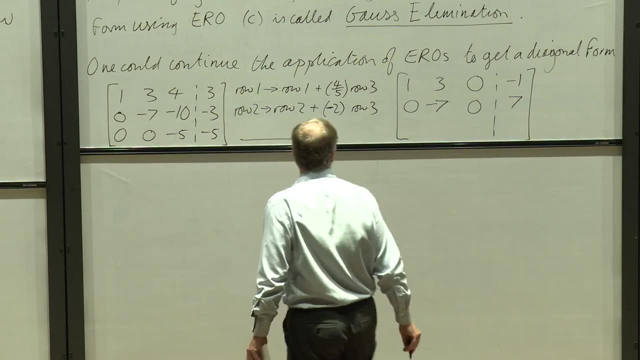 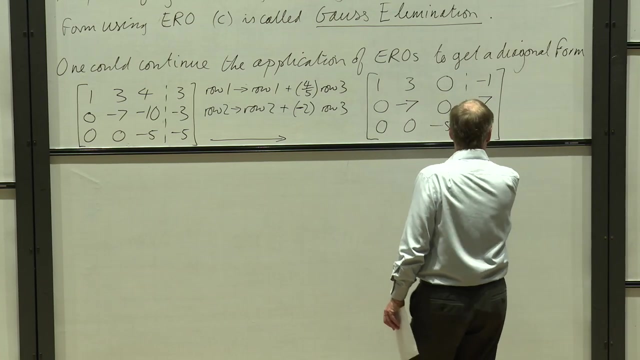 and the one, hmm, minus 7. thank you very much. Didn't change it, because I added 0 times here and the last row becomes 0. well, it stays as it was: 0, 0 minus 5 and minus 5. so now we just have to add some multiplications. 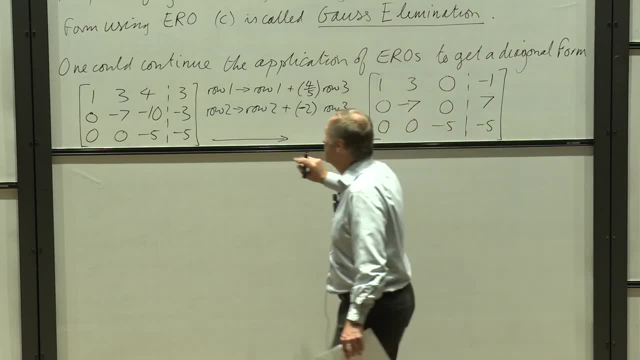 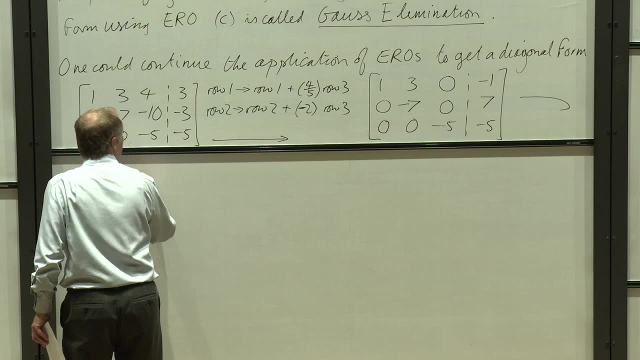 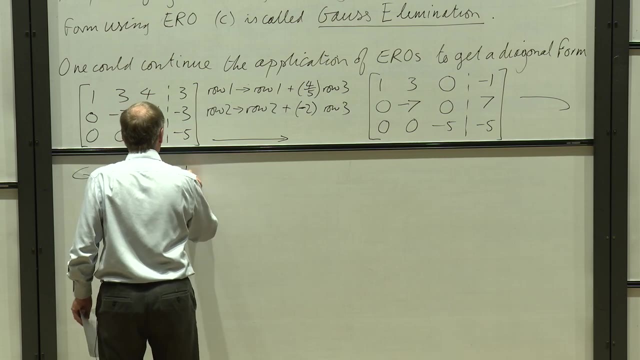 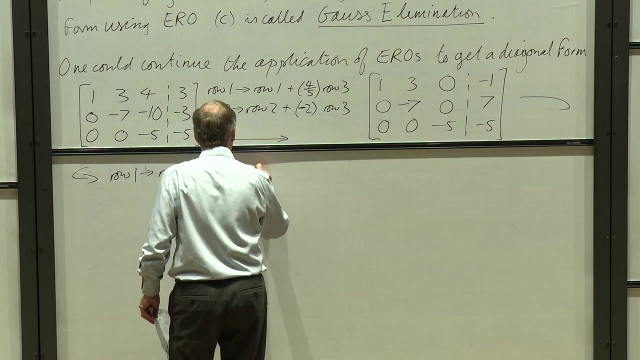 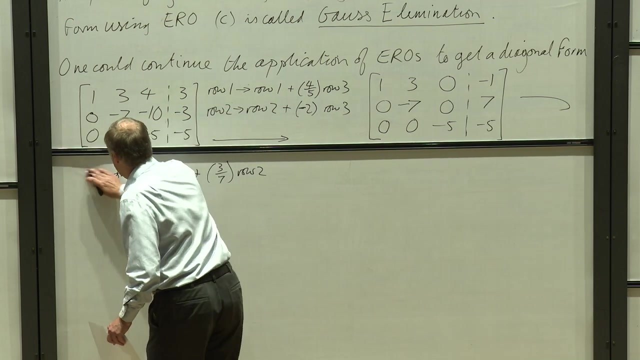 of this to this to make a zero. So if we again carry on and then we have Rho1 becomes Rho1 plus and this is 3 sevenths, isn't it of Rho2.. If we get 3 sevenths of Rho2, then this gives us the following. I should say this here: 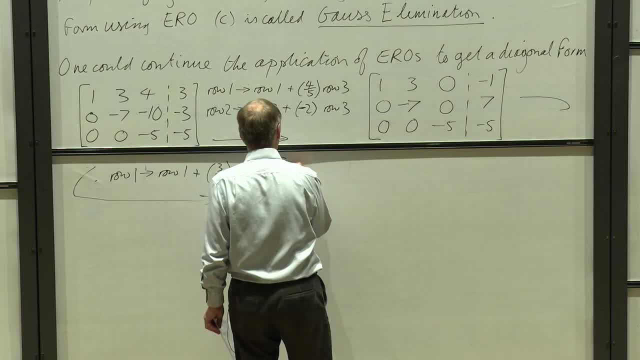 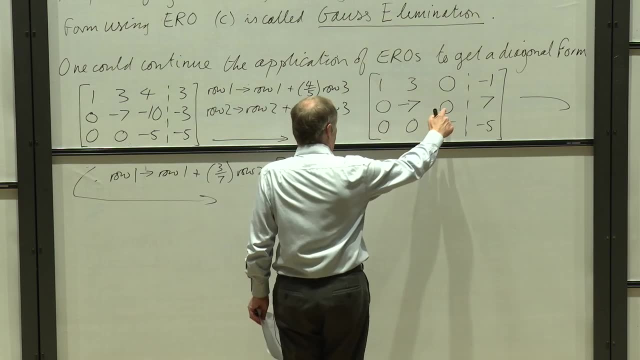 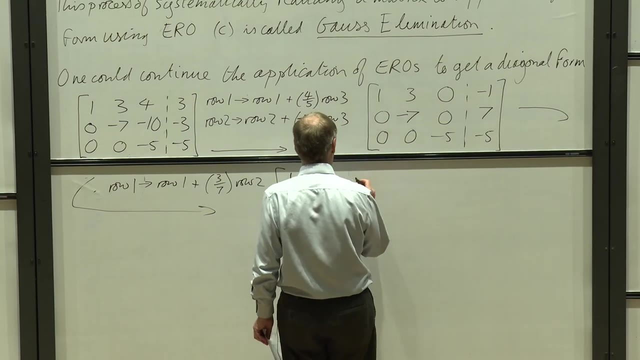 gives us the following: 1,. again, this doesn't change. this becomes a 0. now that's the 3 sevenths. Fortunately, this doesn't change. you can see why we use Rho2 right. so this is a 1, what I'm saying, and then this is 0, then this is minus and this: 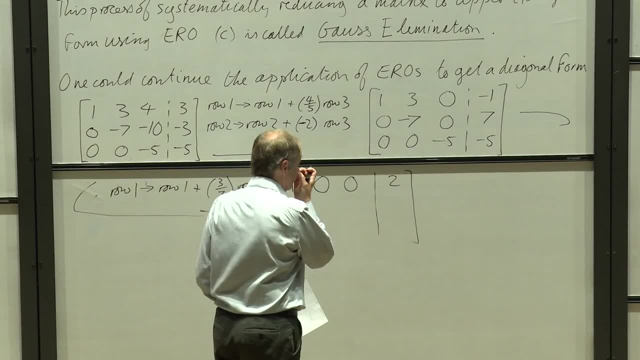 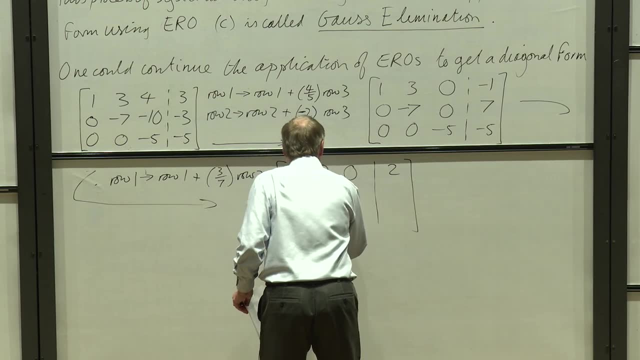 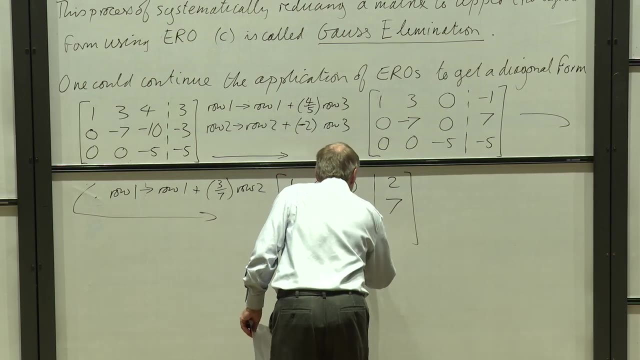 becomes 2.. 3 sevenths of this, and then the second row is 0 and minus 7 and 0 and 7.. And the final row is 0, 0 and minus 5 and minus 5.. And I'm going to give this a label, So 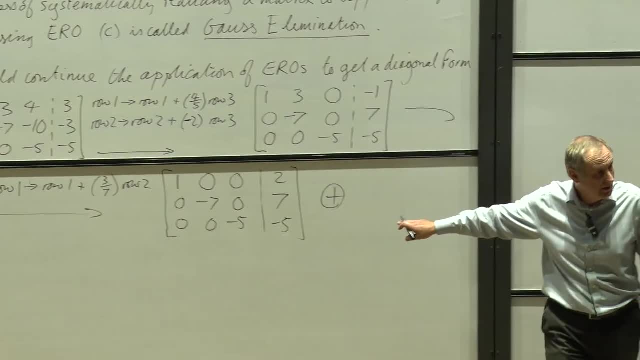 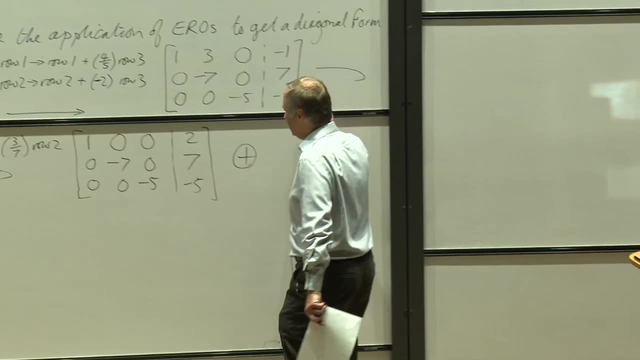 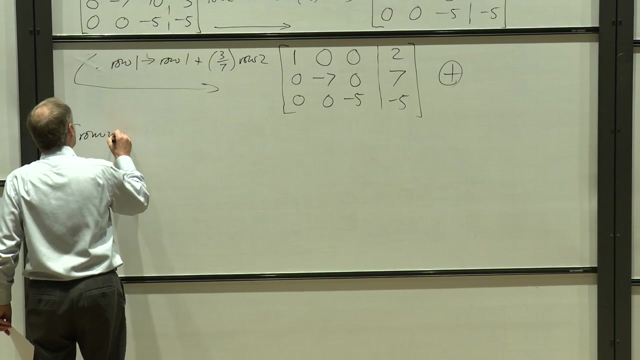 my labels are all together local, so today's label plus is this equation: Okay. if I write plus tomorrow, it means whatever equation I say tomorrow, Okay, And you can see from here the solution set, from which the same, of course it should be. 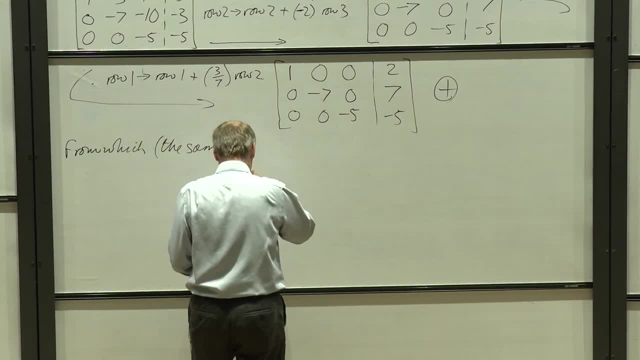 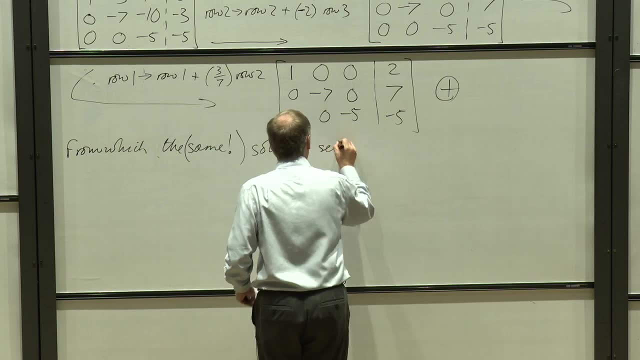 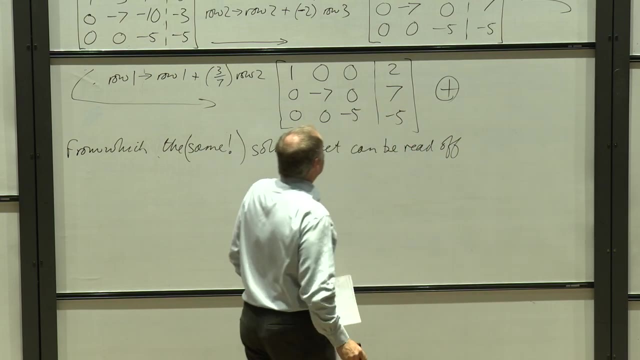 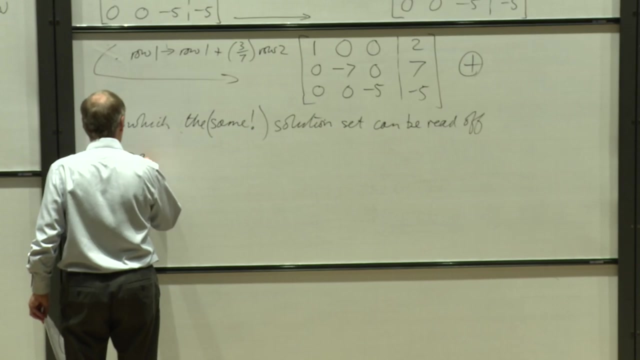 that solution set. Okay. Okay, so you can actually get a diagonal form, if you wish, to This. and here's an interesting verb you've perhaps never heard of before this: zeroing. okay, so this is the participle of the verb to zero. 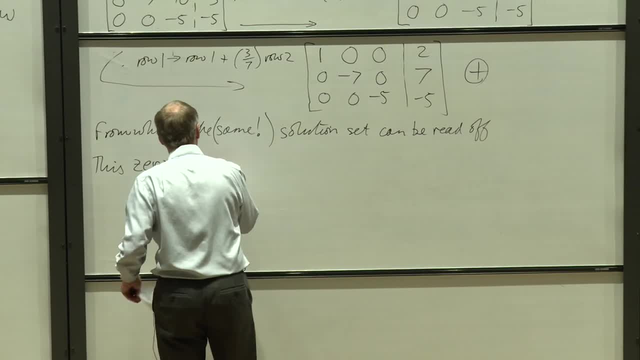 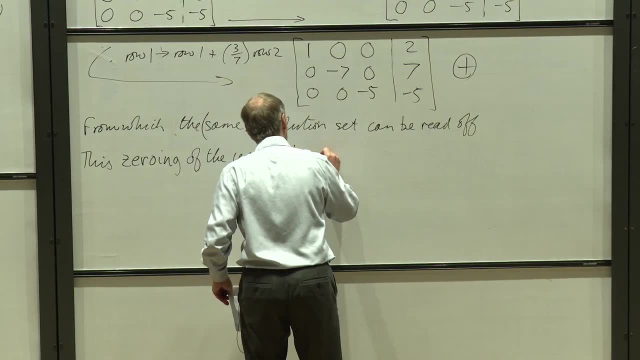 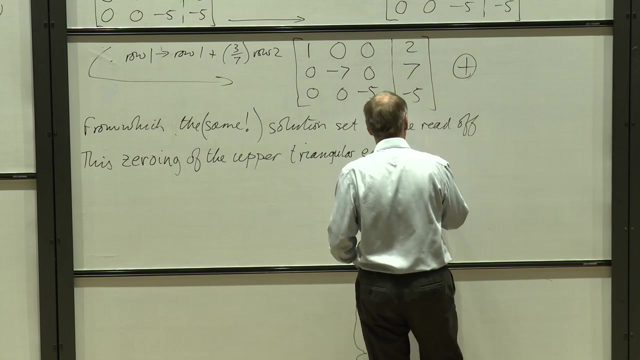 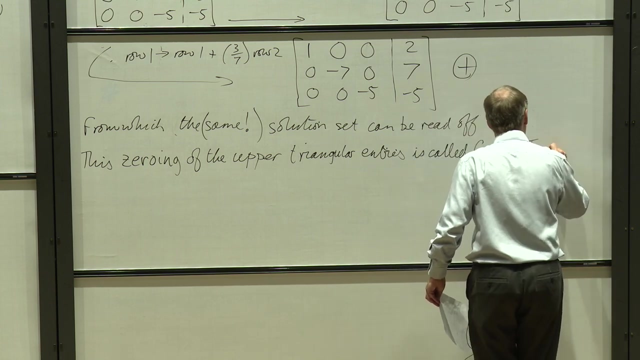 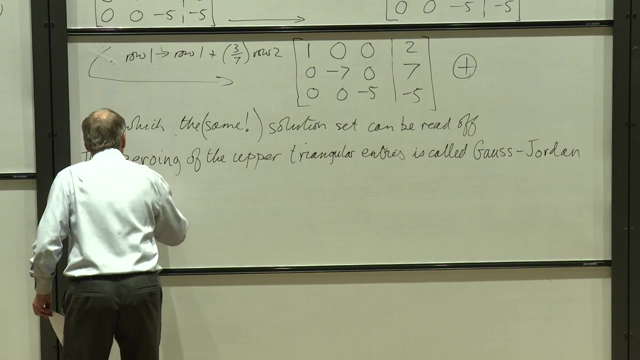 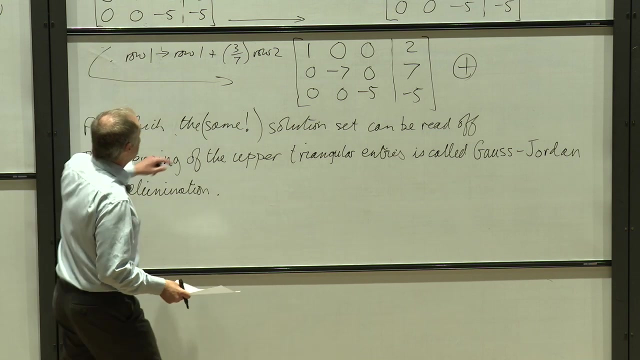 this zeroing of the upper triangle is called. it's also named after Gauss, so Gauss and also Jourdain, So in English, Gauss-Jordan elimination. Okay, so it depends what your purposes are whether you want to do Gauss elimination. 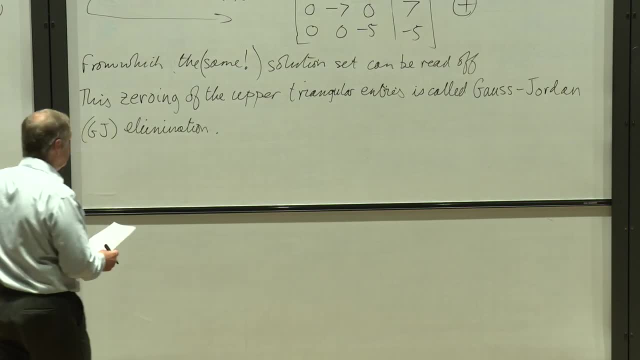 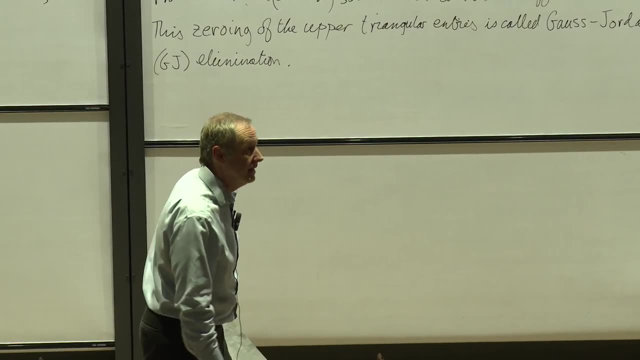 or whether you want to do Gauss-Jordan elimination, Okay, but you can see what I've done right And this example shows you exactly how you do this right, And you can see why I took here the multiples of row three. 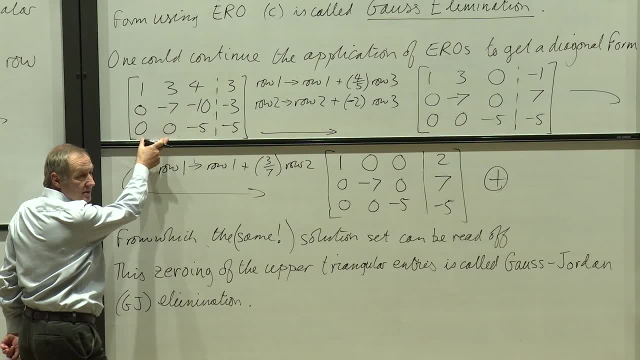 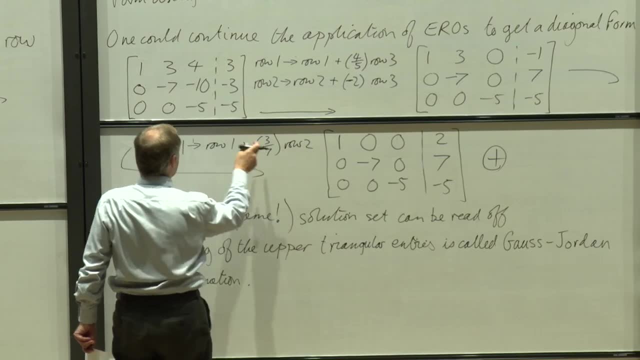 because I've got these two zeros. so by doing these two zeros I don't change anything in these first two columns, right? And then here I use row two because I don't want to reintroduce something into the third position, right? 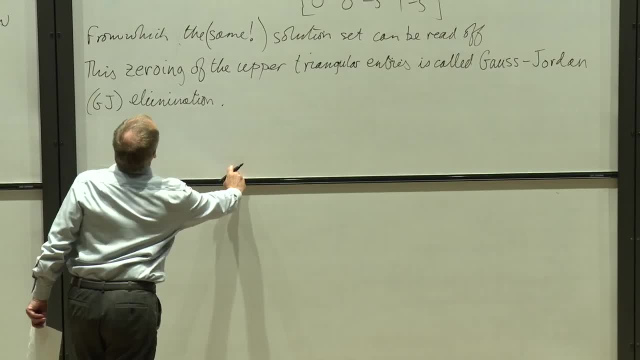 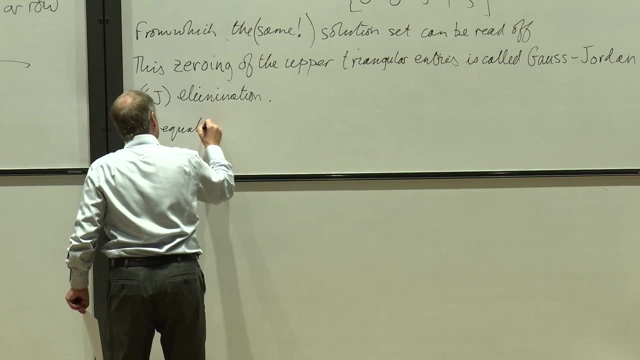 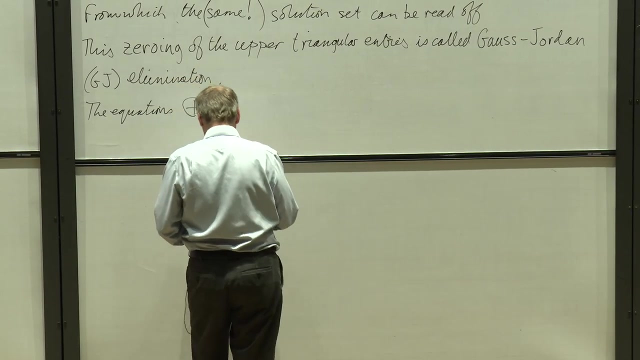 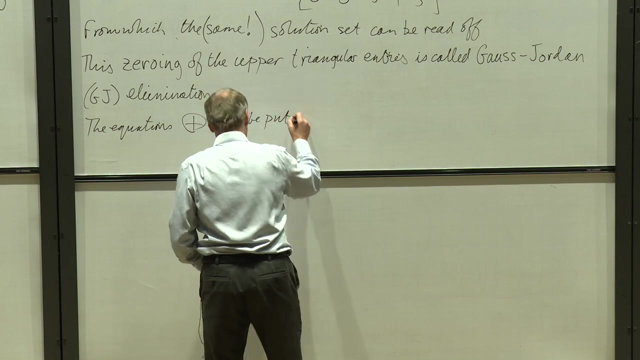 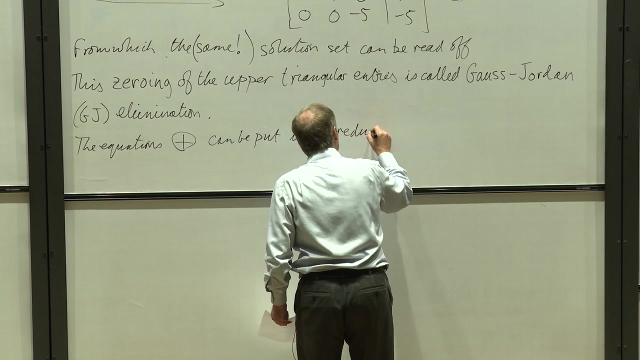 So this is the system, This is the systematic treatment of this thing, right, Okay, so the equations plus. the equations plus here can be put- sorry, I said the equations plus, okay, can be put into a reduced row. echelon. 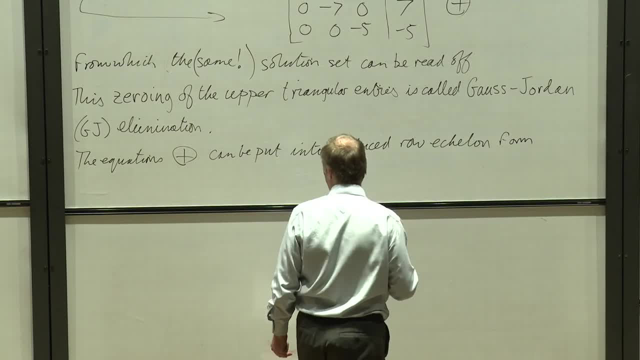 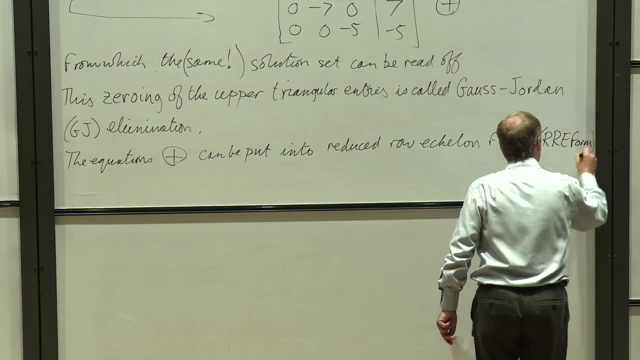 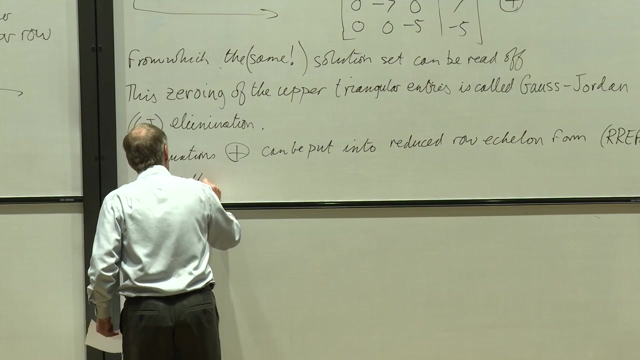 Okay form. That's clearly a mouthful, even for me, so I'm not going to call it that. I'm going to call it RRE: reduced row echelon form. Okay Okay. In which the leading entries or the leading non-zero entries. 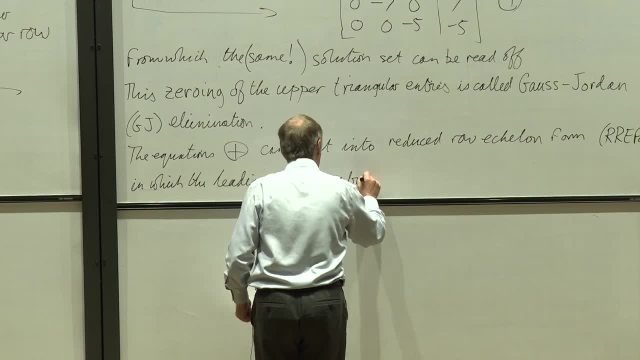 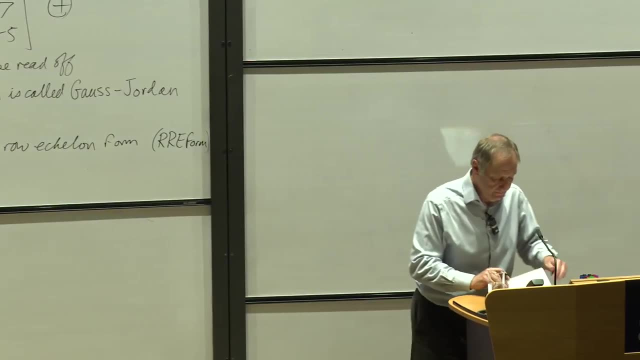 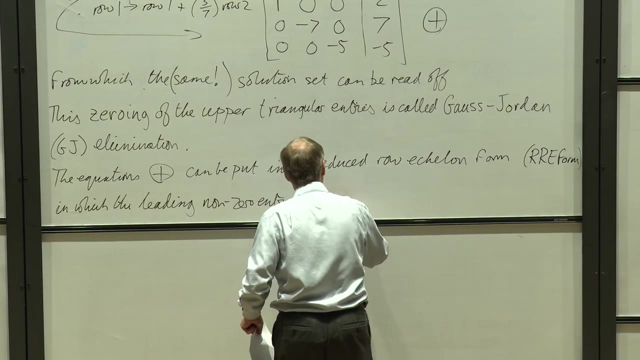 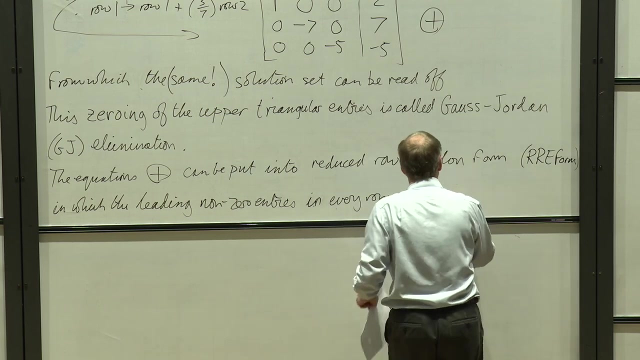 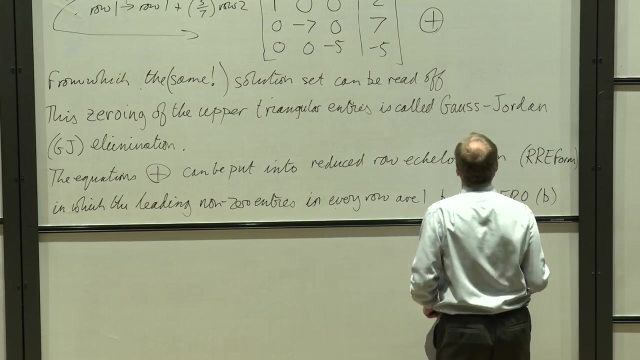 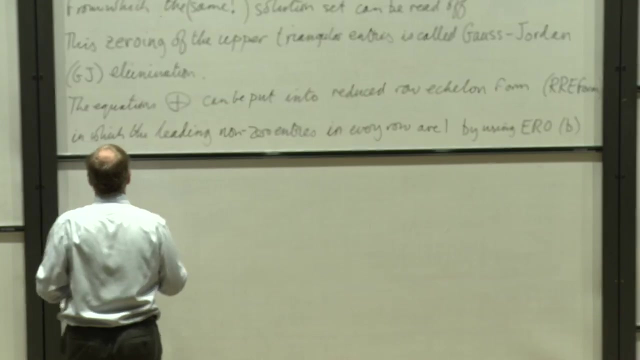 are one. okay, I should say in every row. Okay, I'll have the number one by using ERO B. In other words, it's quite clear. you can scale right, And I'll just do this very briefly and then I'll stop. 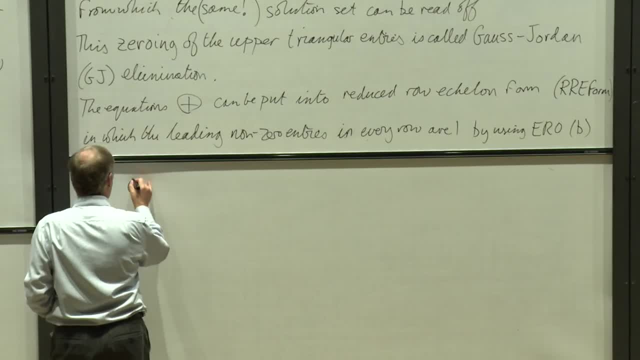 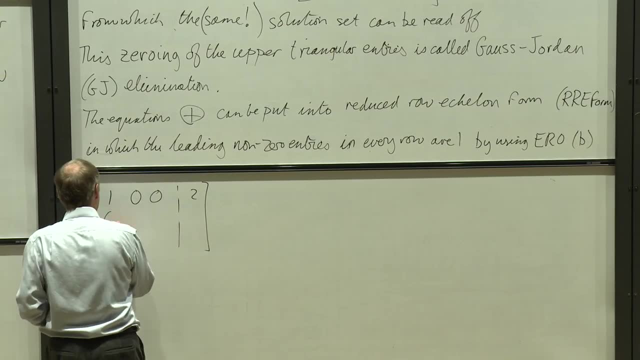 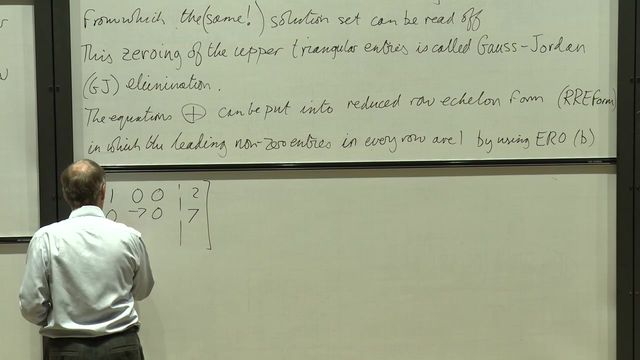 So I've got 1, 0, 0, 2.. That's already in reduced ratio, one form, so I don't need to do anything with that. 0 minus 7, 0, 7.. Okay, and I've got 0, 0, minus 5, minus 5.. 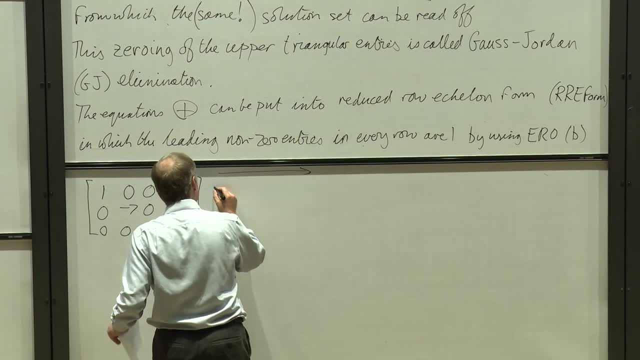 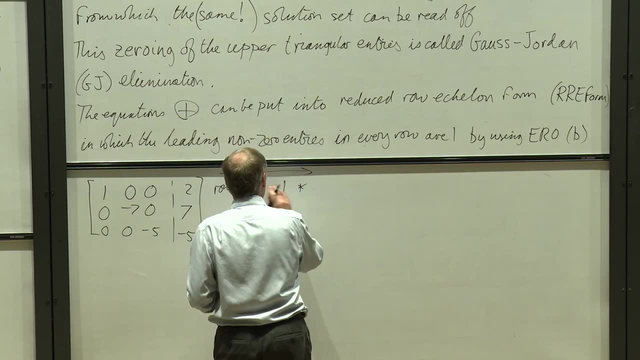 And all I'm going to do is I'm going to do scaling. Rho 1 becomes Rho 1 times what Becomes 1 times Rho 1.. This is obviously a sort of irrelevant thing to do, right. 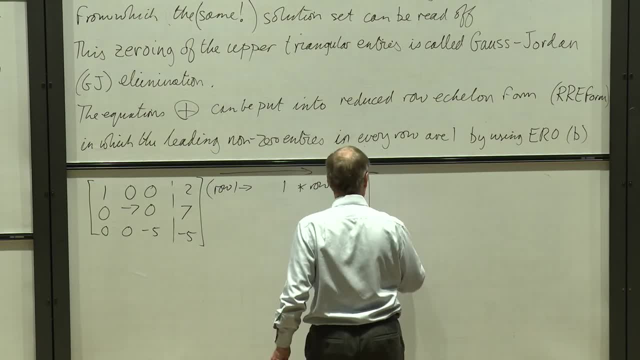 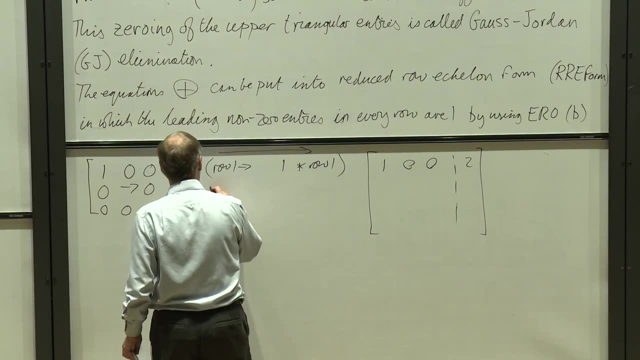 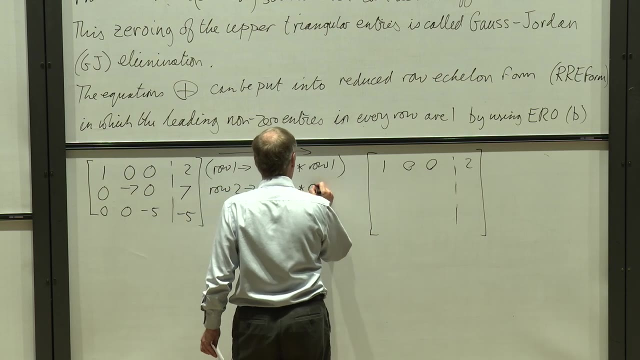 Because I'm already in ratio, one form, Reduced ratio, one form, that's this Okay. And then the second one is obviously not so trivial: Rho 2 becomes minus 1, seventh of Rho 2, which gives us 0, 1, 0, minus 1.. 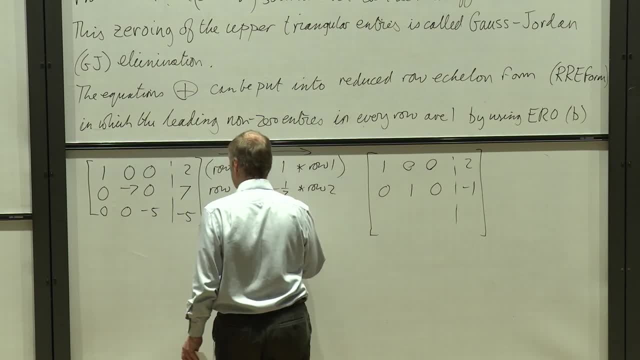 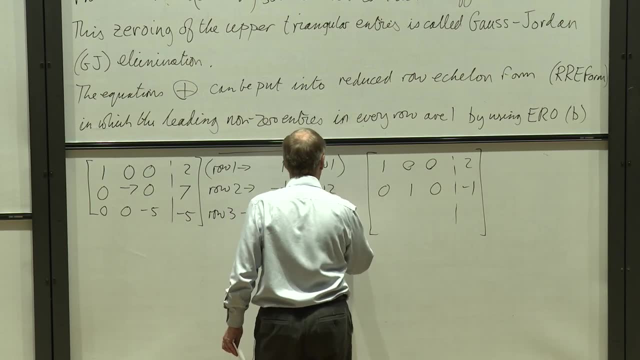 And Rho 3 becomes Rho 3.. Oh, minus a fifth, Minus a fifth times, Rho 3 gives us 0, 0,, 1.. And this becomes. What does it become now? It becomes 2.. 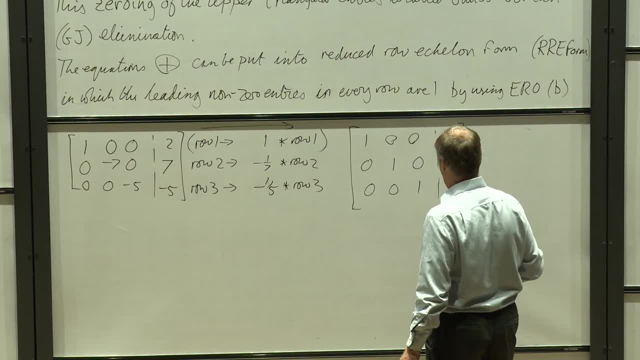 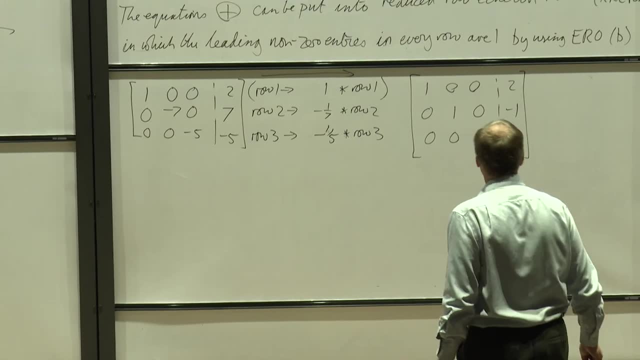 1. Oh, of course, of course, There you go. You can see that I'm not very good at arithmetic, but that's fine, Good, You're all right now. That's very good, You're good at arithmetic. 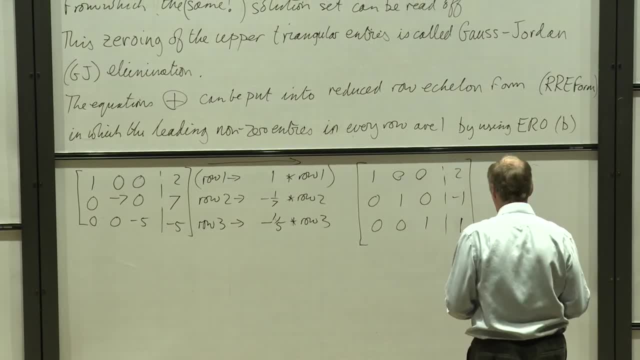 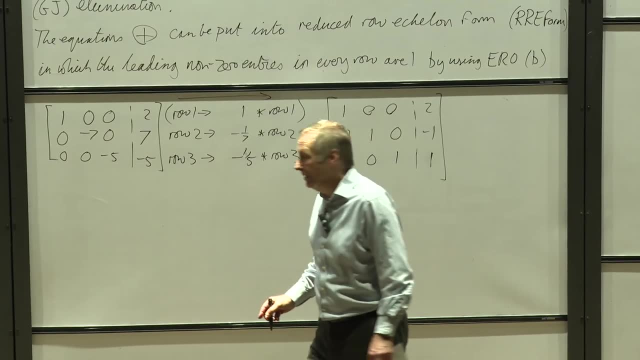 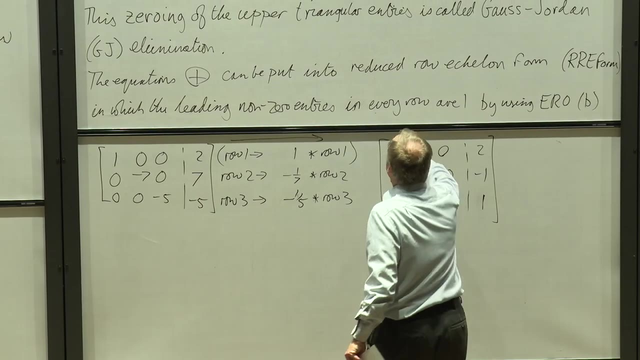 So this is our reduced Rho echelon form And again, you can very clearly see that this is now the solution. Okay, so sometimes this so-called triangular form, what I've called upper triangular, sometimes that's called Rho echelon form. 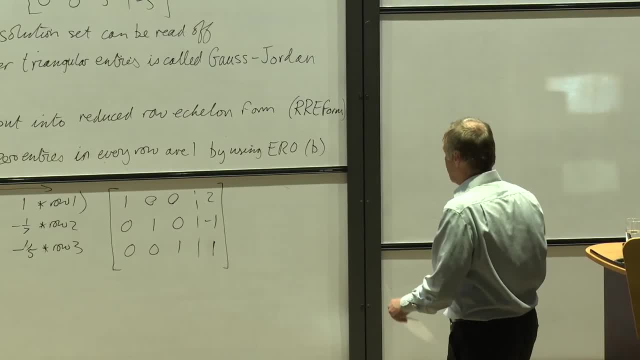 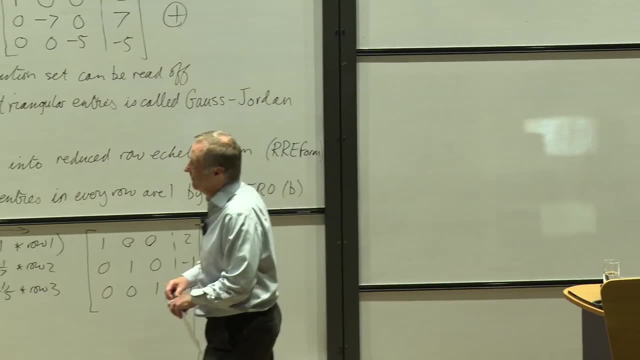 And this is reduced Rho echelon form, But you'll see these different words at different places and at different times. Okay, So this is all we needed to do, That is, elimination to find the solution. Okay, In this case, we could go further. 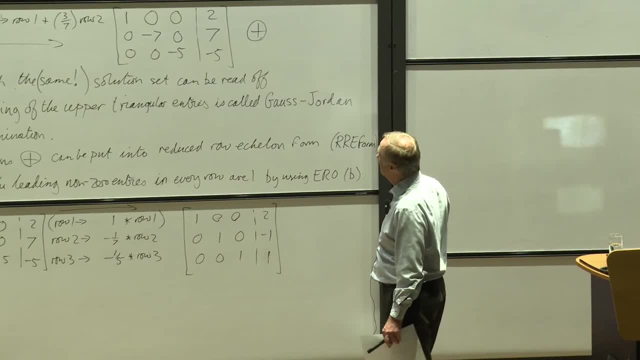 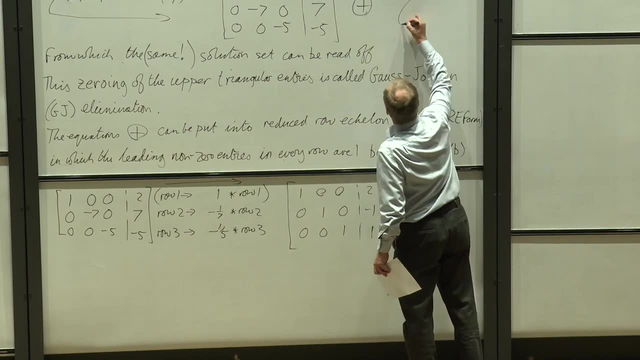 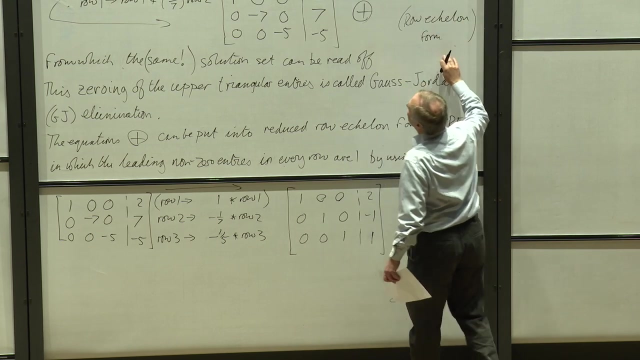 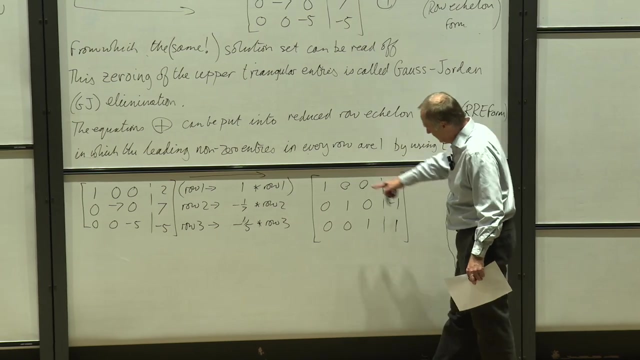 and use Gauss-Jordan elimination to find this form, which is in Rho echelon form. This is Rho echelon form, as I say- And this is Sorry, I must get this right- And this is the reduced Rho echelon formula. 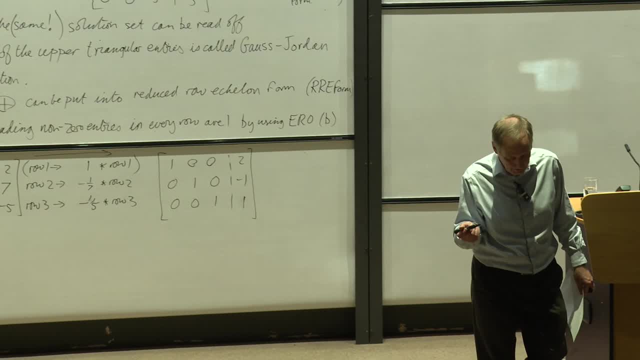 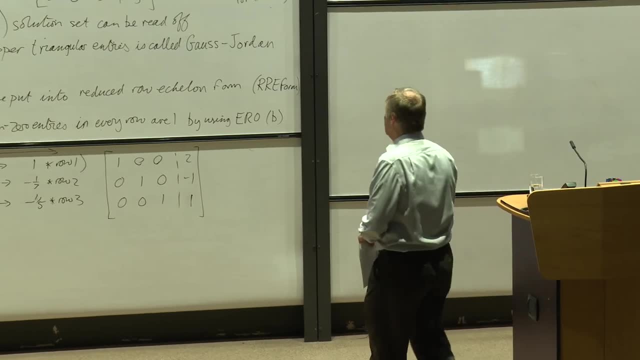 This is the one I'm going to talk about a little bit later, And this is the form that is used quite a lot in the problem sheets. So you'll see this. Okay, I'm just showing you how you can do this. Now you might say, well, okay. 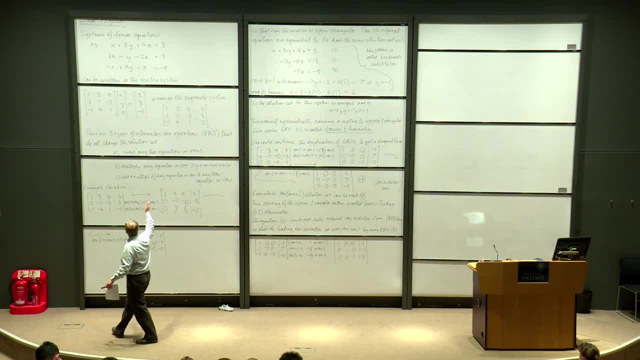 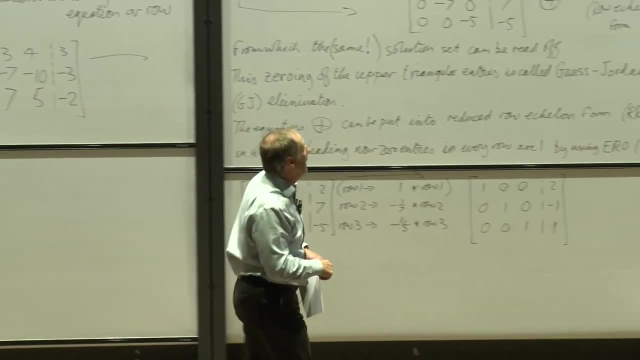 why did I put up three EROs? I've only ever used this one And then, finally, I've used this one to get myself to reduced Rho echelon form And is A ever used, And let me just say that EROA. 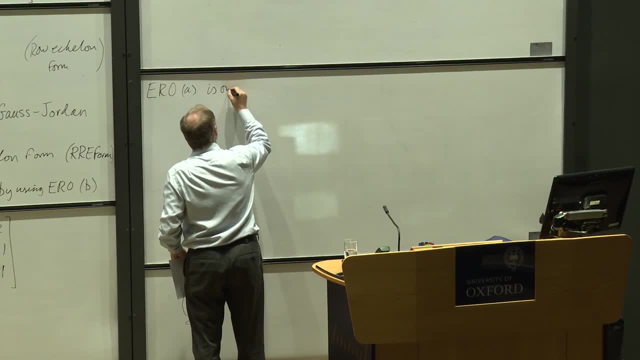 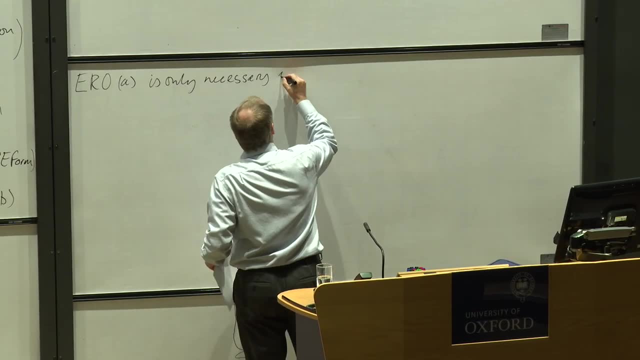 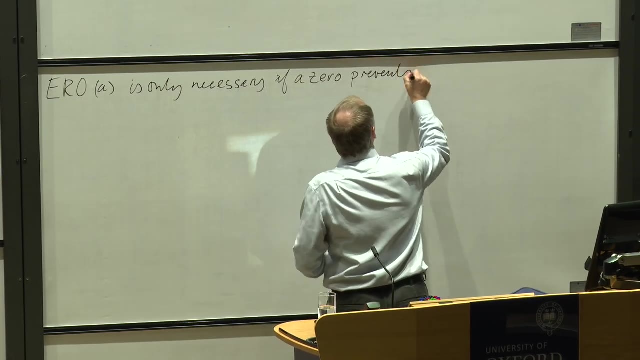 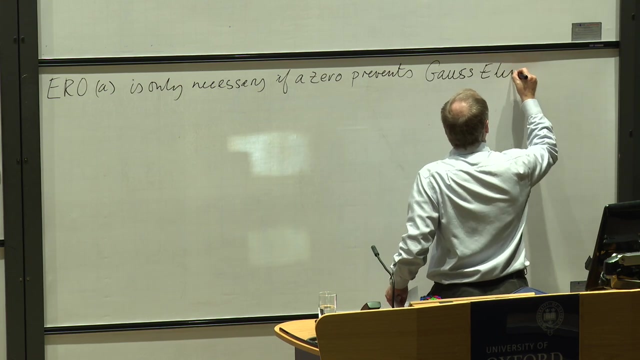 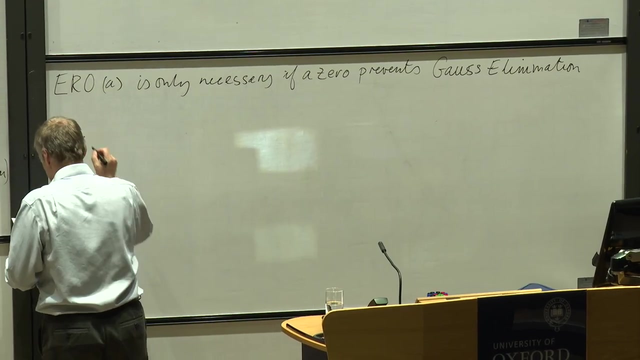 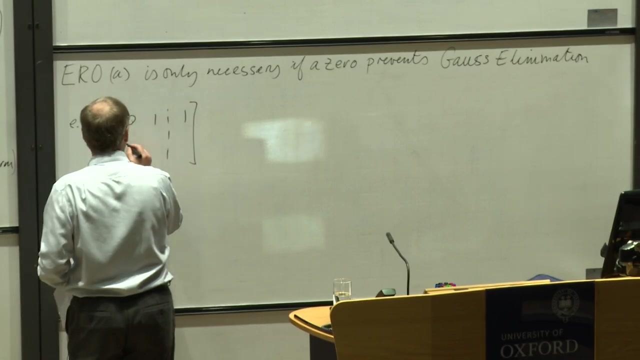 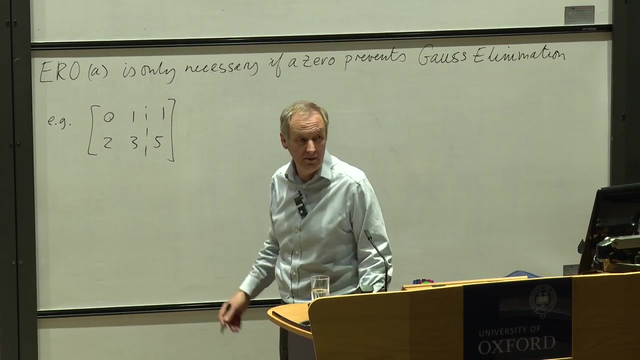 okay, is only necessary if a zero prevents Gauss elimination. Okay. So, for example, if you have the equation simply zero, one partition one And two, three partition five, If you have this situation, then you can't do Gauss elimination. 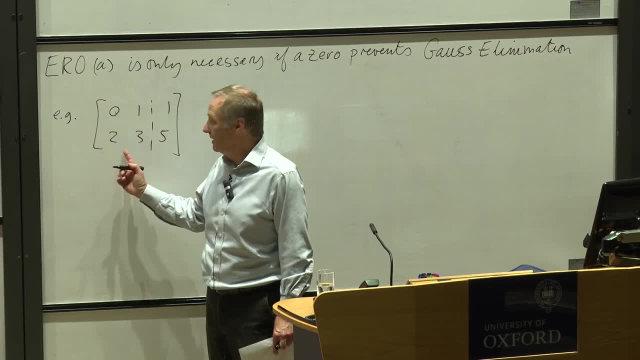 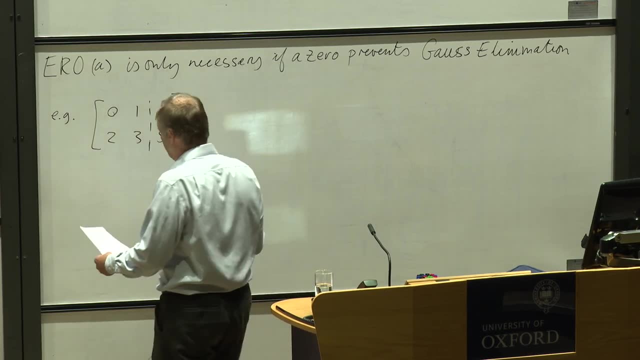 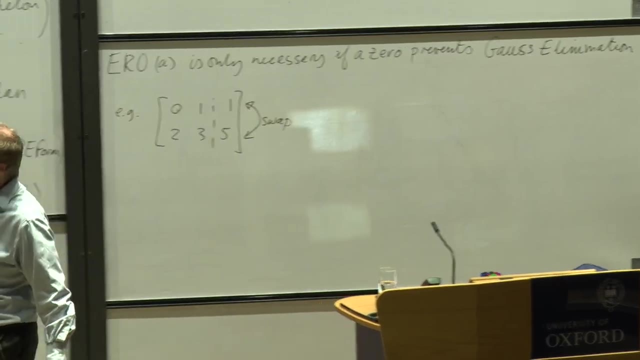 because there's no multiple of this equation. you can add to this one to make a zero in this position, But that's not a problem. So what do you do? You just swap. All right, That's EROA. Swap the two equations. 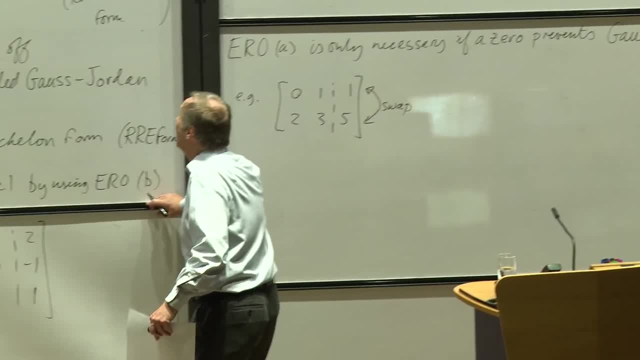 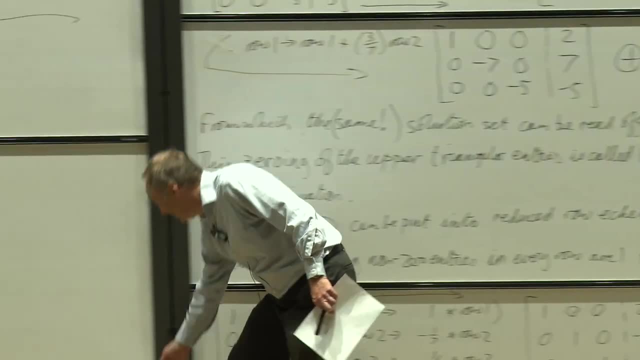 And then it's already in upper triangular form. I'm sorry I've been wrong here. This is: I should be a little bit careful with my nomenclature. It's not a nomenclature I'm going to use. I think, upper triangular, lower triangular. 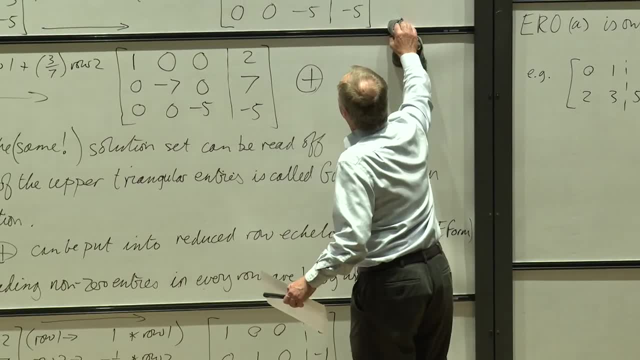 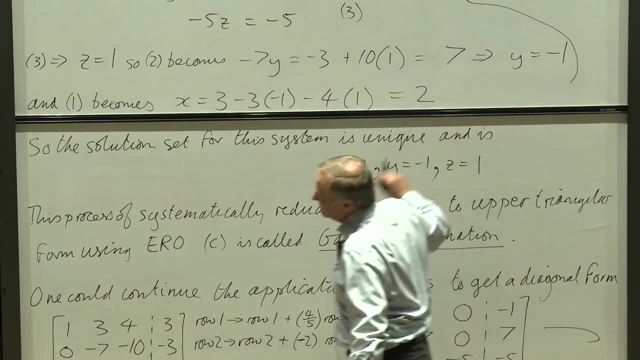 and so on is easier, But this isn't Rho echelon form. I'm sorry. The Rho echelon form is precisely this form right, The upper triangular form. Okay, This is Rho echelon form. This is Rho echelon form here. 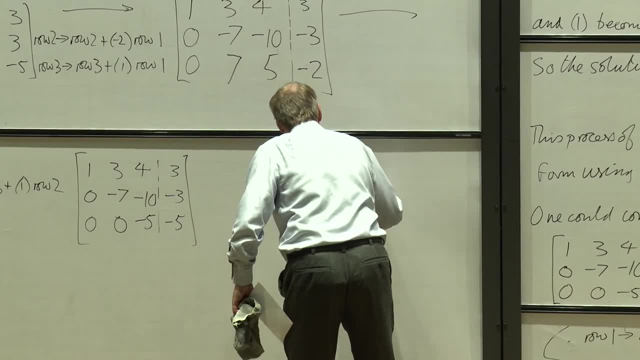 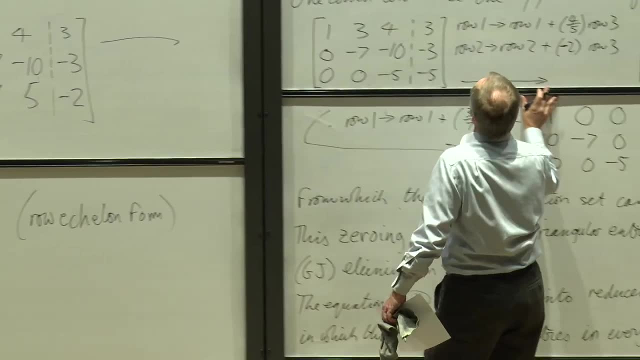 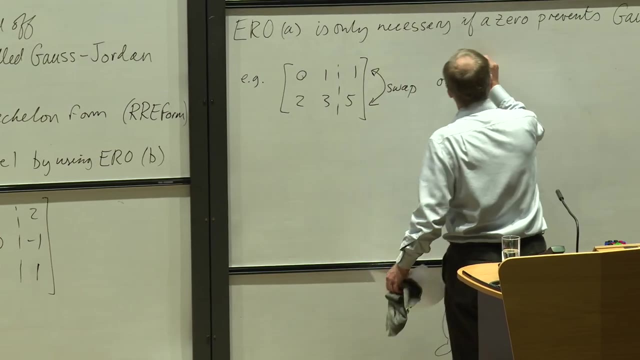 Oh There, Rho, echelon for triangular. Okay, Just to show you that you don't have to have such trivial examples as this. If you have, for example, minus 1,, 2, 1, and something doesn't really matter. 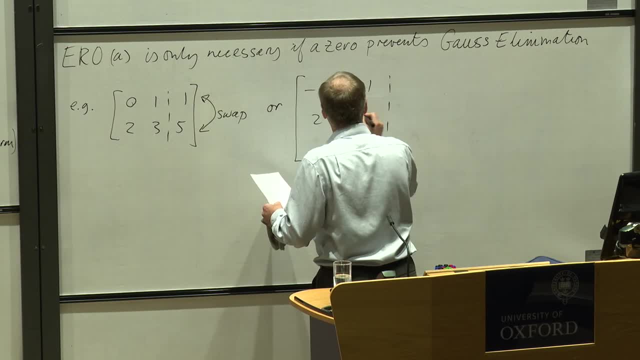 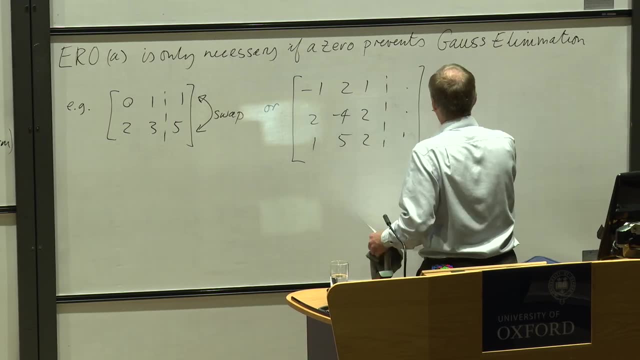 2 and 1.. 4, minus 4, and 2, and 1, and 5, and 2.. And it doesn't matter what you have here. Okay, This will then go to, if you do, Gauss elimination. 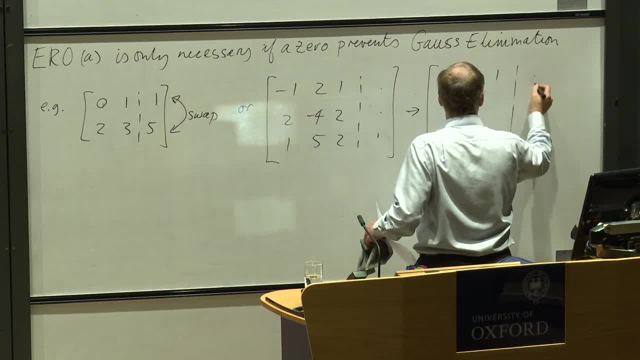 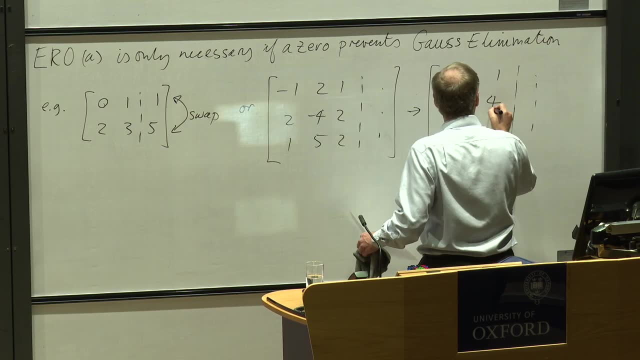 you'll go minus 1,, 2,, 1,, something on the right-hand side, And then it will go to well, 0 and 0, and in this case I think, 4. And then 1 and 5.. 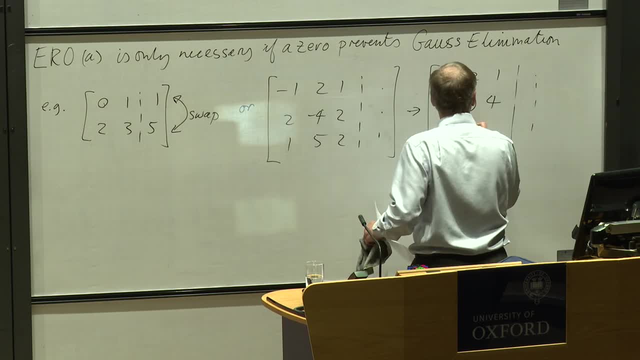 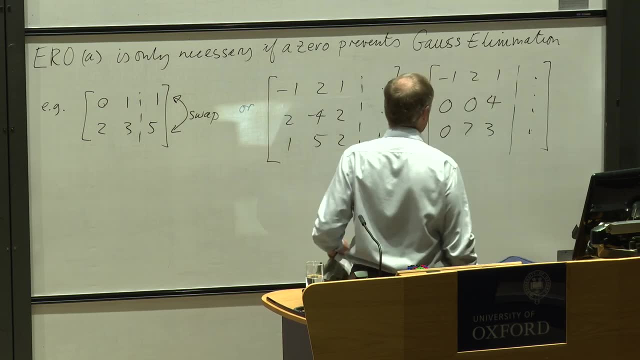 0 and- sorry, elimination here- 0. And 7, and 3, and something on the right-hand side here. It doesn't matter what these numbers are here. And again, I can't do, if I do, Gauss elimination there. 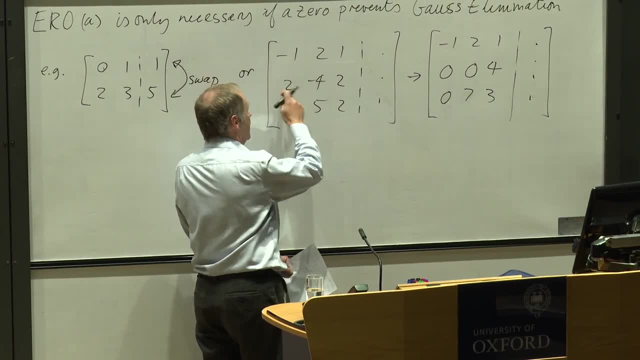 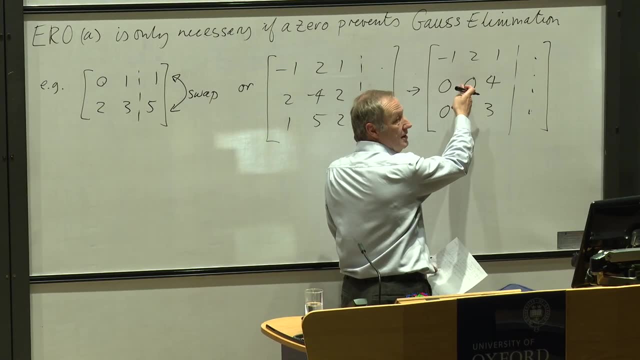 that's exactly what I get, Because, unfortunately, add 2 to that to that and you add 2 of that to that, you get two 0s. And now I can't do Gauss elimination because I can't take a multiple of this row to add. 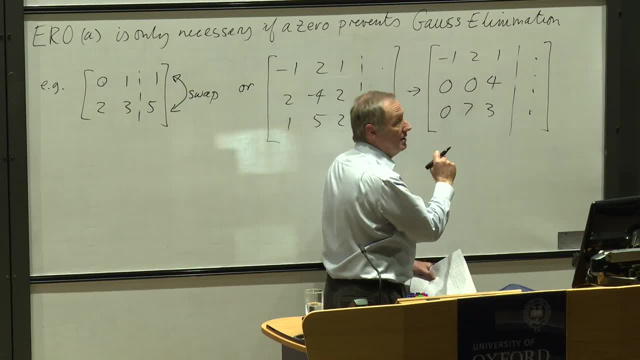 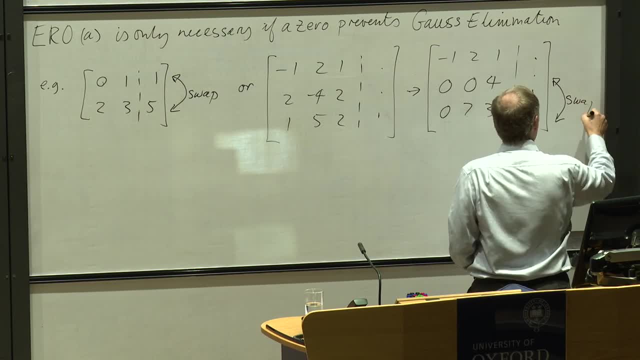 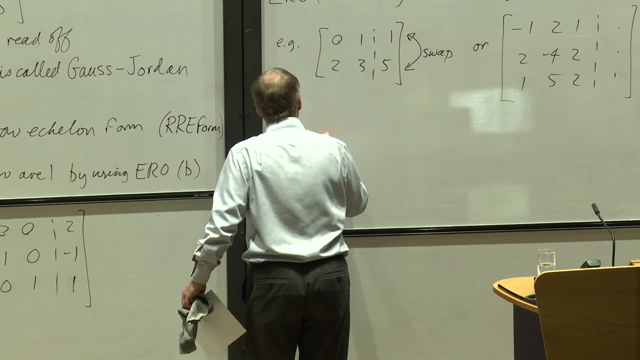 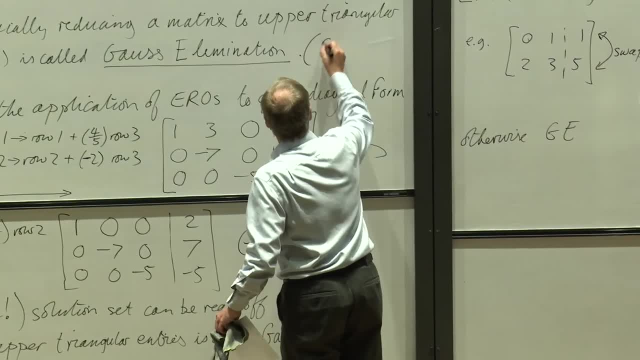 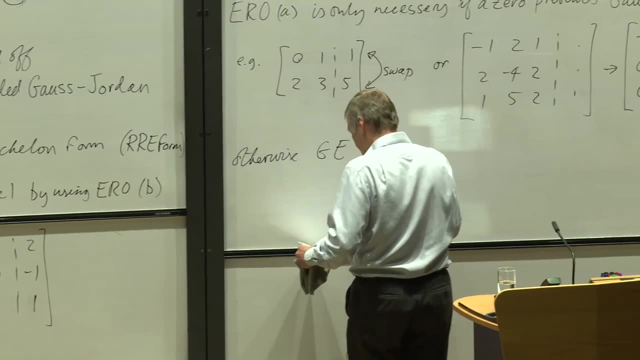 that's what this is right. Gauss elimination. I shall call it GE And GJ, which I have said: Gauss Jordan. Okay, So this is the arrow. So this is the arrow, So this is the arrow. 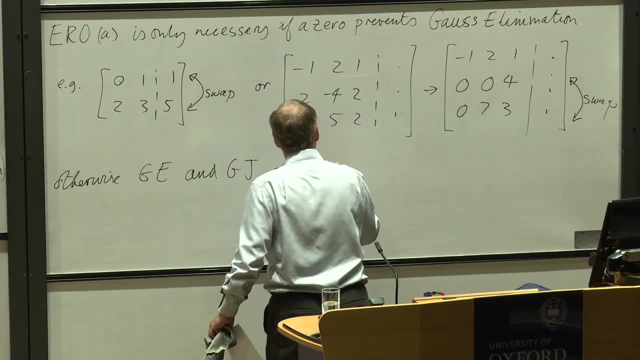 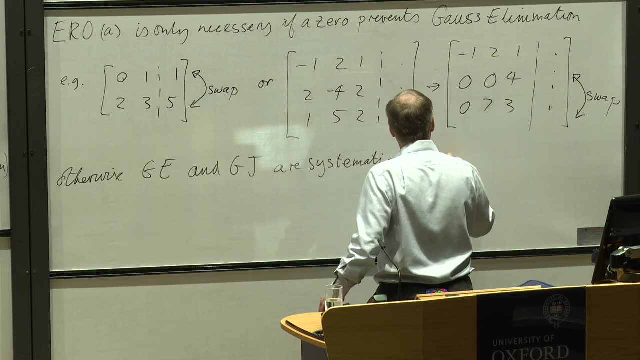 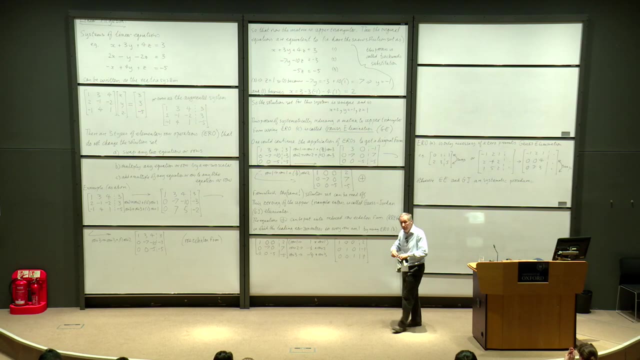 Okay, Our systematic procedures. In other words, I can give them to a machine or a monkey to do these calculations. Okay, All right, All right. So I've done that, All right, All right, just done that example so far, and that's sort of like what you've already seen. I 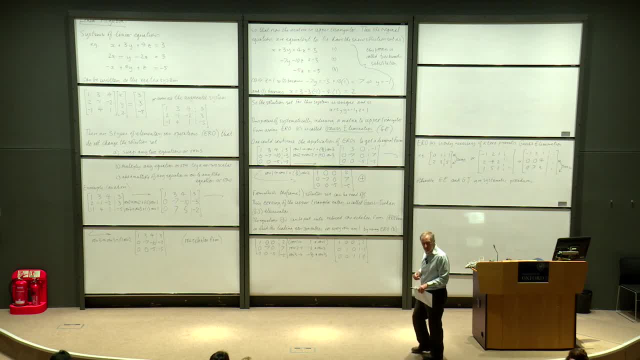 guess perhaps some of you- I'm just solving a system of equations and I'm being a little bit pedantic about it, and I'm not going to apologize for being a little pedantic. that is, you, as humans, try to use your intuition and your to make your life a little easier. I am trying to do something that's entirely. 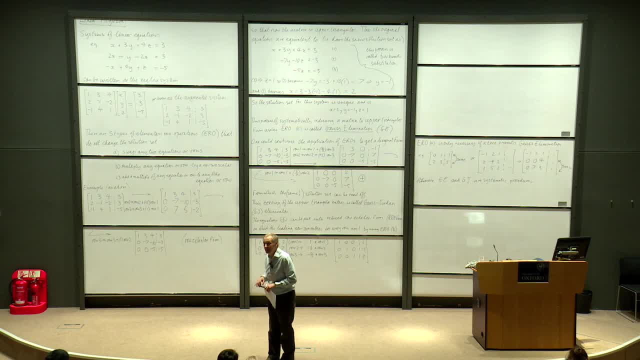 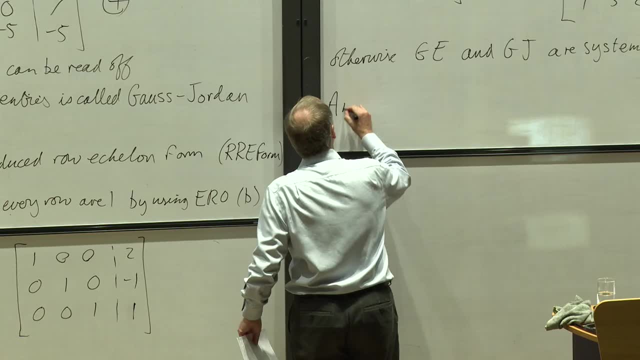 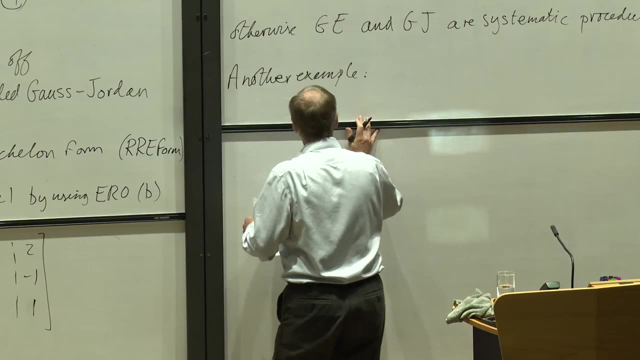 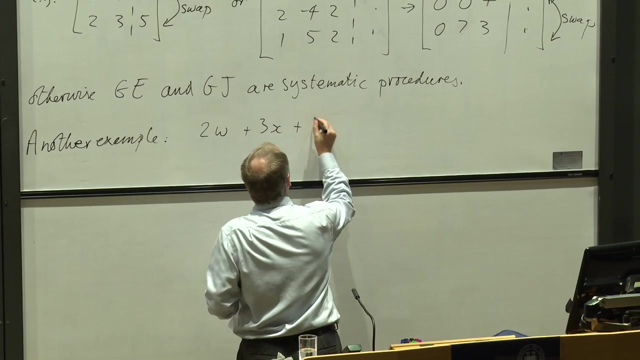 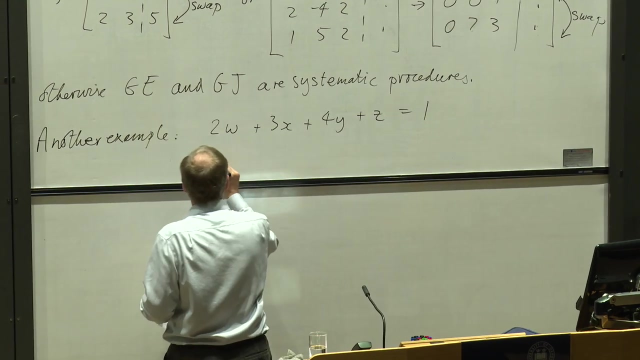 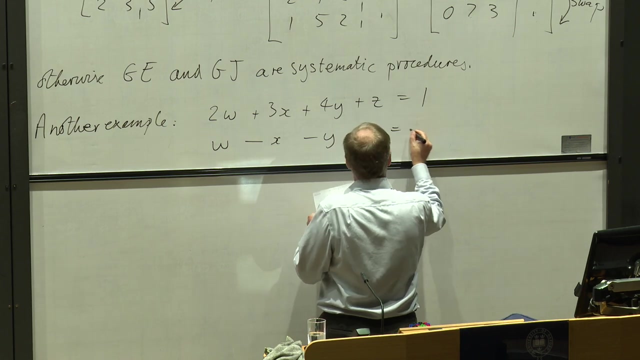 systematic. all right, okay. here's another example. okay, so this one is going to be: 2w plus 3x plus 4y plus z is equal to 1, and w minus x minus y plus z is equal to 1, and oh and I'm. 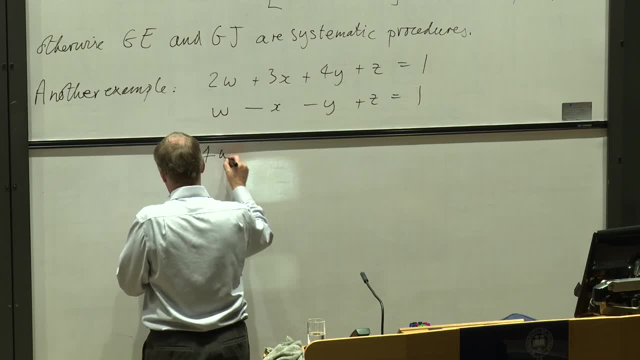 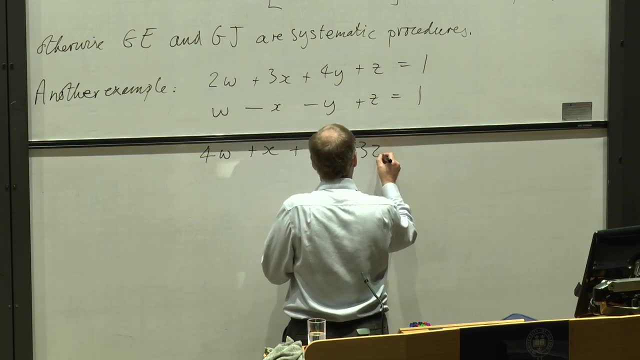 sorry, I'm going on to the next board. that's fine. it's still three equations: 4w plus x plus 2y plus 3z is equal to- and I'm going to put in a parameter here, let's call it: x plus 2y plus 3z is equal to- and I'm going to put in a parameter here, let's call it. 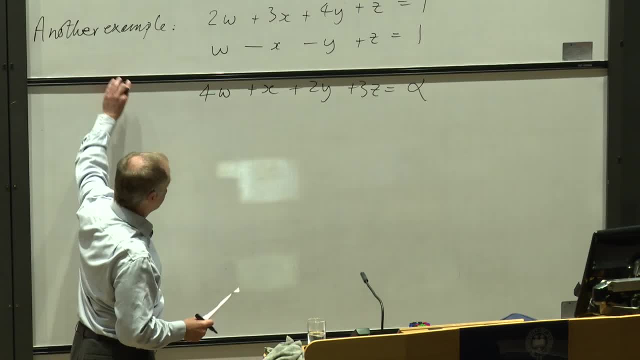 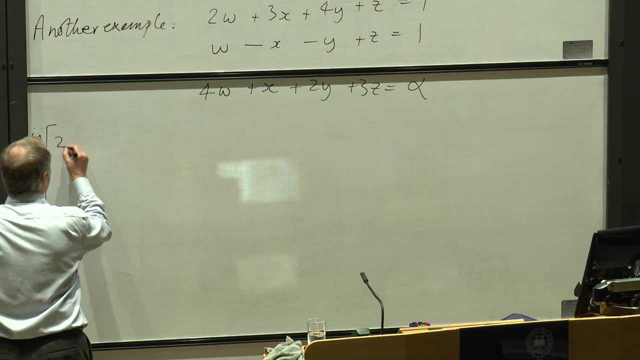 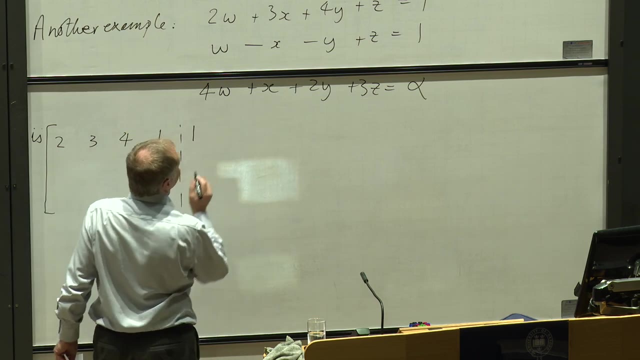 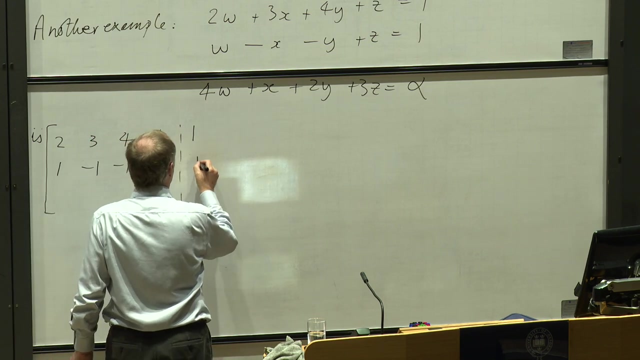 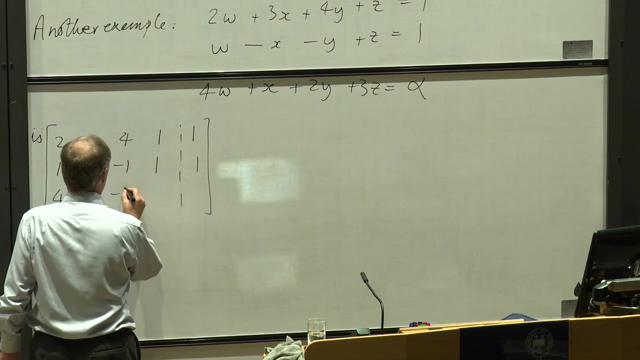 alpha. okay, so now we can write this as an augmented system quite easily. this is: two, three, four, one partition one and 1 minus 1 minus 1, 1 partition 1 and 4 minus Minus 1, minus 1, 1.. 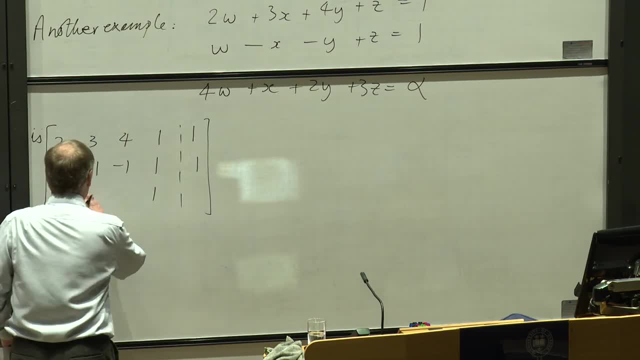 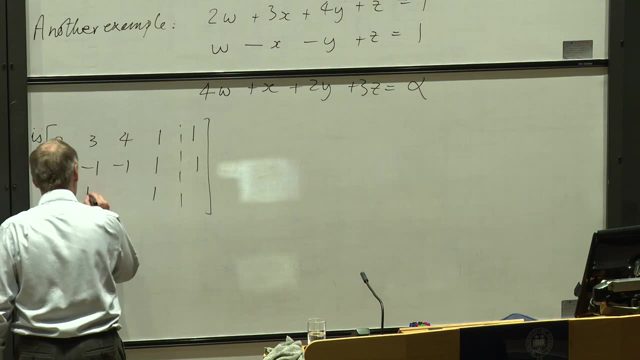 Oh no, I'm writing down the same equation. This is the problem of being too close to the board. You can see it, I can hardly see the board 4.. So this equation I'm writing down, Plus 1, right. 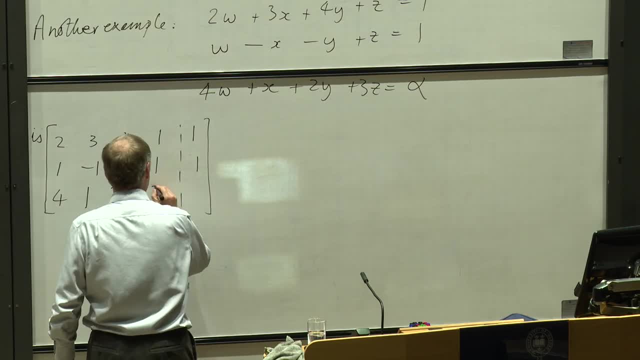 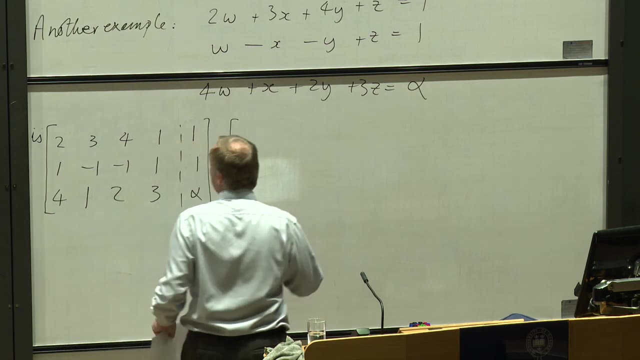 Plus 2.. And plus 3.. That's this one here, And then there's an alpha down there. OK, So here's another augmented system for this set of equations, And I'm now going to do Gauss elimination. OK, And Gauss elimination is going to not change the first one. 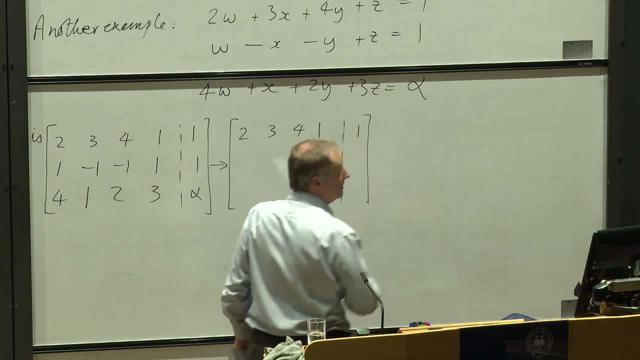 as before, And then the second one. I'm going to take a half of the first equation from this equation to make 0 here, right, And so on, And that will give me 0. And I'm just going to write down the numbers. 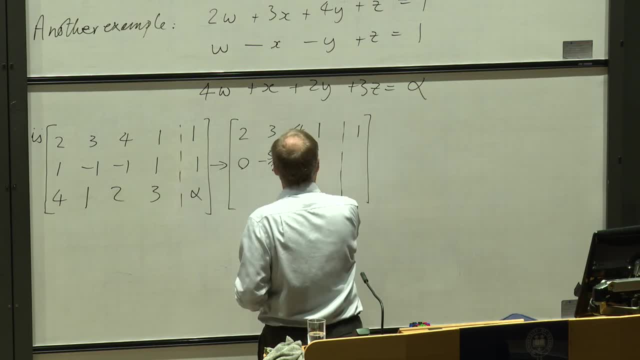 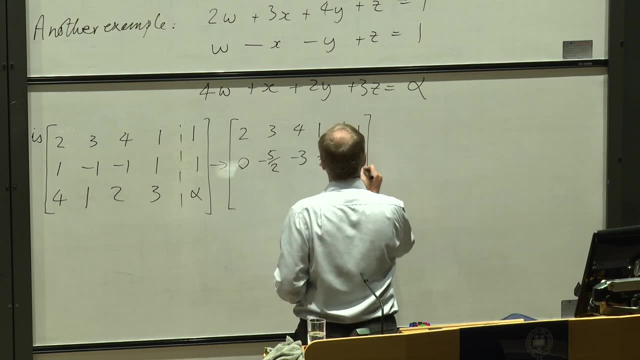 And you can do the arithmetic And you can tell me if these numbers are correct. I believe they are. This is a half And then I'm going to take twice that row from that row And I'm going to get a 0 there. 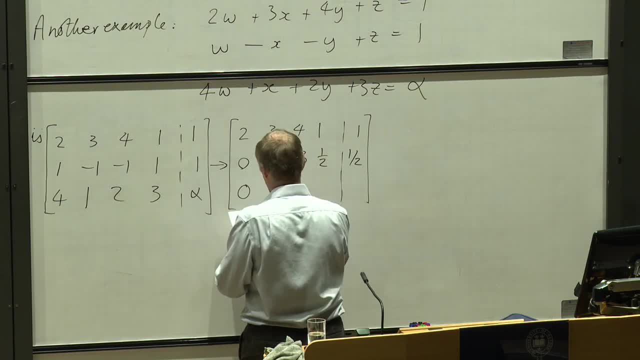 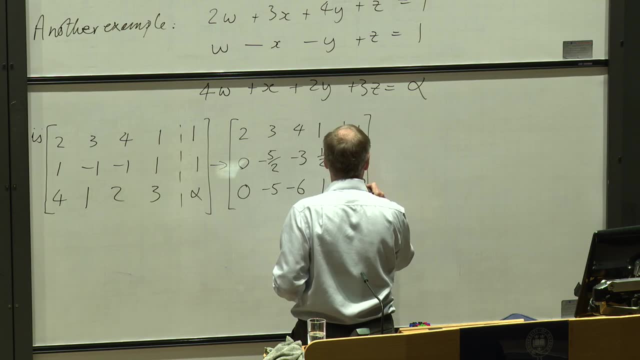 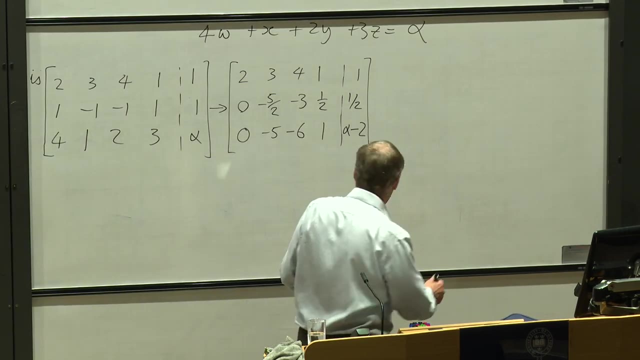 And then I get these numbers. I think I get 0, minus 5, minus 6,, 1, and alpha minus 2.. That's the first stage of Gauss elimination, And then I'm going to do the next stage. 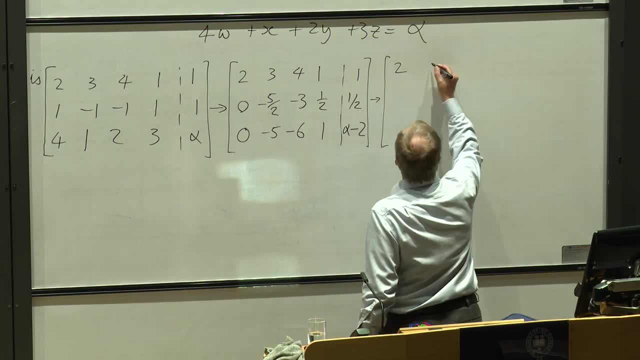 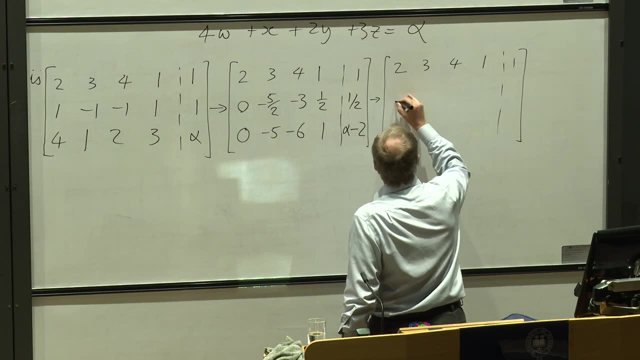 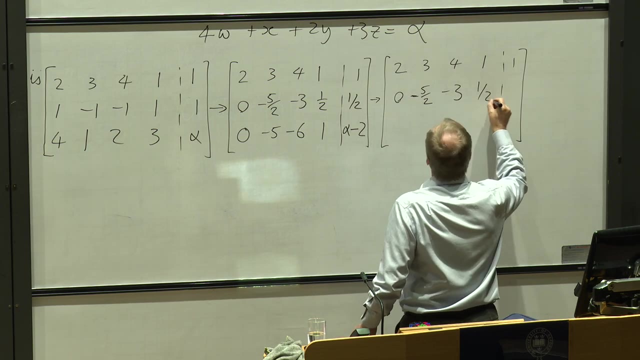 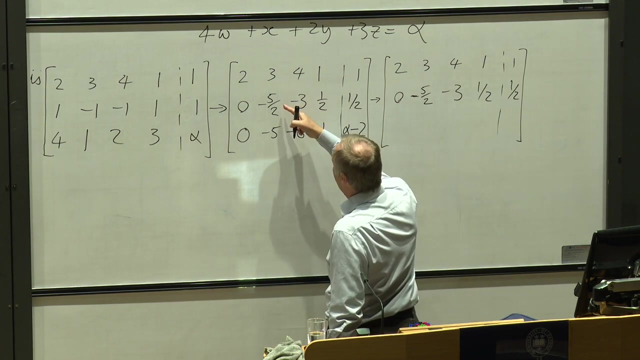 And the next stage of Gauss elimination is not going to change the first equation Nor the second equation, But the final equation is going to become: I've got to add twice that to that And I'm going to get 0, 0, because 0 is plus 0 is 0. 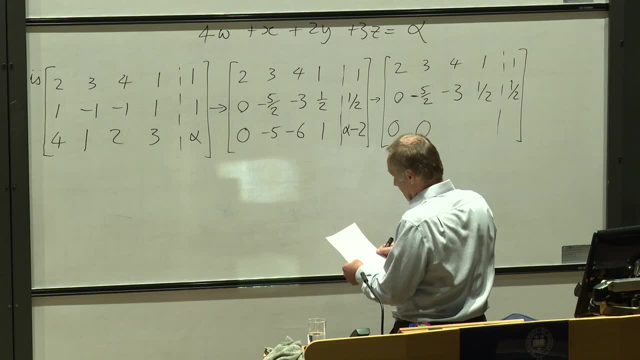 And if I add twice that to that? OK, have I got this right? Yes, I think I've got this right. It looks like that must also be a 0.. OK, Sorry, I've got to subtract twice that, Minus 2 times that and add to that. 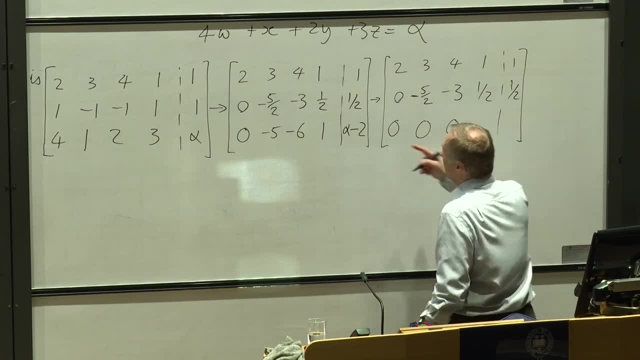 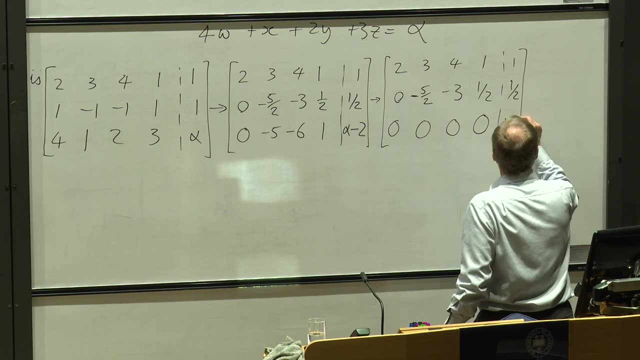 Minus 2 times that and add to that. And the last equation is: oh, minus 2 times that and add to that is also 0. And then what do I get? in the right, I get alpha minus 3.. So I've just done Gauss elimination. 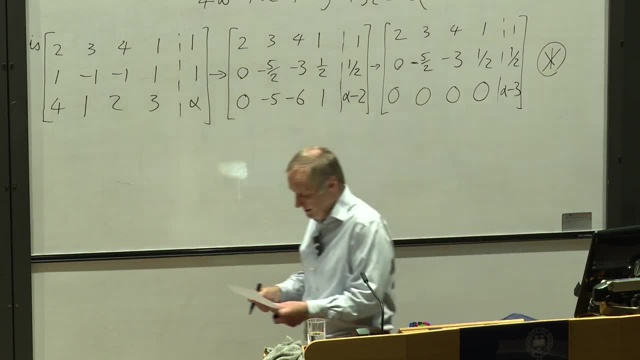 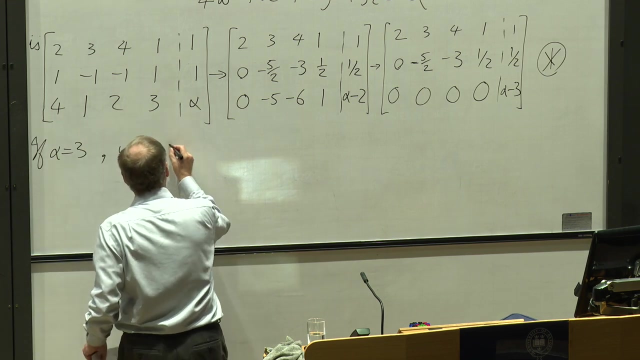 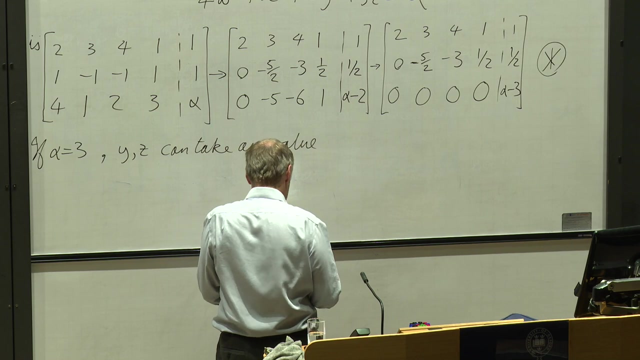 And these are my equations for today, which I will call star OK. So, first of all, if alpha is equal to 3, OK. then y and z, OK, can take any value. So I'm going to parameterize, OK. 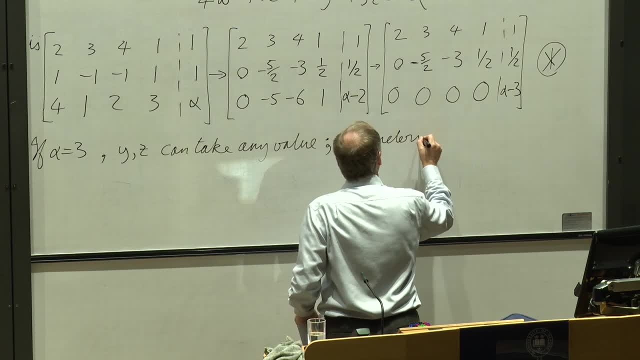 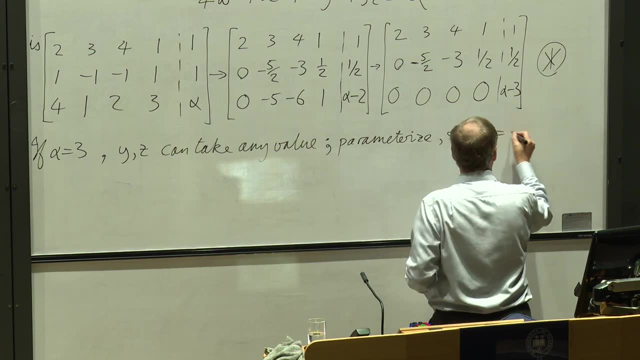 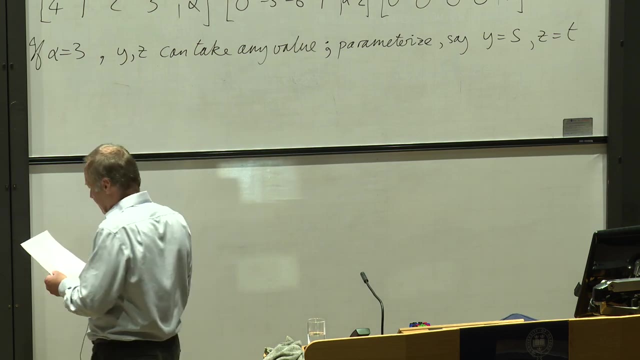 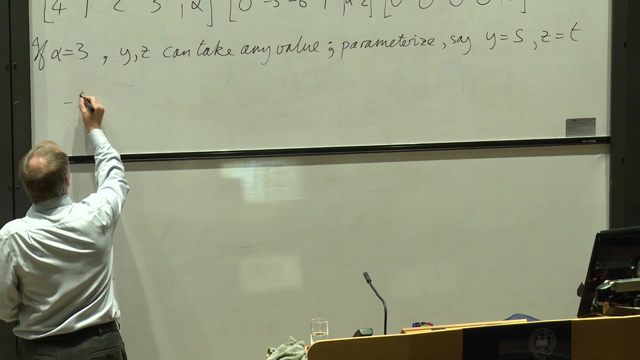 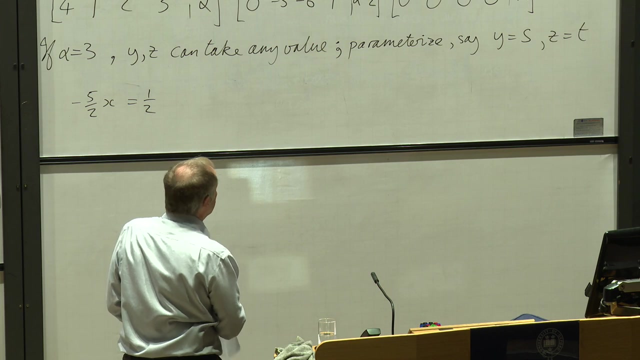 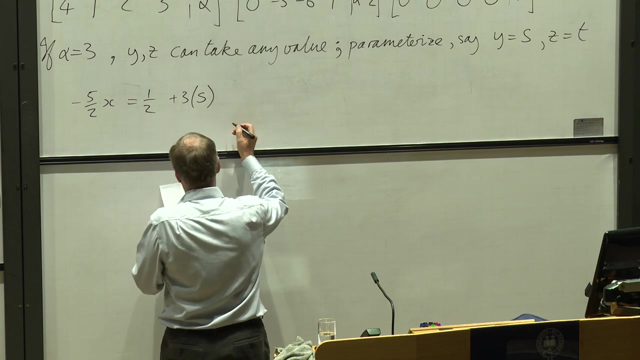 I'm going to parameterize. I'm going to say: put: y is equal to s and z is equal to t. OK, And then? OK, what do I get? I get that minus 5 over 2 lots of x is equal to a half, plus 3 lots of s, minus a half lot of t. 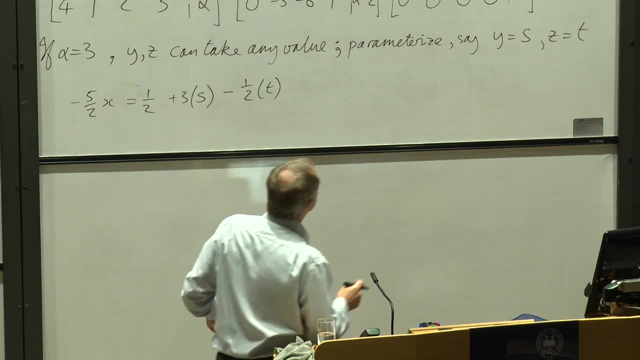 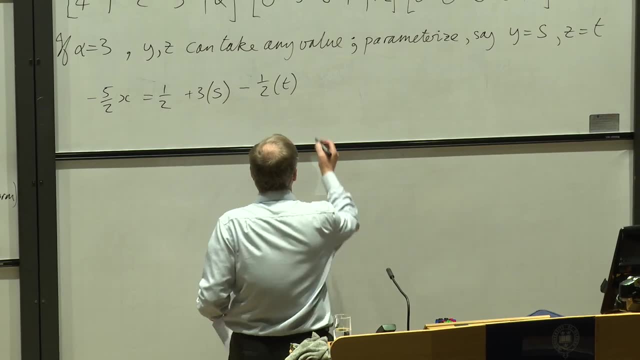 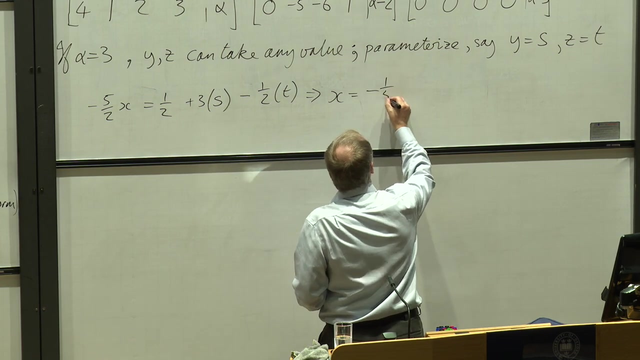 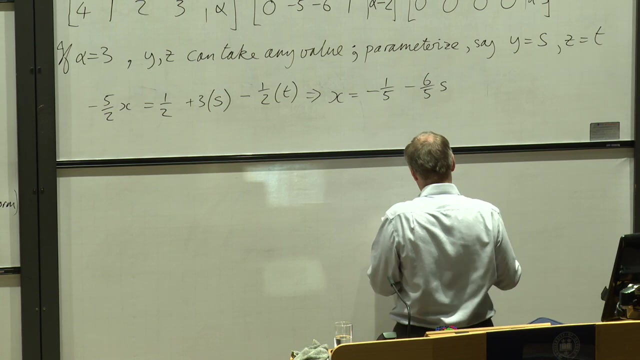 Minus 3? No, it's plus 3, I think There's a minus sign here. OK, And so this tells me that. So this tells me that x is equal to minus a fifth, minus 6 over 5. lots of s plus 1 over 5, lots of t. 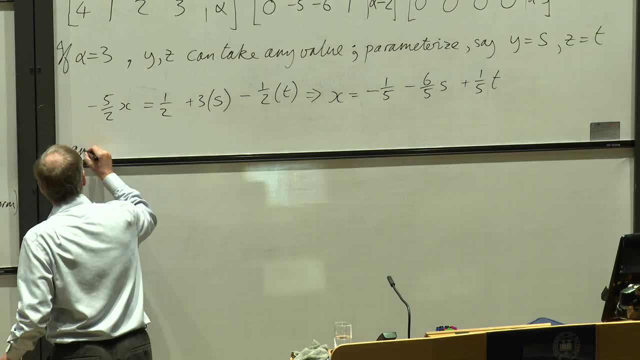 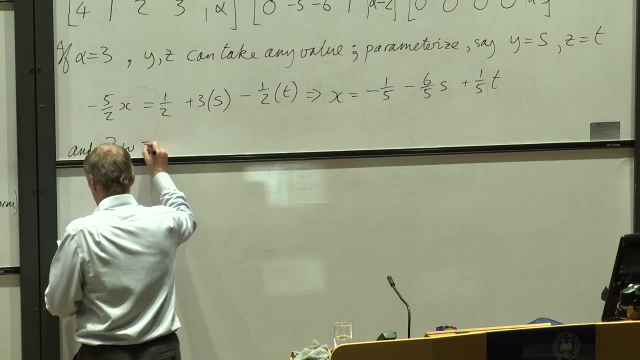 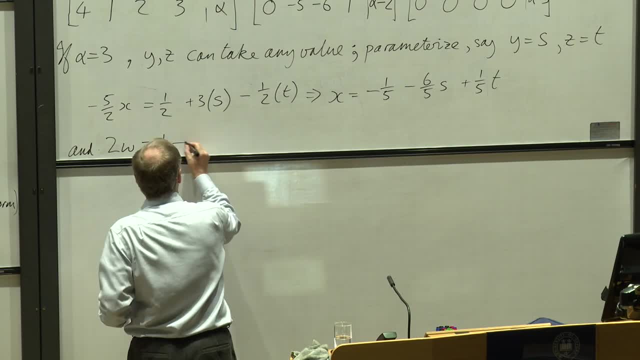 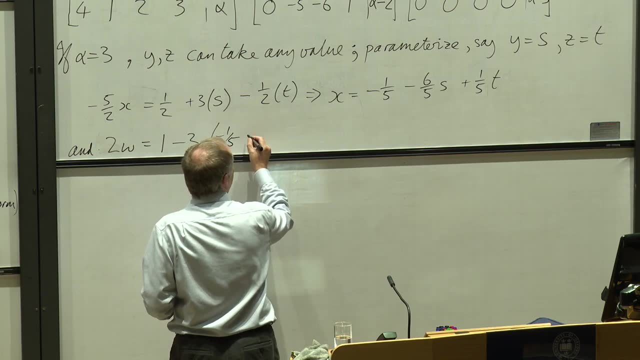 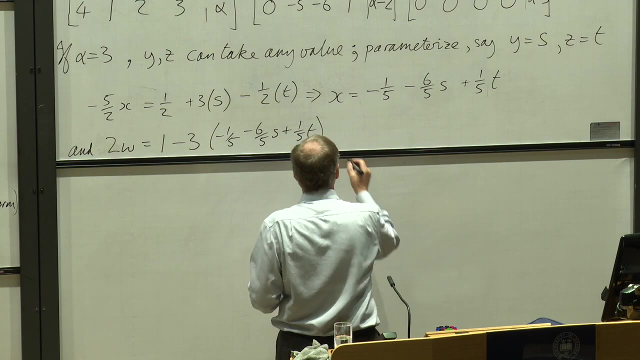 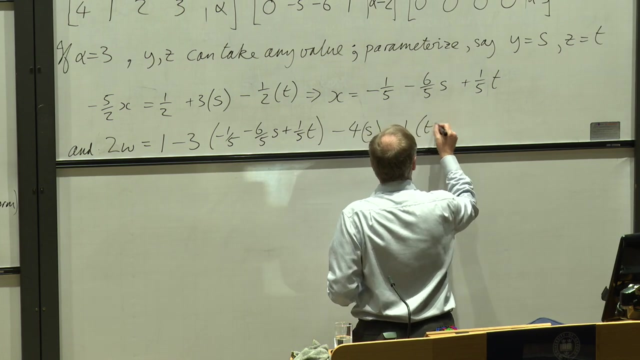 2w is equal to 2w is equal to 1 minus 3- lots of x. And now I know what x is. x is equal to minus 1 over 5, minus 6 over 5. s plus 1 over 5. t minus 4. lots of s, minus 1, lot of t. 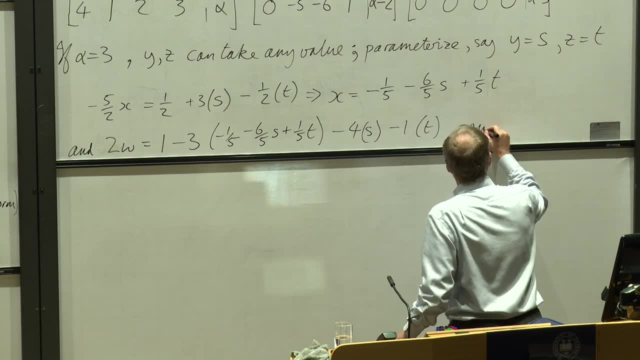 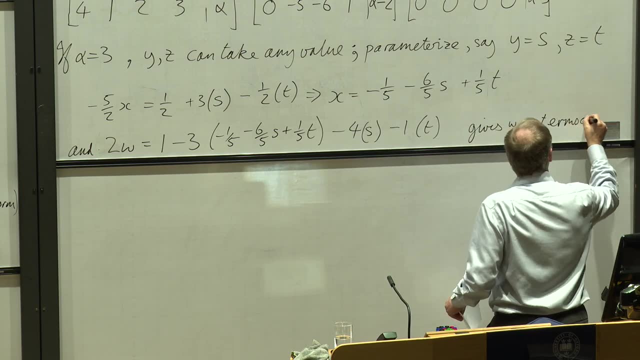 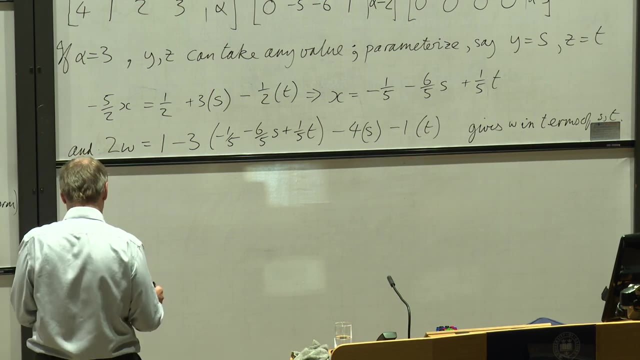 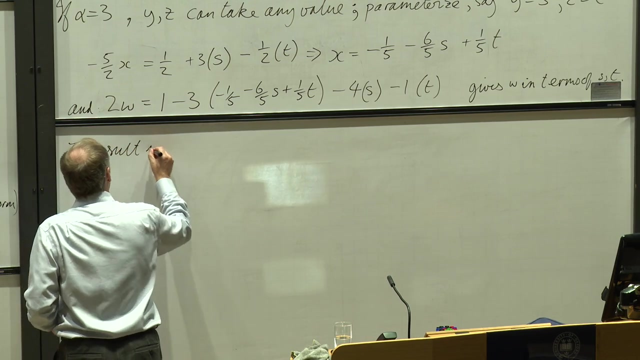 OK, And so this gives. This gives w in terms of s and t, And you can simplify it, but it's clearly giving me w in terms of s and t. OK, So now I can write down the result. The result is that w. 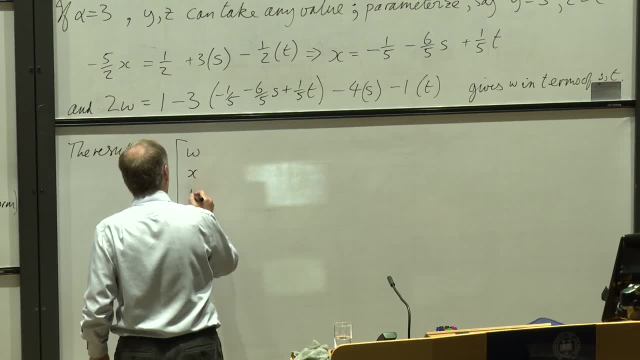 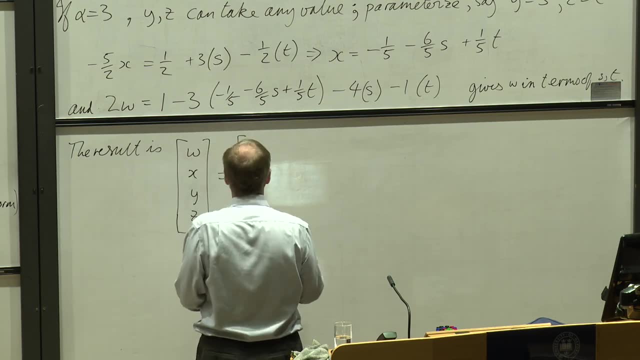 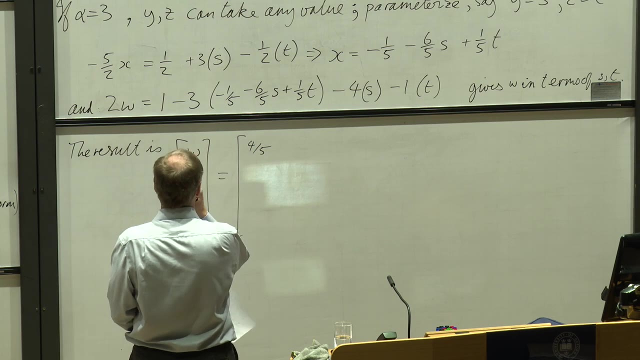 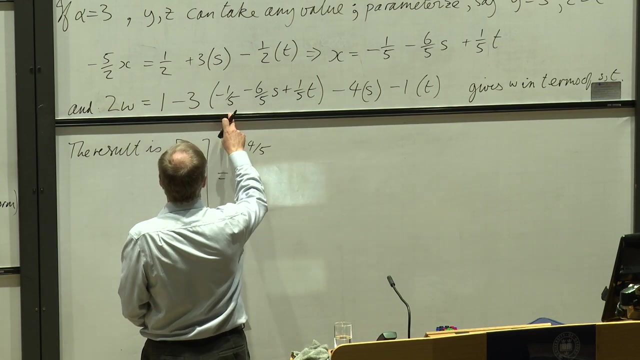 I'm not sure I've got enough space here. w and x and y And z is equal to, And then it looks like it's 4 fifths. OK, So this is 1 plus 3 fifths, That's 8 fifths. 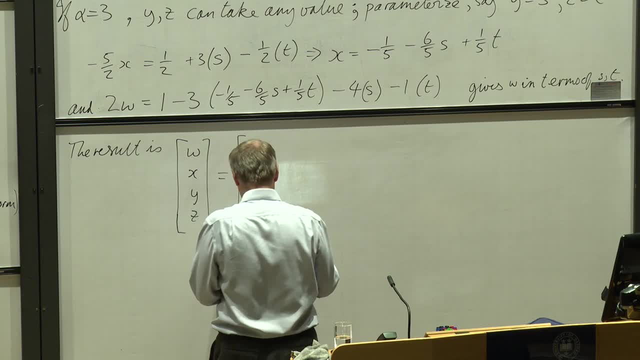 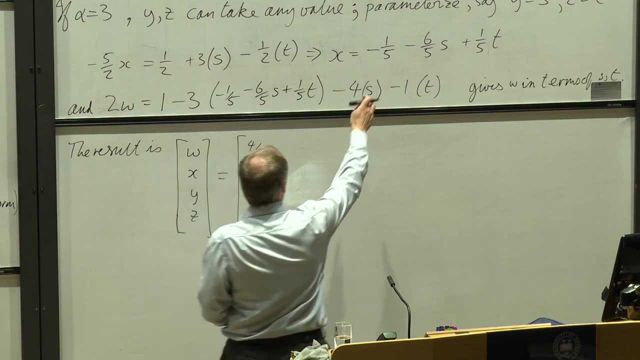 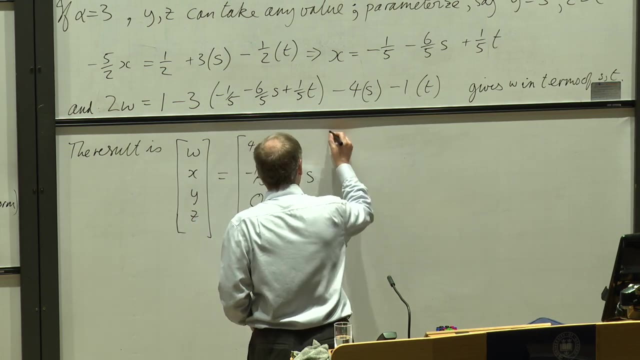 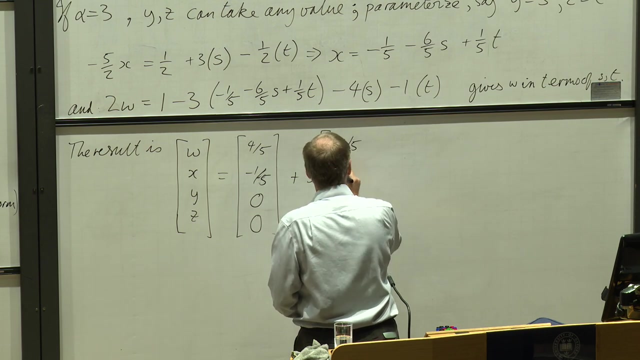 And you've got to divide by 2.. And minus That's a fifth- Oh, That's this guy here- And 0 and 0.. And 0 plus s times the vector minus 11 over 5, minus 6 over 5, and 1 and 0.. 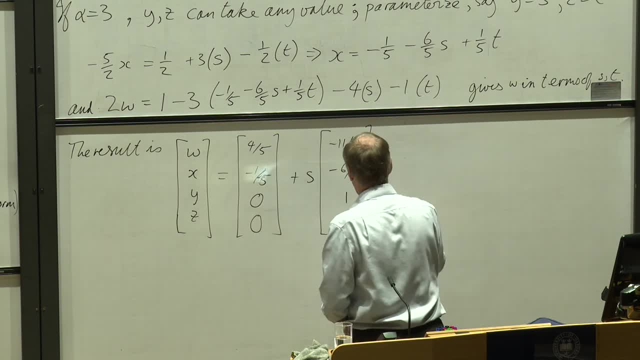 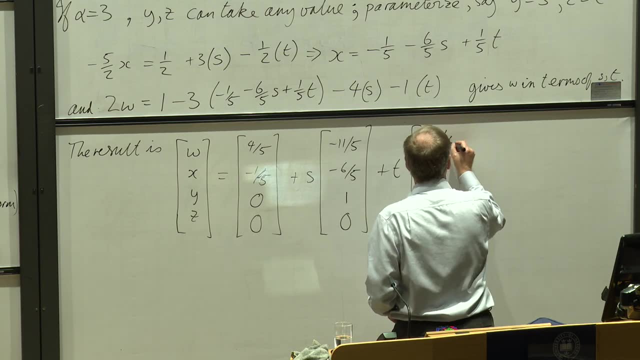 So this just says y is equal to s in this state, Plus t, And then the appropriate numbers are minus 13 over 10.. You can check these things for yourself. You can't do them in your head, like I can't at the moment. 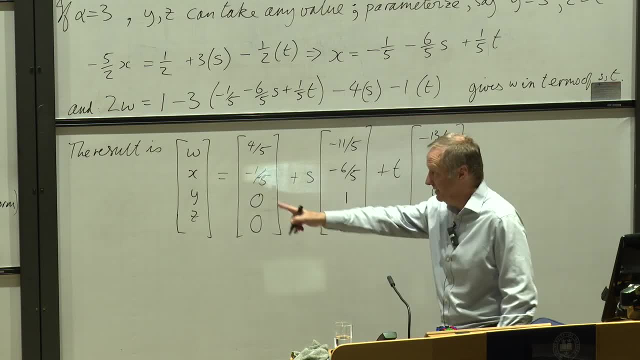 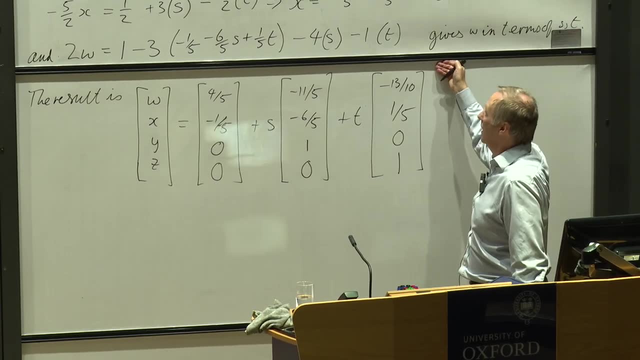 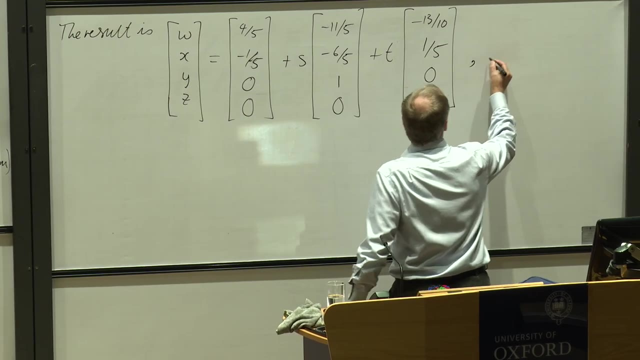 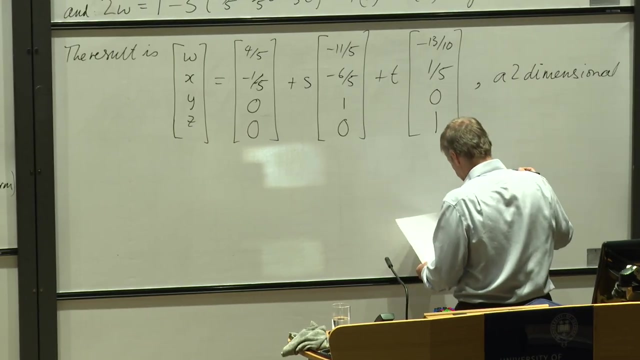 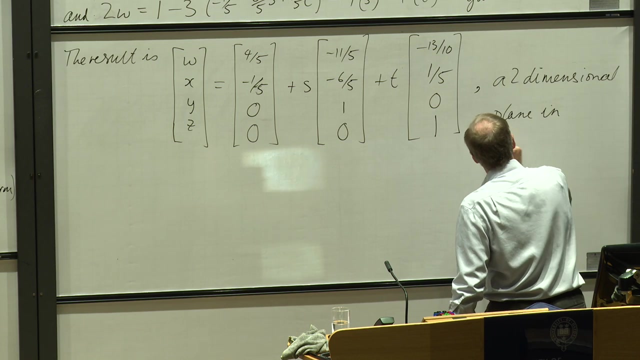 And 0 and 1.. So this last equation says z is equal to t. OK, So this is A two dimensional Plan in 4 dimensional real space. You want to think of geometrically what this point means? I'm in 4 dimensional space. 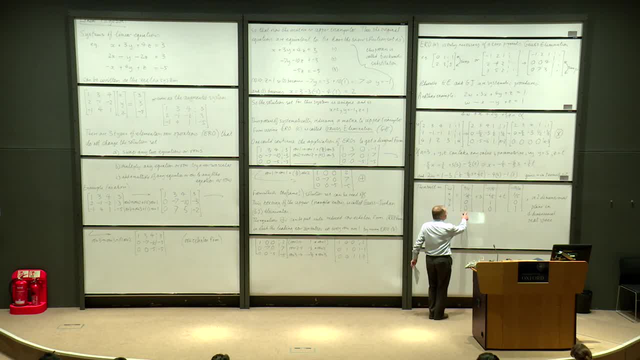 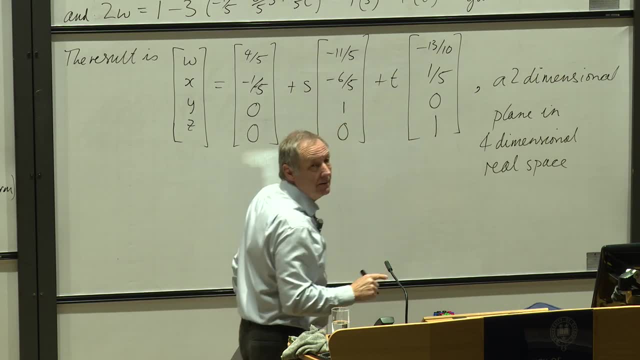 And I can go to a particular point. And I can go to a particular point and then I have to go any distance in another direction plus any distance in another direction. so I go to a point and I can go that way or that way, so that fills out a plane for me. 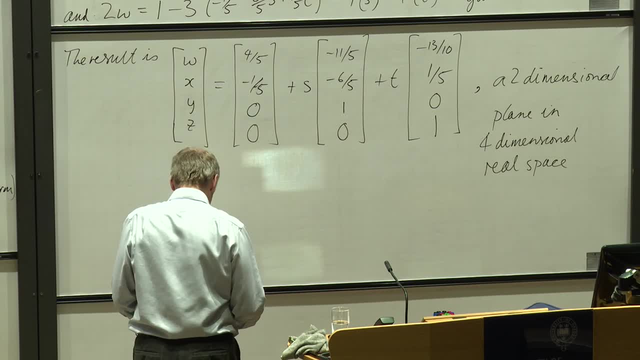 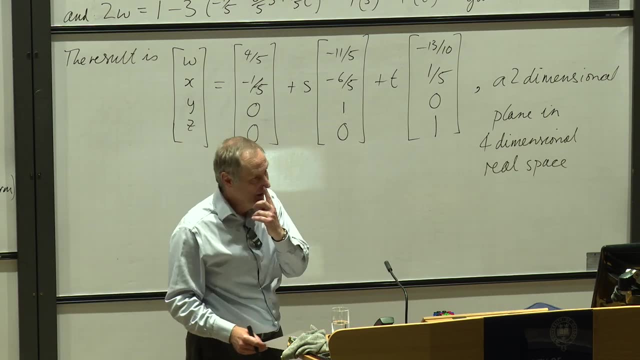 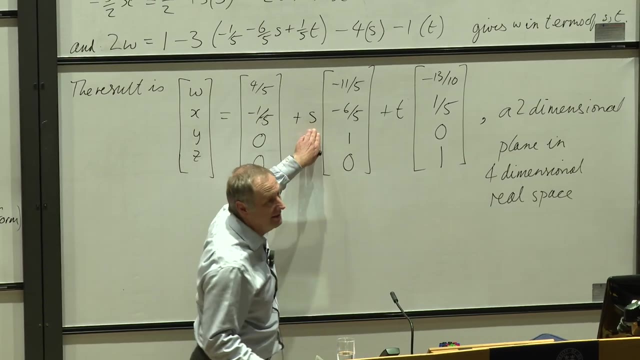 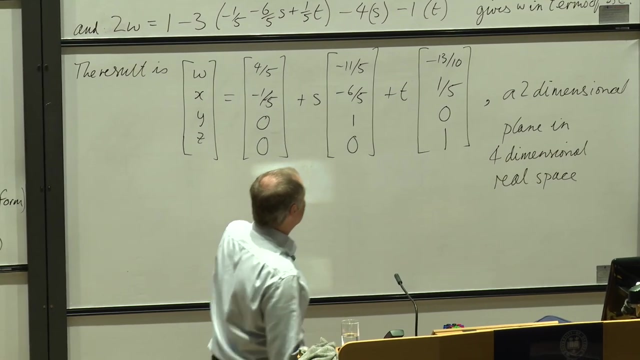 okay, so that's what happens. clearly, my parameterization by s and t is sort of unnecessary, but explicitly done here to make it a little bit easier for you to see it it does. I could clearly have called this y and I could have called this z. that's exactly what they are, right. 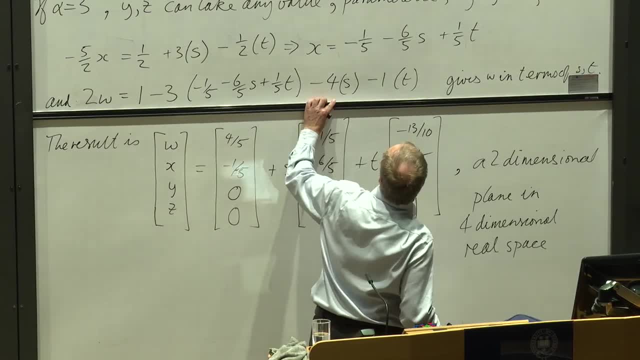 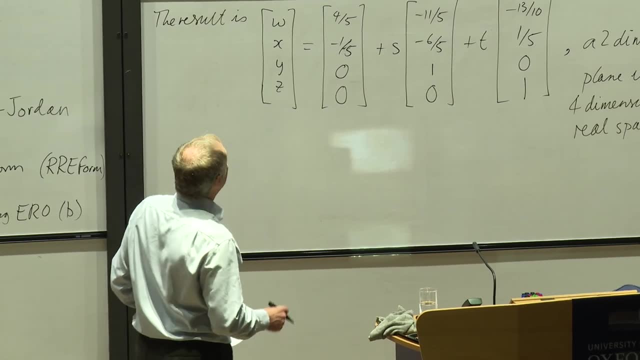 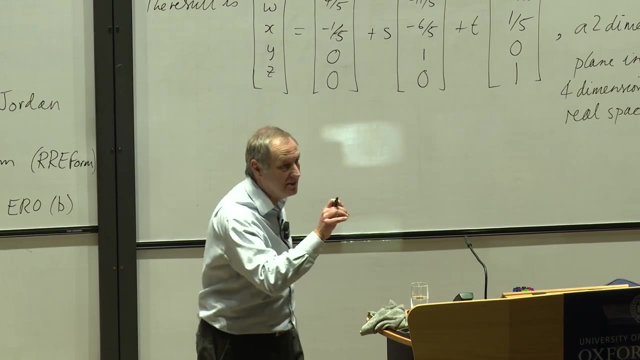 I just introduced things that you might think would be parameters. now I'm going to carry on here, in danger of breaking my rule of making sure you guys can see, because I want you to see. this follows on. I'm not you. if I jump over there, you're going to think: oh, there's a discontinuity, and I don't want that to. 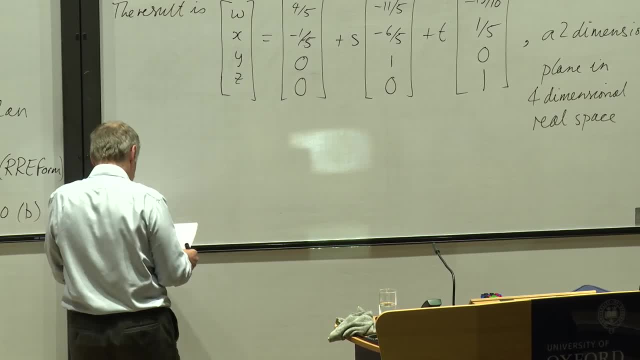 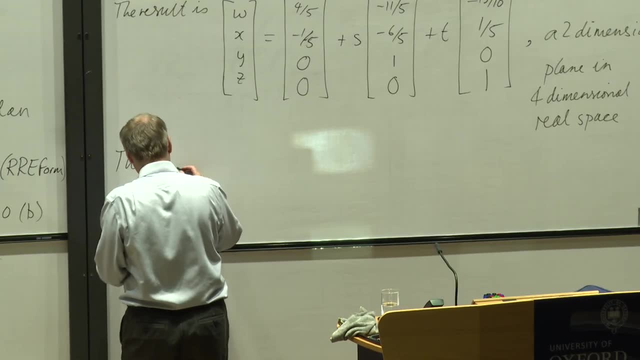 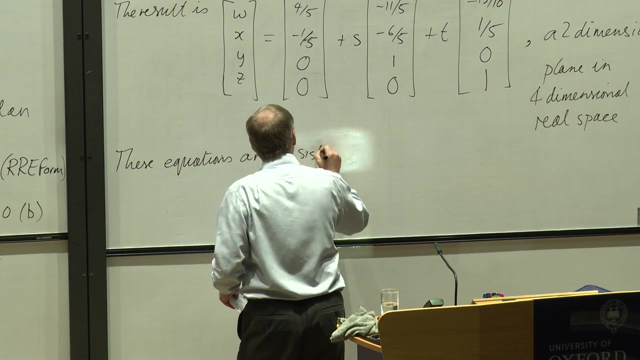 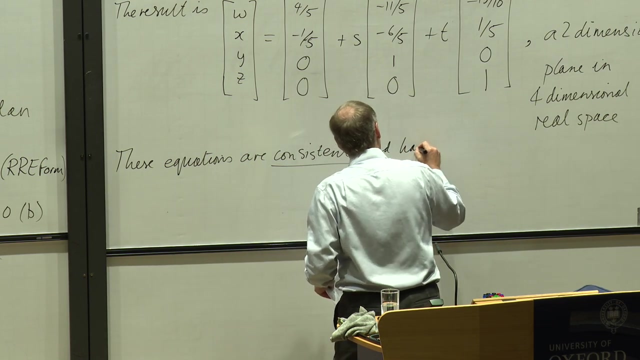 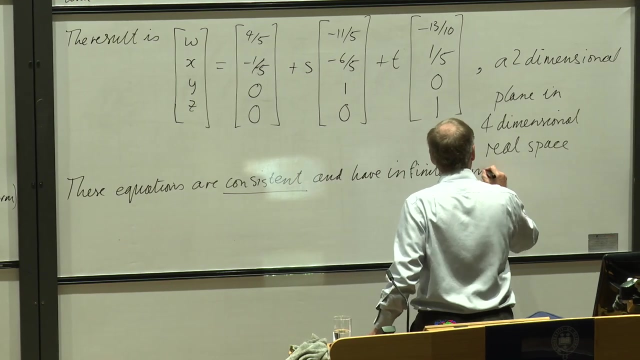 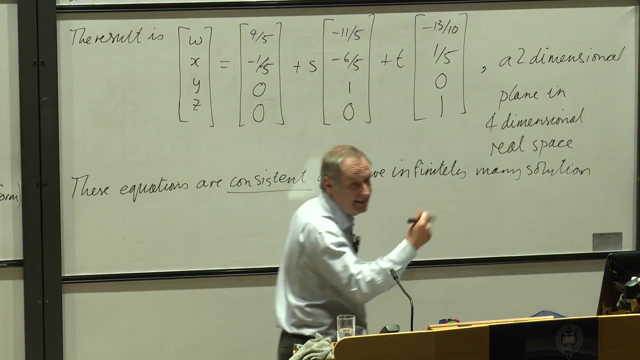 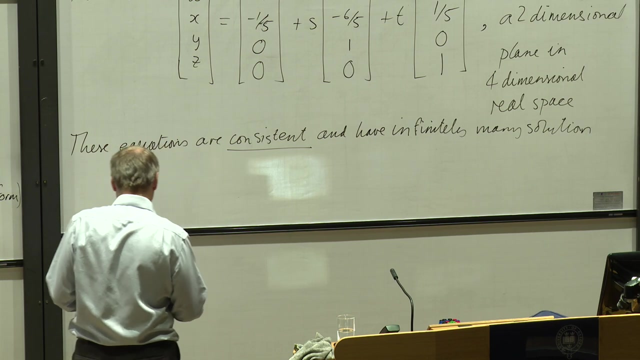 happen. so the question is if okay, okay. so first of all, I should say these equations are consistent, okay, and have infinitely many solutions. some people would say doubly infinite, because there's two parameters, s and t. you can choose, but certainly infinite um. on the other hand, if 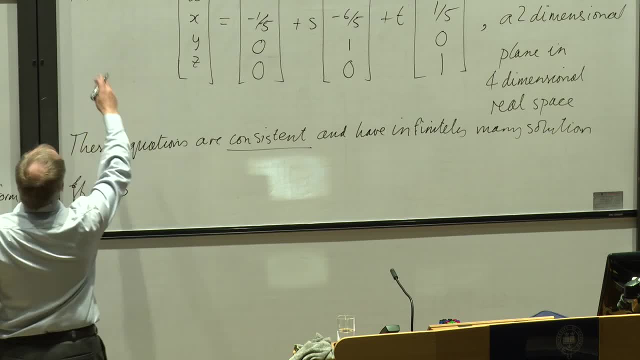 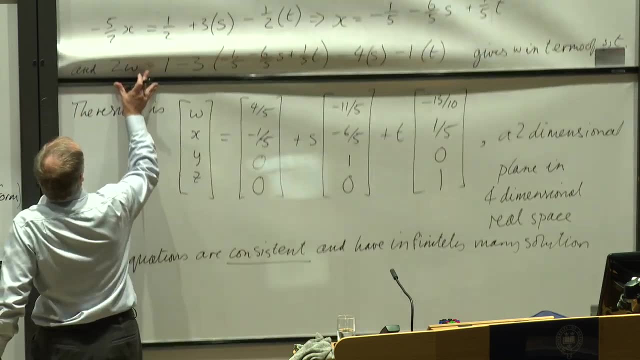 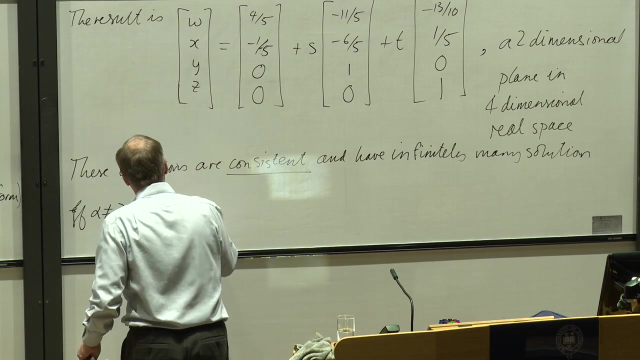 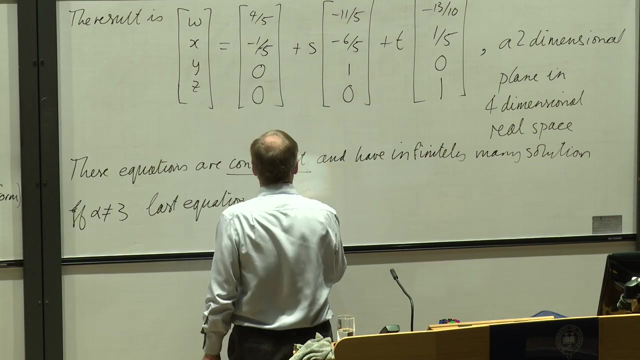 alpha is not equal to two. remember, all of this is predicated on. if alpha was 3,, then all this follows, But if alpha is not 3,, okay, the last equation is: well, take it from equation star. there it's. 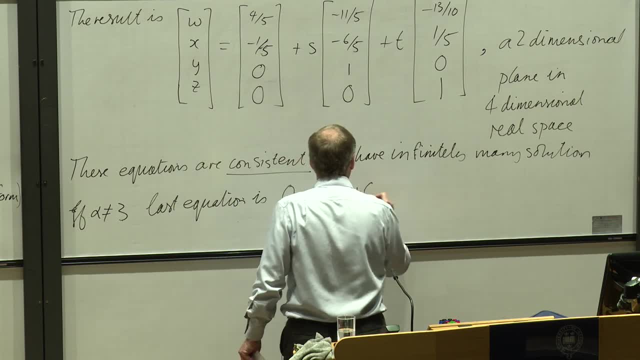 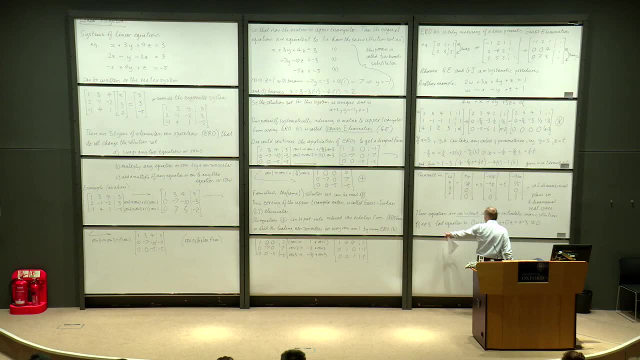 0 times w plus 0 times x plus 0 times y plus 0 times z is equal to alpha minus 3, and alpha minus 3 is then not 0 if alpha is not 3.. And what's the solution to that? 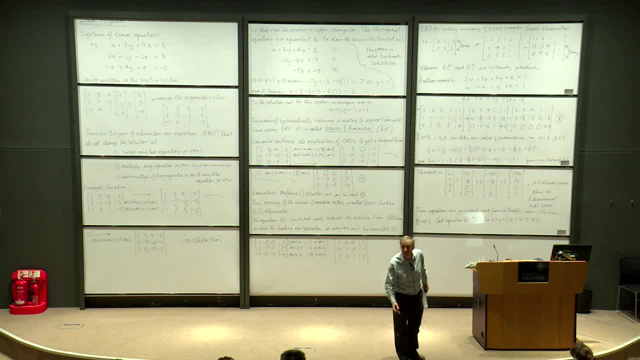 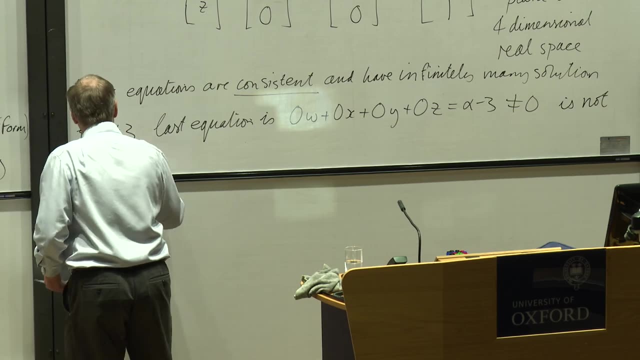 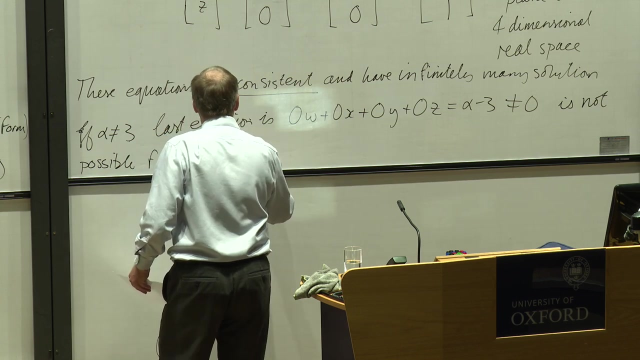 Sorry, There isn't one, There is no solution, Okay, And so this is not possible for any choice of the variables. So this is not possible if alpha is not 3.. For any x, oh, sorry, w, x, y. 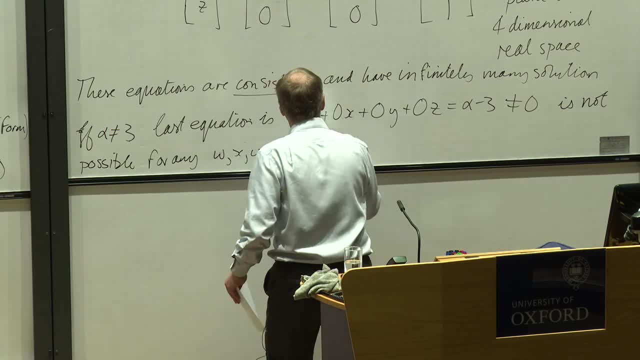 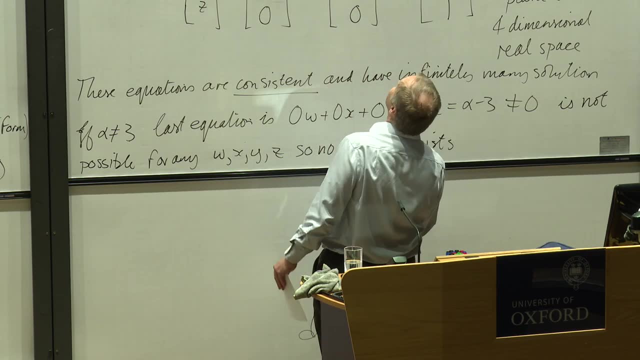 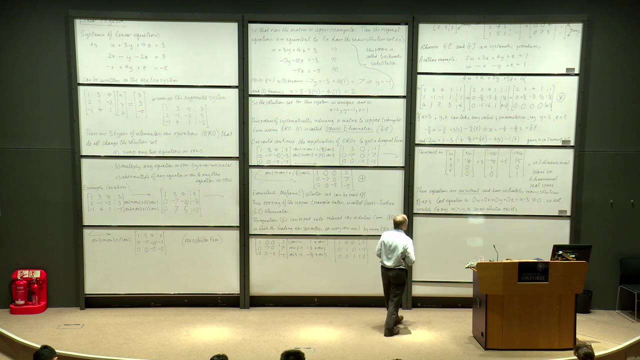 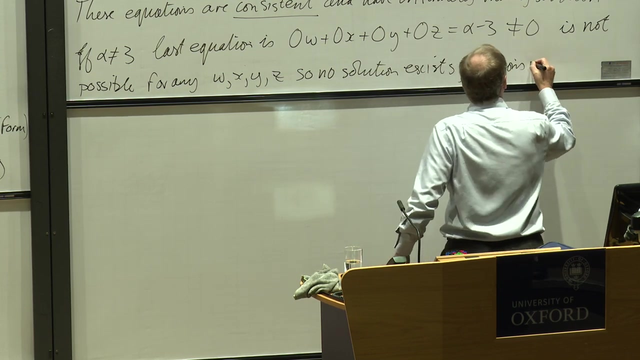 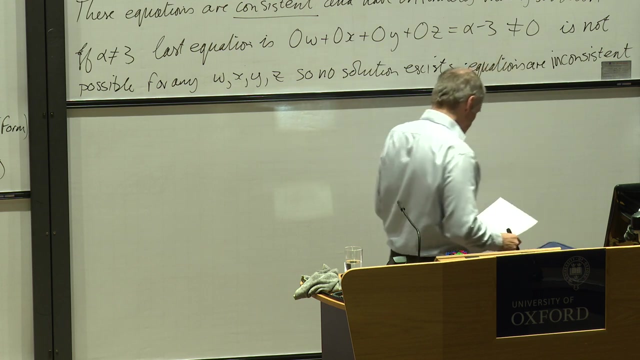 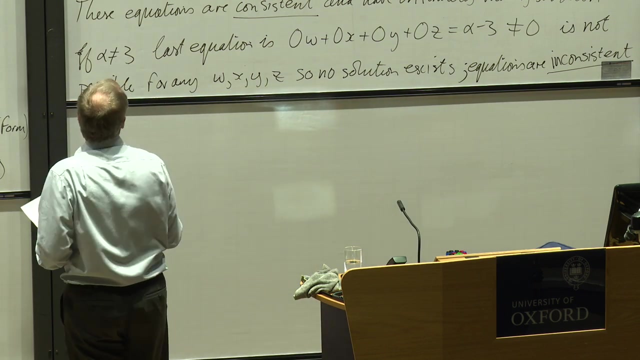 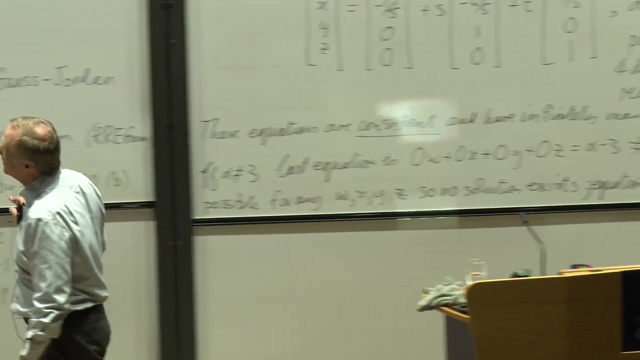 and z, so no solution exists. In other words, the solution set is the anti-set. Okay, These equations are inconsistent. These equations are inconsistent. I'm now going to make some notes. It is the same example, but I do want to observe my rule. 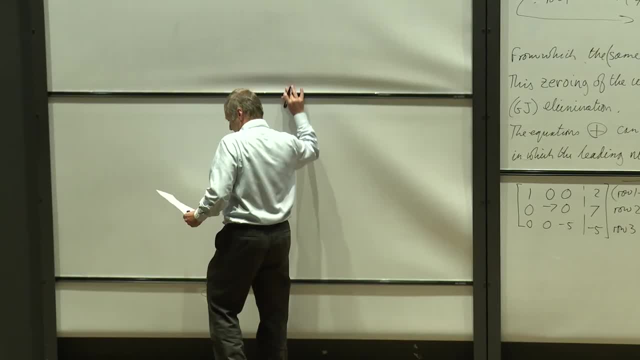 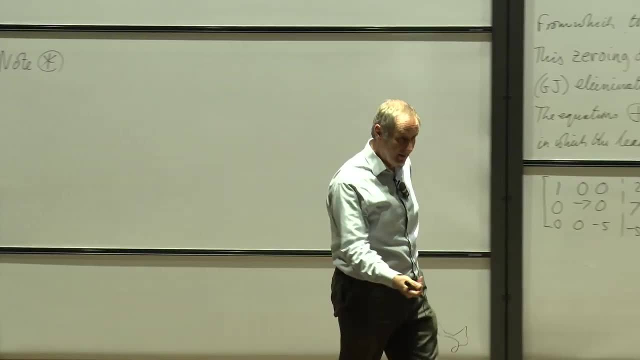 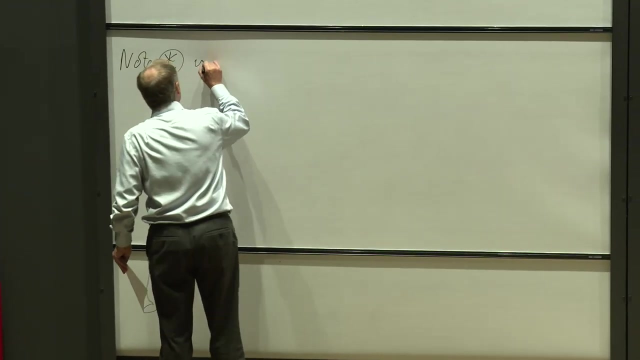 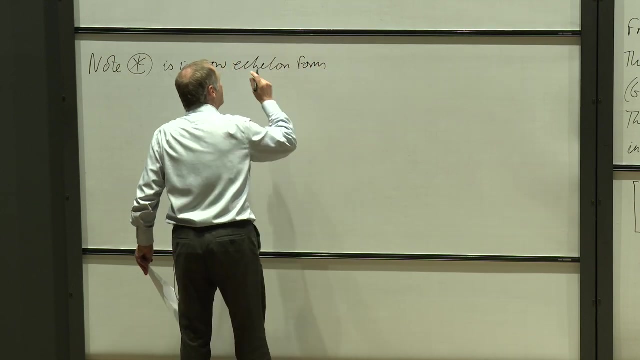 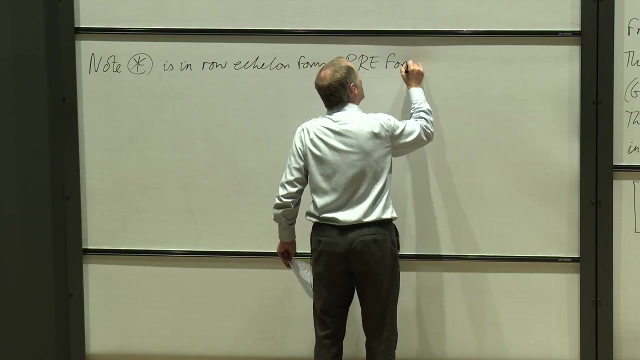 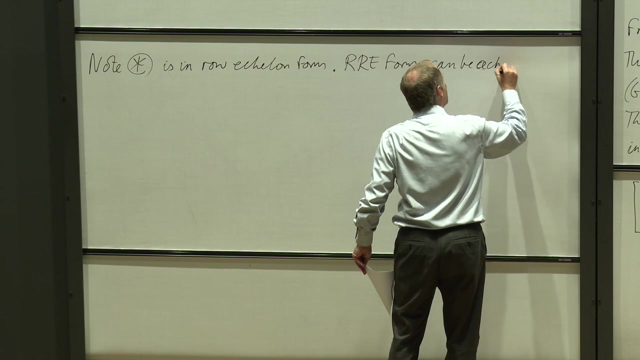 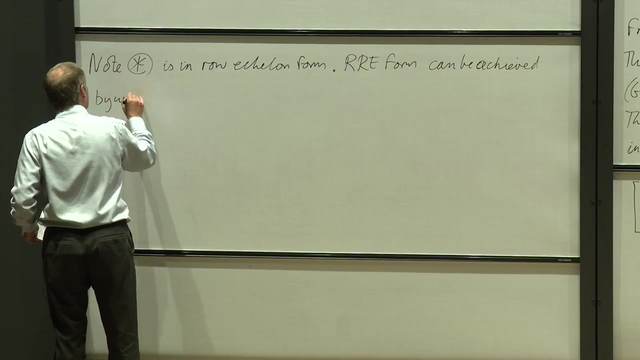 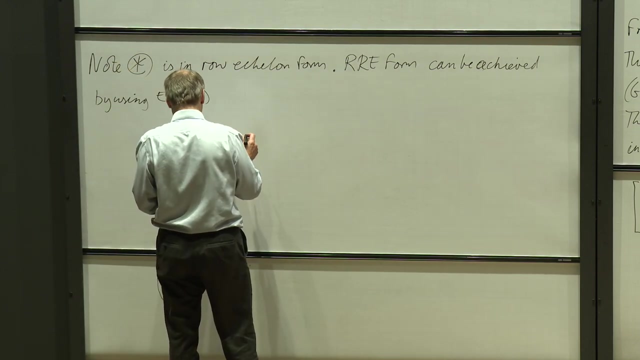 a little bit here. So note that that star. there's still only one star on the board and that's that equation over there. so that must be star, okay. so star is in row echelon form okay. reduced row echelon form okay can be achieved by using EROC to create a zero. 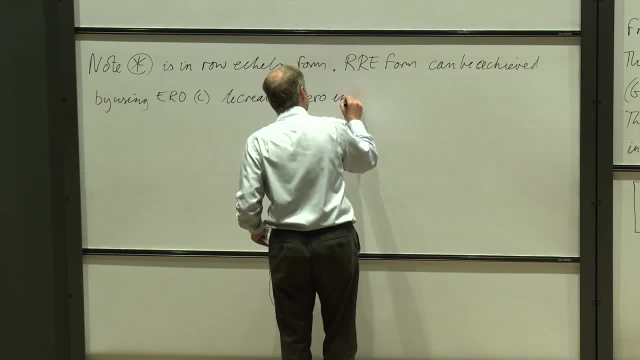 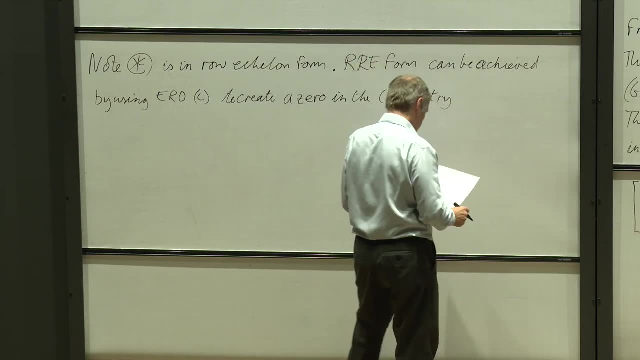 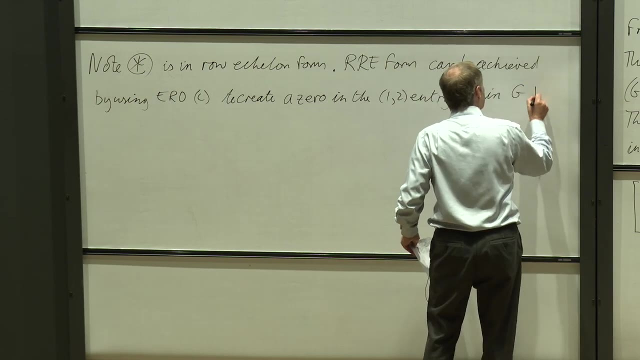 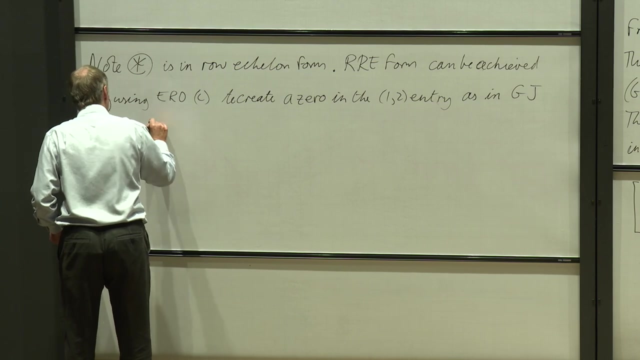 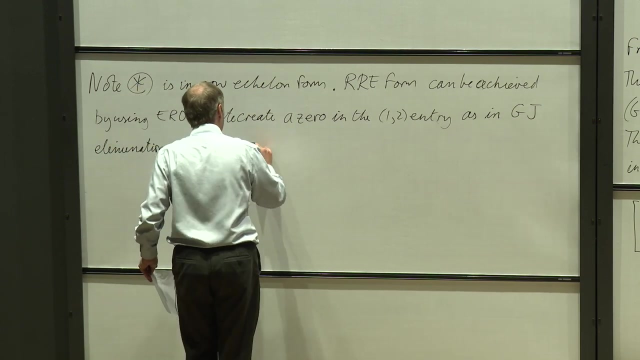 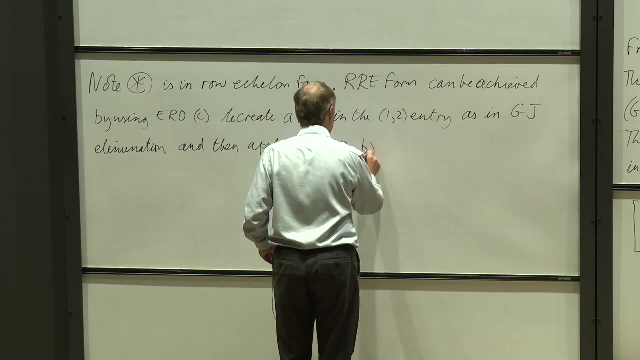 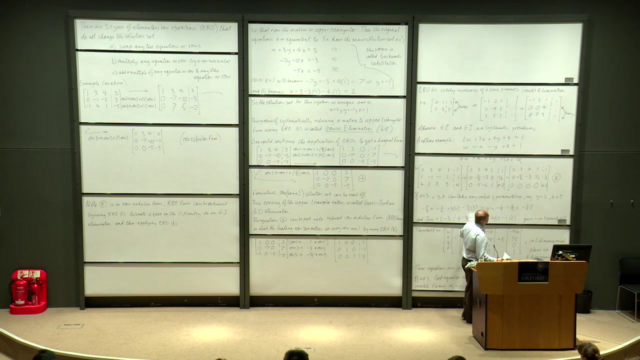 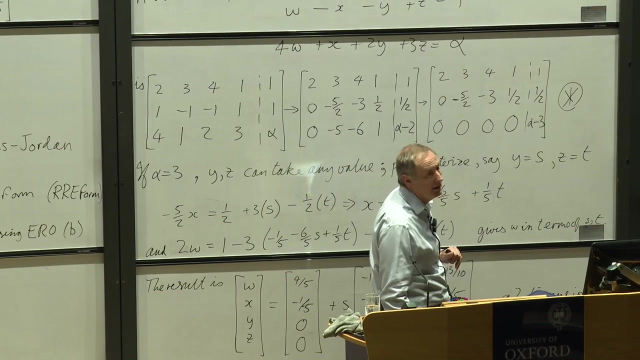 in the one-two entry, as in guess Jordan elimination okay, and then applying ERO B. that is just scaling equation. so all I'm saying is that if you take these equations star here, you can't really make the last row much simpler. but you can make this row a little simpler by taking some multiple of this but adding: 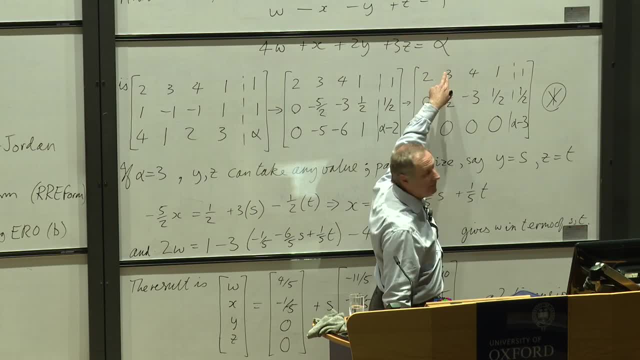 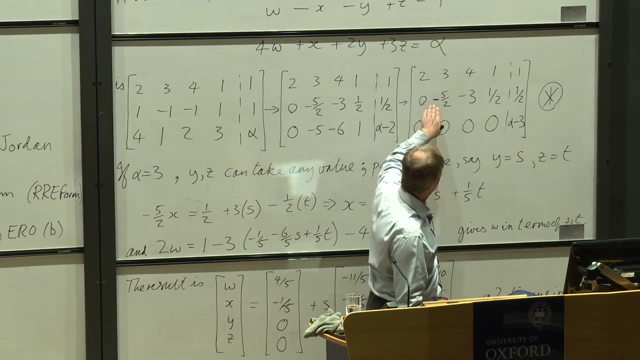 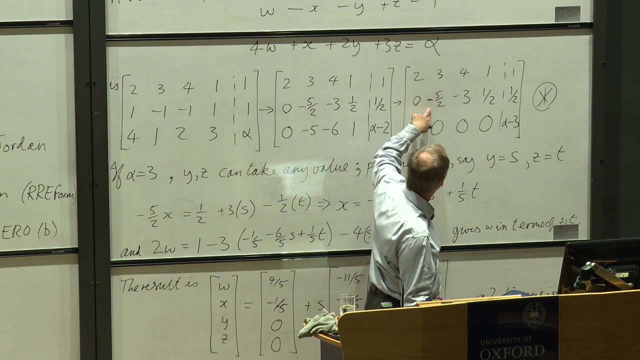 to this to make a zero. in this position, You can't create zeros here and here, right? So the only thing you can do is do one elementary row, operation C, to take what is it? Some multiple of this to add to this to make zero. 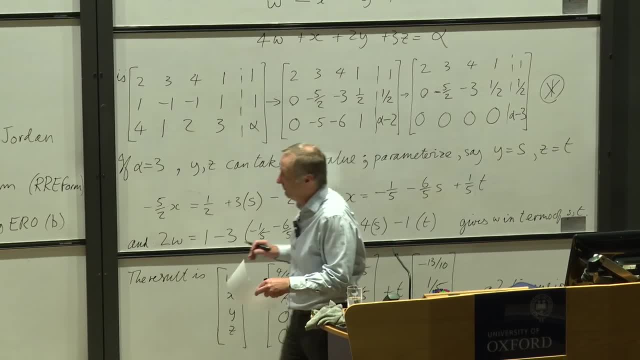 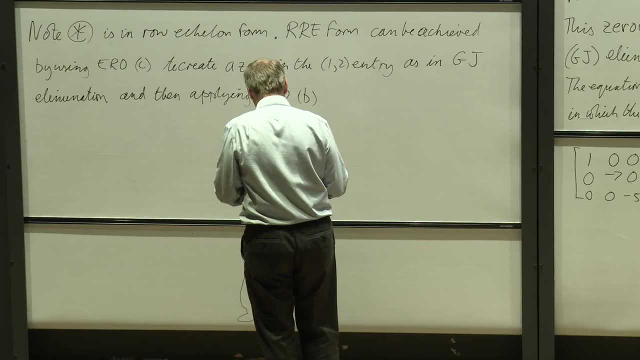 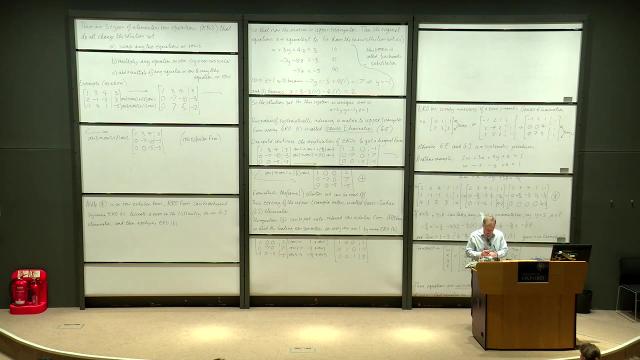 And then you get what's reduced to low echelon form. if you follow that up with scaling to make all the diagonal entries equal to, or all the sorry- all the leading entries equal to one. Okay, so I don't have time to say that, but I will, tomorrow at nine o'clock, be very precise. 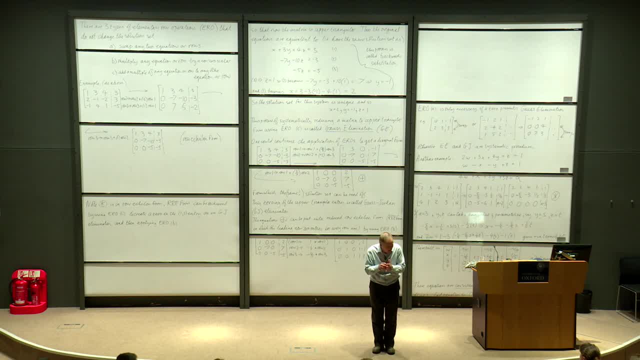 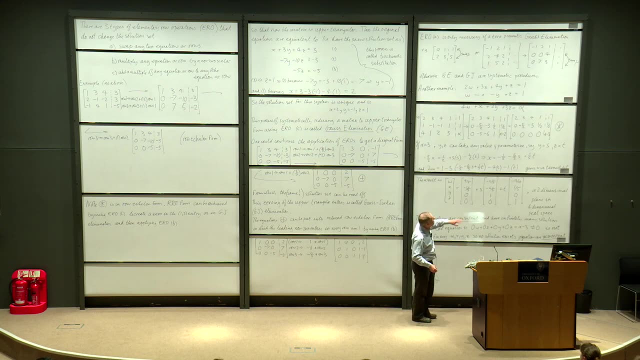 about what this reduced row echelon form is. I've sort of hinted at what it is, but I haven't quite stated it very clearly and you clearly in this example where you have here: Okay, If you have more variables, then you can't make it up a triangular. 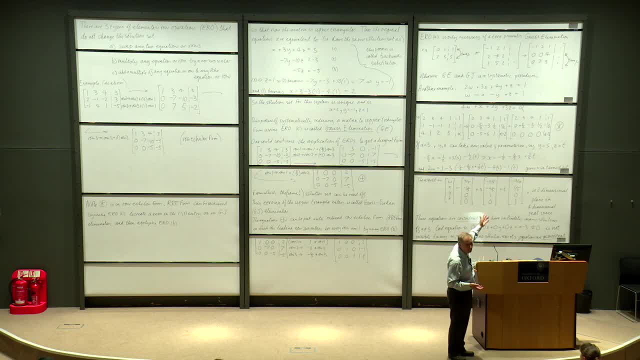 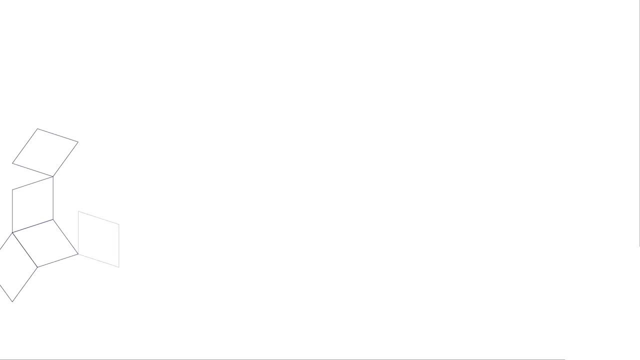